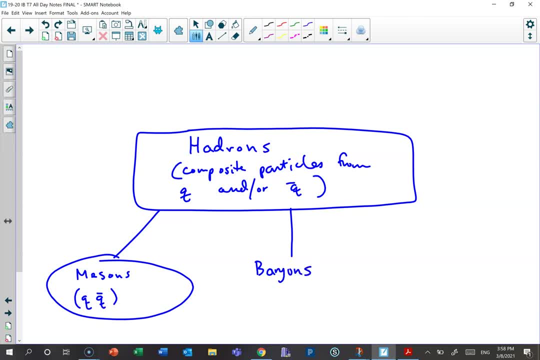 like the neutron and proton. those are baryons, It's three quarks. Or you can be a baryon if you are three anti-quarks. They do you know. there are suggested like tetra-quarks- I think that's what they're called- tetra-quark composite particles- and even like penta-quarks. 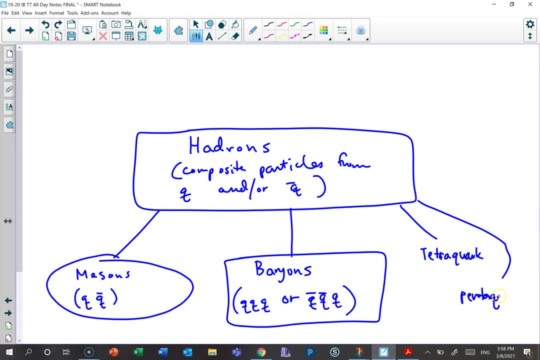 Did they see? they may have found a penta-quark for the first time recently, but I can't remember. I think they've produced penta-quarks in the lab for very, very short times, But these, like these, are not part of the IB physics curriculum and I think to some extent. 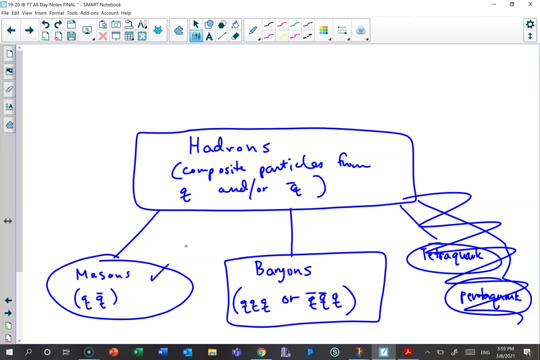 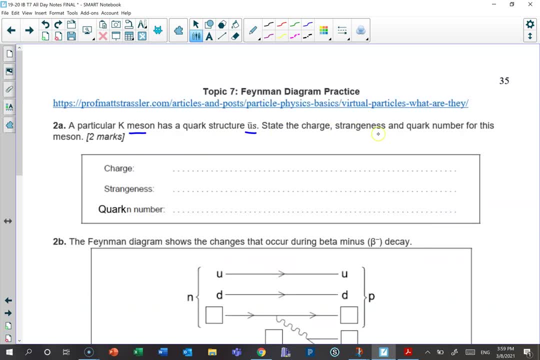 they're still sort of speculative physics. The two that we definitely know are there, that I definitely know are there, are mesons and baryons. Okay, state the electric charge, the strangeness and the quark number for this meson. 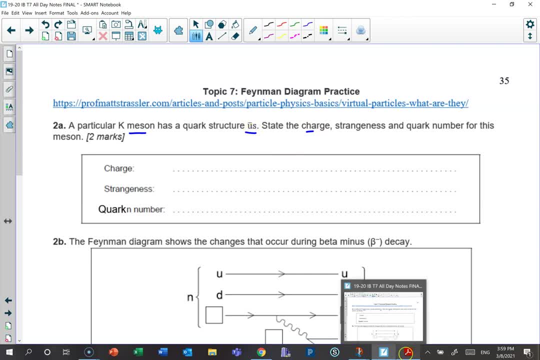 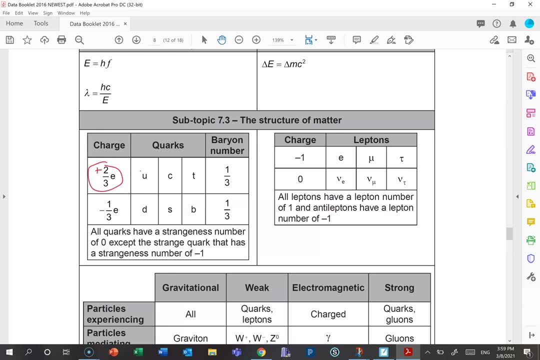 Let's start with charge Anti-up. and strange. Get your data booklet. Here's up, it's positive. two-thirds charge, Anti-up, it becomes negative. two-thirds charge, right. And then here's strange, it is negative, one-third charge. 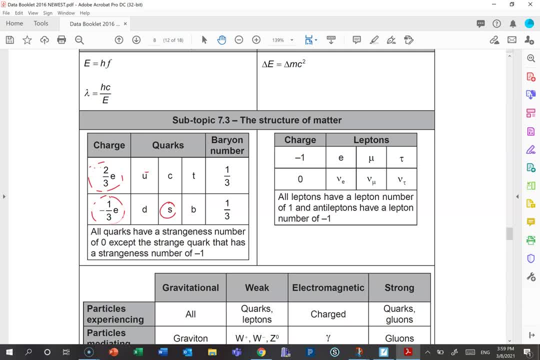 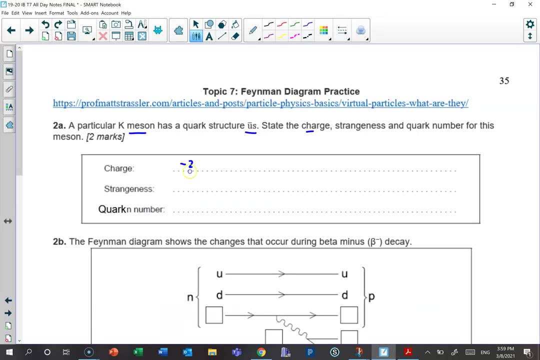 All right, let me clear off my data booklet. And when you add those all together- negative two-thirds plus negative one-third, the total charge is negative one times the elementary charge. E- Negative two-thirds: Two-thirds of the elementary charge plus negative one-third of the elementary charge is negative. 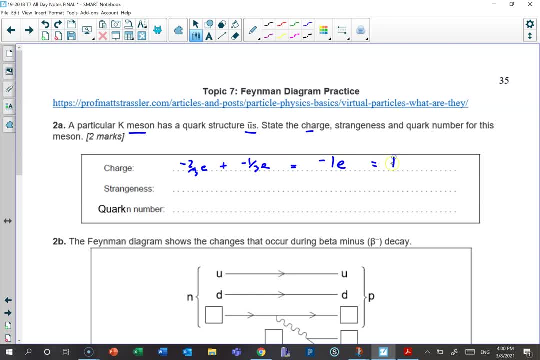 one of the elementary charge. So you could also say: if you wanted to be really fancy, but we don't really worry about this- you could say: it's equal to negative 1.6 times 10, to the minus 19 coulombs. 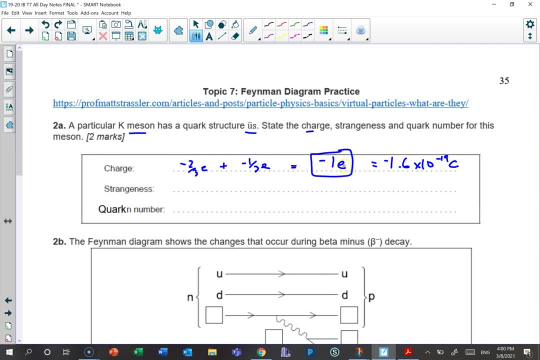 But it's fine, they expect you to leave your answer like in terms of elementary charge. Strangeness, Remember, let's do quark number first. Let's do quark number. You're counting how many quarks and anticoagulants. 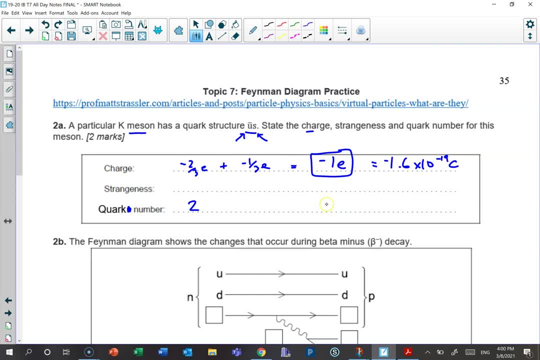 Okay, How many quarks and anticoagulants are there? Careful, the answer is not two, because the anticoagulant, you recall, is counting as negative one. when we tally our quarks And the regular- strange the matter- that's positive one, and so the total is zero. 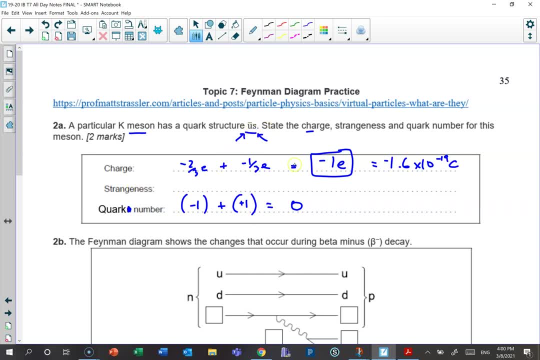 Now, strangeness is literally the same thing. Count how many strange particles are there? Something like this would have a strangeness of three. something like this would have a strangeness of negative three. except because it's so strange, we flip it. 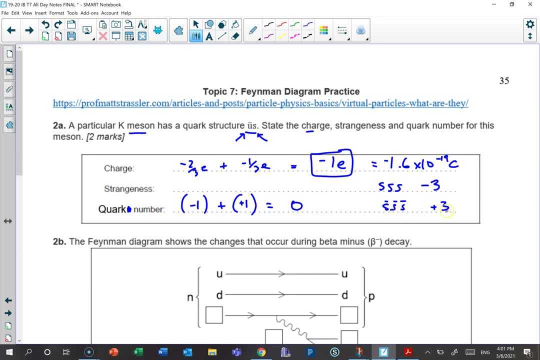 Regular matter counts as negative and anti-strange counts as positive when you're tallying your strange value. So the total strangeness here is you would think it's positive one because it's matter, but you flip it for strange. That's weird, I know. 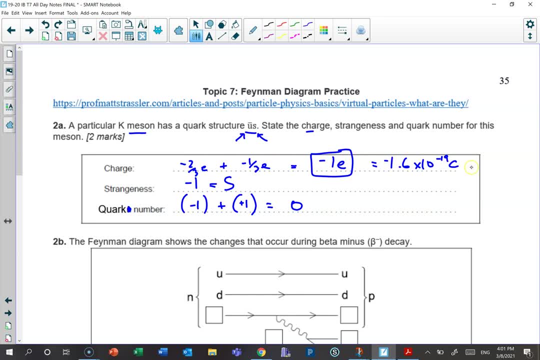 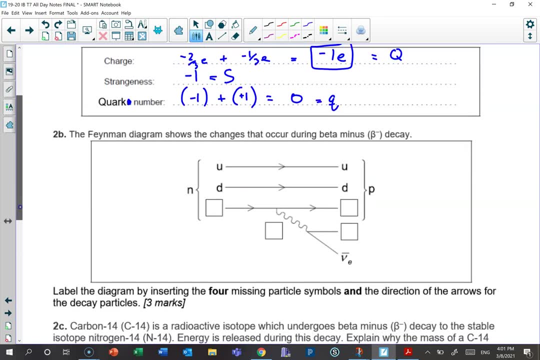 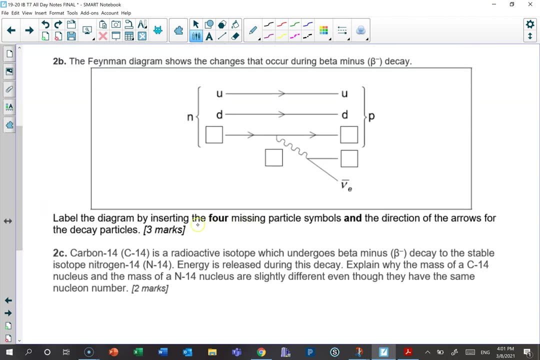 Okay, So that's capital S strangeness. Okay, So this is capital Q charge, electric charge, And I use little q for quark number. Okay, Here's the Feynman diagram for beta minus decay. Label the diagram by inserting the four missing particle symbols: one, two, three, four and 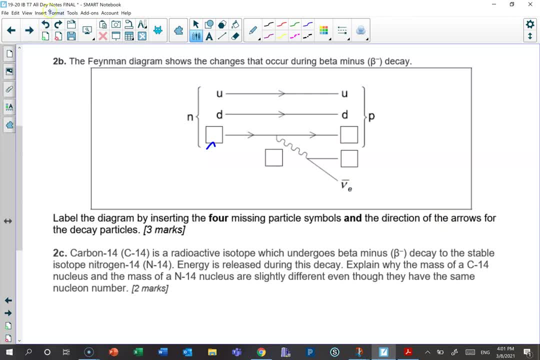 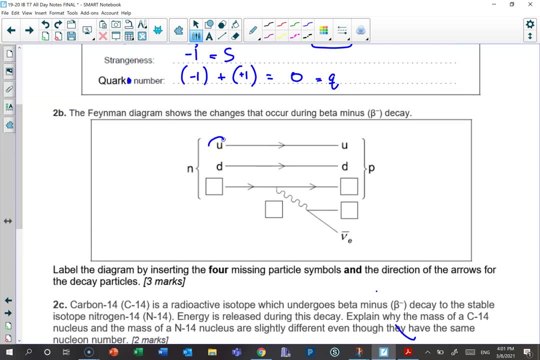 the directions of the arrows for the decay particles. Well, don't you need to know where the time axis points? Hang on, we do. The up quark is matter, And so its arrow must be, with the time axis, like this: 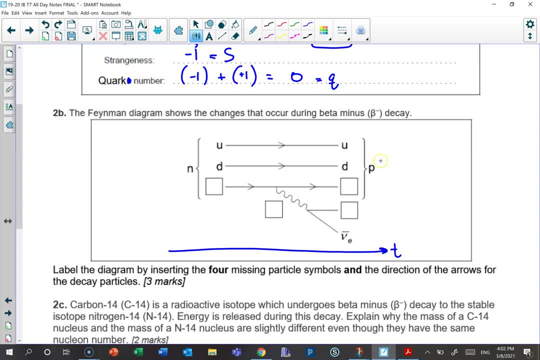 So now we've deduced where time is pointing. Okay, first, you know, when you have beta minus decay, the first thing you immediately know is that we produce a beta minus particle, And you know that that has to pair. Okay, The electron has to be paired with the electron neutrino, because together they're total, like. 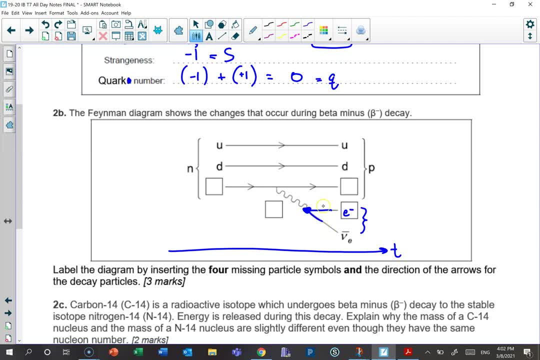 if you look at this intersection here and here, the total lepton number is zero. afterwards And coming in, you only have an exchange particle entering that vertex. So the lepton number is still zero initially And so that's the only you need the electron to be here. 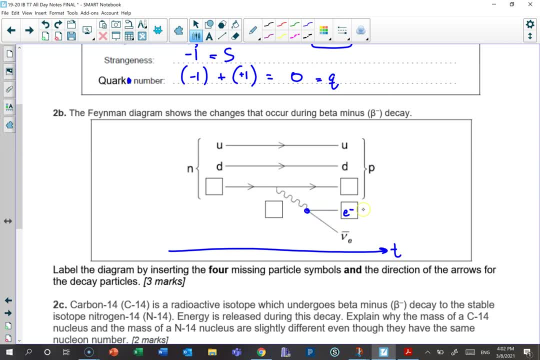 Okay, What else do we know? This is matter. so its arrow is with time. That's antimatter, so its arrow is against time. We know proton: It's not a proton, it's a proton bruh. Two ups and a down. up, up down. 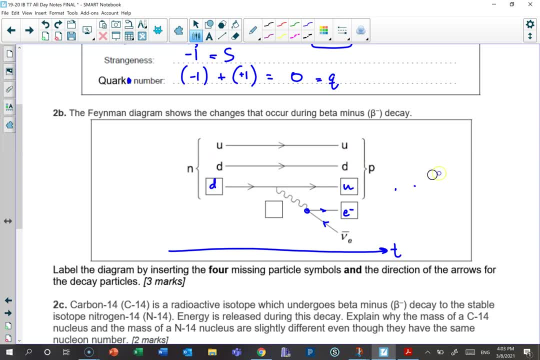 And the neutron is the opposite. two downs and an up. Finally, you can figure out what this exchange particle is. Sometimes the exchange particles are drawn with these lines, the squigglies. Sometimes they're like this: That usually means it's a gluon. 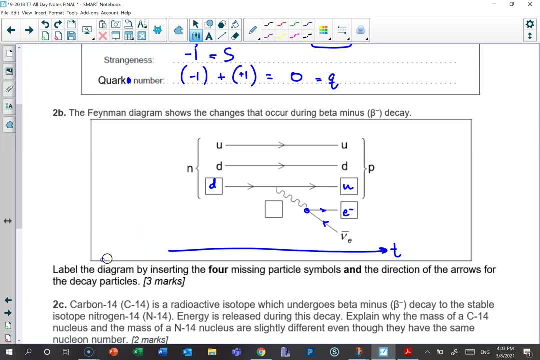 Sometimes it's like this, But you'll see different things happening. Well, okay, Continue to look at this vertex. The total charge exiting is negative one for the electron and zero for the neutrino. Add them up and the total charge exiting the vertex is negative one. 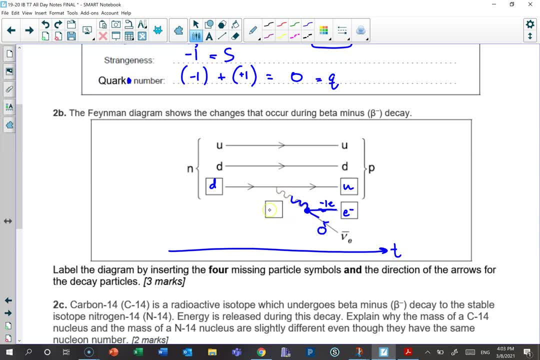 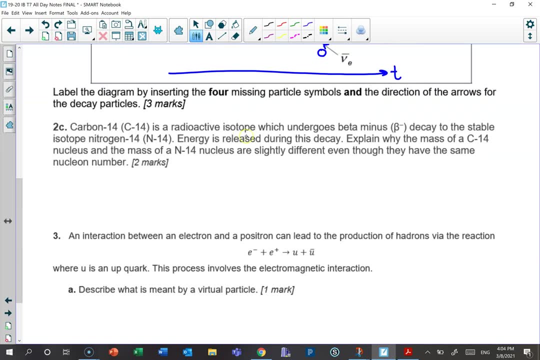 So what's the total charge entering the vertex? It's negative one. This must be a negative minus boson To see. carbon-14 is a radioactive isotope which undergoes beta minus decay to a stable isotope, nitrogen-14.. 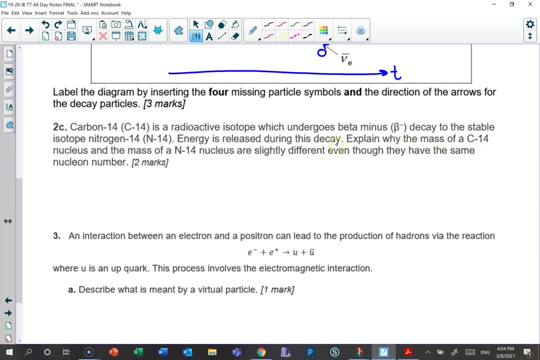 Energy is released, Explain why the mass? ooh, yes, I'm going to let you think about this one. Yeah, I'm going to let you think about that. Carbon is negative. Carbon is zero. It's negative minus six. 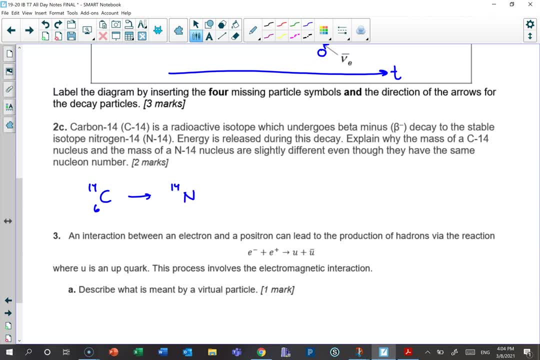 Here's the idea. You can even write this out if you wanted. Like this, What they're saying is: hang on. if you add the total nucleon number, the total mass number, at the end and you compare to the beginning, It sure looks like mass is negative one. 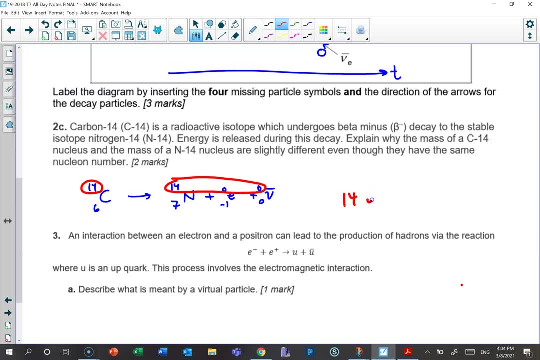 That's a negative, negative, negative. It's negative 1, negative 1.. That's negative, 1.. is conserved, But that's not right. The mass initial would be something like- I'm just gonna make up values: 13.997.. I know that this is wrong And then that 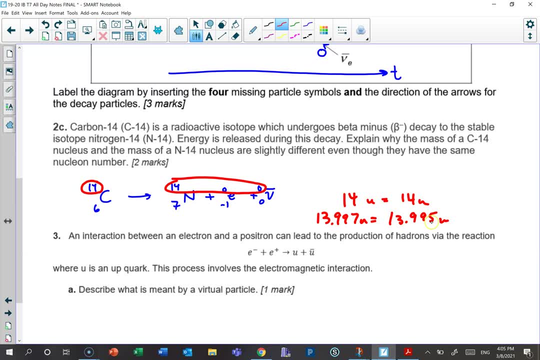 mass final might be like 13.995.. So when we write 14 up here at the top and over here too, we're rounding, And if you look at these extra digits they're not the same. Why is that? As a hint, think about Einstein's right, You've got some. 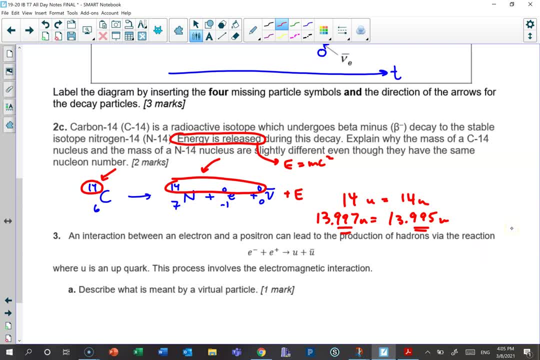 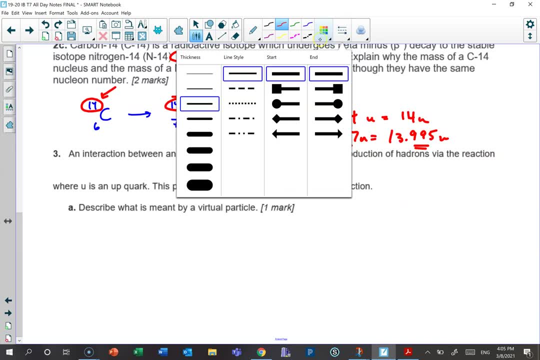 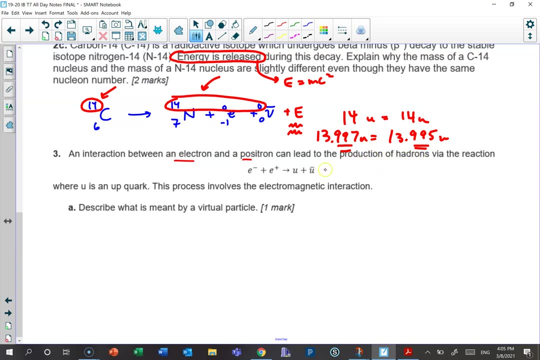 energy at the end that did not exist initially. Where are you getting that energy from? Okay, let's move on. Okay, an interaction between electron and positron can lead to production of hadron. It involves the electromagnetic interaction That means photon. Describe. 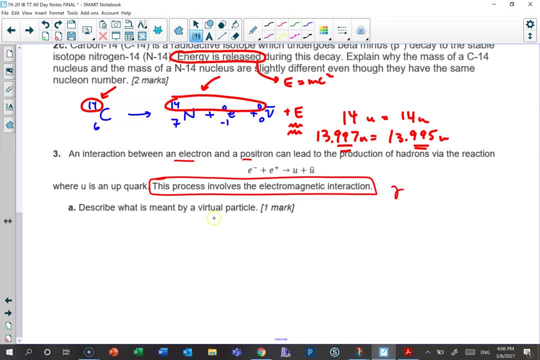 what is meant by a virtual particle? Hmm, a particle that attends hybrid school or NTI school, right? No, no, just a little, just a little pandemic joke for you. A virtual particle is a. what do you put here? It's an exchange particle That mediates, I think. what? 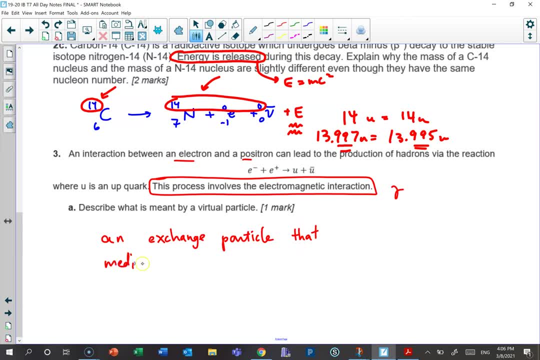 IB wants you to say is mediates one of the four fundamental interactions. That's a position, And it can have a negative or negative reaction. Yep, there it is. I mean, a really cool definition is a quantum, an alternate definition? 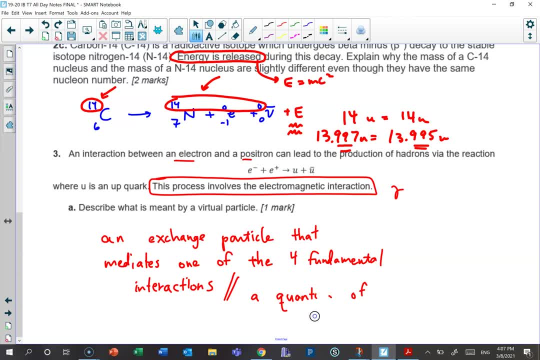 maybe if you want to blow their socks off. I don't know, They may not. if their socks are blown off too much, the examiner they may not give you the point because they may not understand what you're saying. But another definition is a. 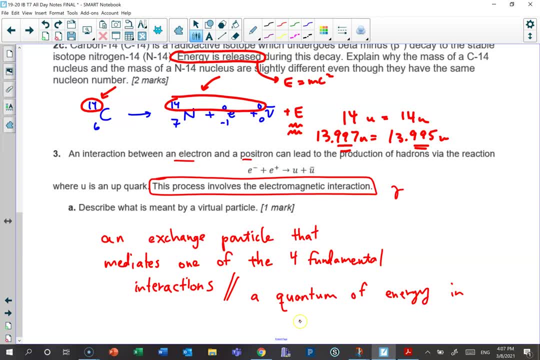 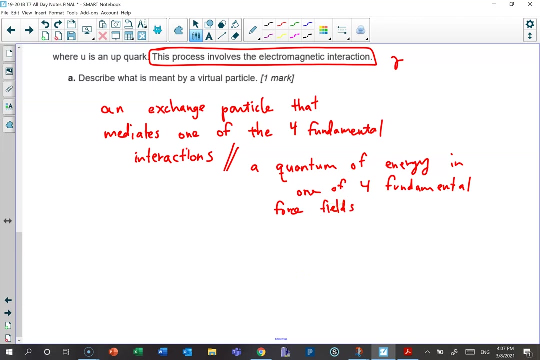 quantum of energy. the four fundamental interactions will fundamental one of the four fundamental force fields- this is a better definition- which is non-real. it's not a real particle. it doesn't obey which is not real. it doesn't obey the laws of physics but is used to model the 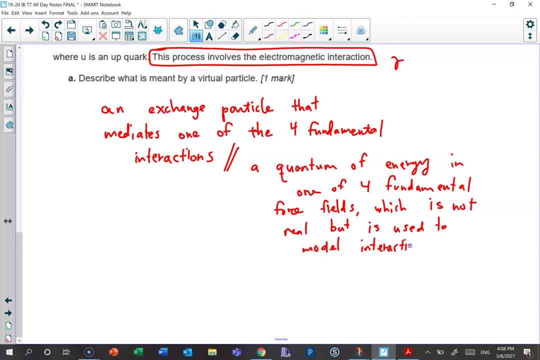 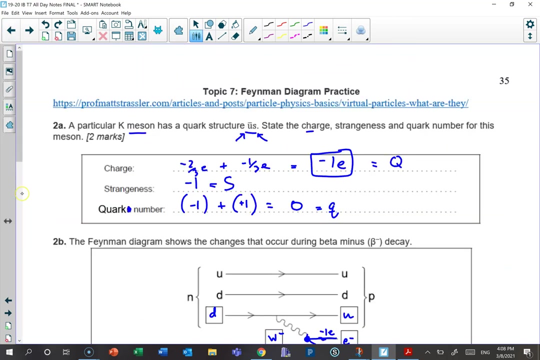 interactions between real particles. that's like your college physics professor next year will be impressed if you say that. okay, but this is what IP is looking for. this first one is what they want: hadrons draw a Feynman diagram. okay. what was it all the way back? okay, got it. 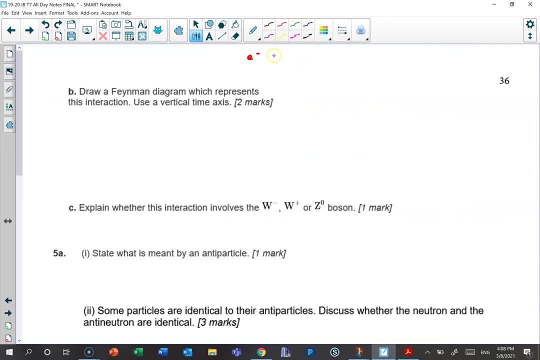 draw a Feynman diagram. it was this right? let's hope so, because that's what I'm solving. use a vertical time axis. alrighty, I know how to do that. I draw my arrow here: time, and we start with electron, which is matter. always label your Feynman diagram, and you know. 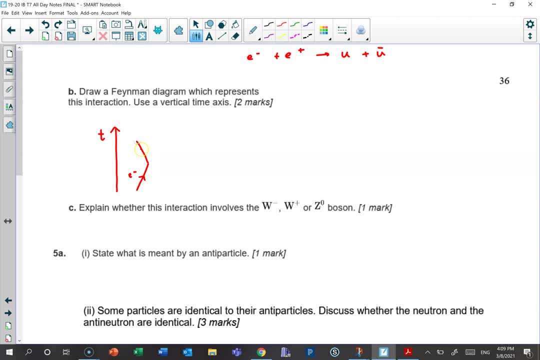 what I'm gonna try. I'm just gonna try something like this. let me try something like this. I'm just gonna try something like this: let me make, make something up that's gonna be wrong and I need something else initial, so I'll make this. the anti- whoops- that's not, that's not initially- is this: and: 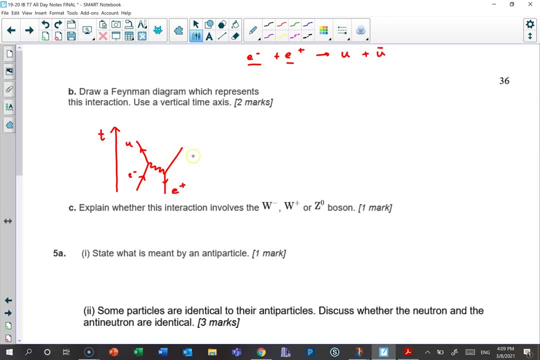 this. so that would have to be the end. the anti electron, the positron, and here is the anti up. now you can probably see why this is wrong. right, because if you consider this interaction, that vertex, for example, the lepton number going into the vertex is negative one because it's an anti lepton and the 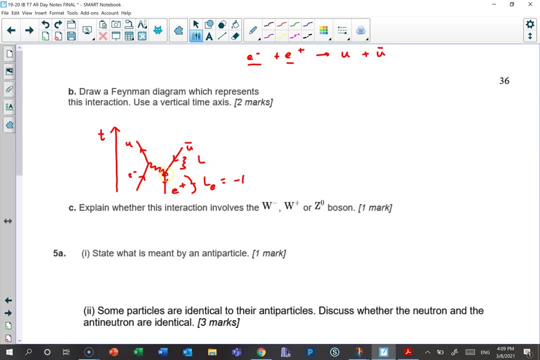 lepton after the vertex. you've got the exchange particle exiting the vertex and you got anti up zero. so that doesn't work. let me try again. how about, instead of having the electron and the anti electron, instead of having them exchange something, let's have them come together? 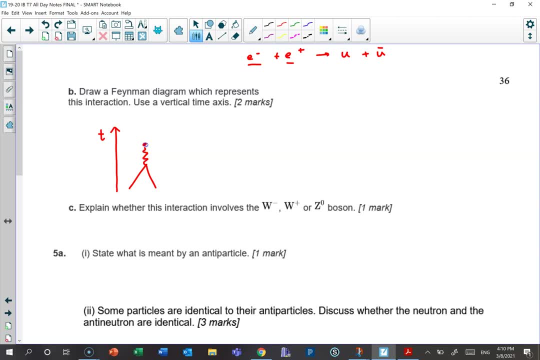 and on the other side we have that. that's it. this one works. I know that these are on the initial side, so earlier in time, remember, look at your time axis- these have to be initial and at the end you have up and anti up. and what is this exchange particle? it's a photon, because they said that the 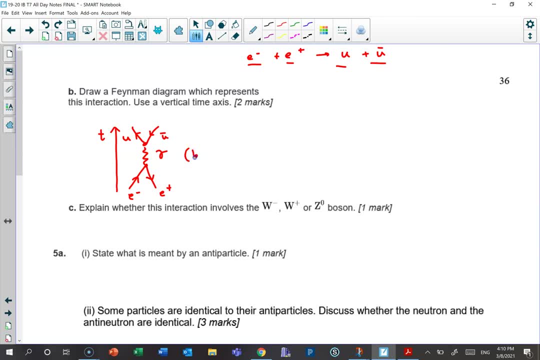 interaction is electromagnetic. that's how you know explain whether the interaction involves: ooh, none. if the prompt you said it involves the weak nuclear force instead of electromagnetic, then the answer would be what? well, look at the total charge entering this vertex. here you've got negative 1 and positive 1, and so the total charge entering comes to. 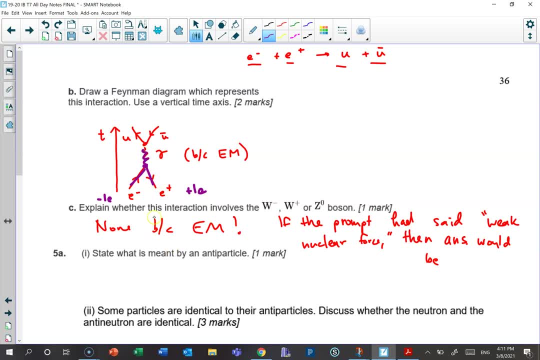 zero. therefore, at the end, the total charge would also have to be zero. if it were a weak interaction, then the answer here would be the W, I'm sorry, the Z boson, because the Z boson is neutral Stan state. what's meant by an antiparticle? 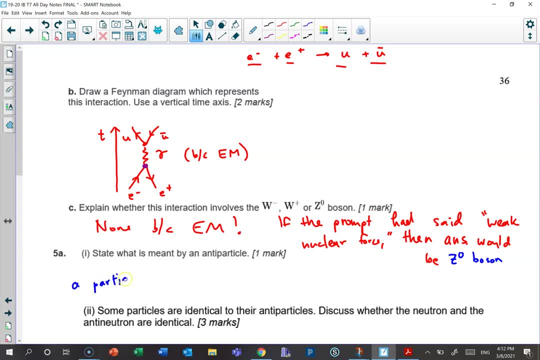 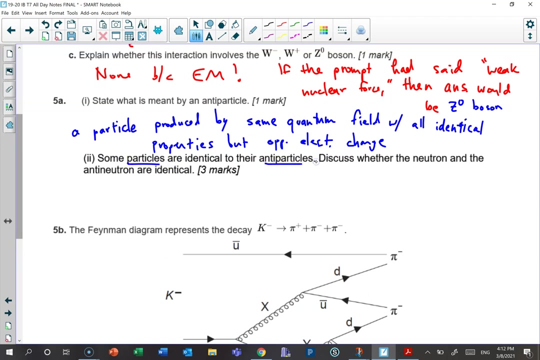 it is a particle produced by the same quantum field with all the same, with all the identical properties. that's the word. same properties, but opposite electric charge, and I'm abbreviating here. but that's the idea. some particles are identical to their antiparticles. how about the neutron? oh, 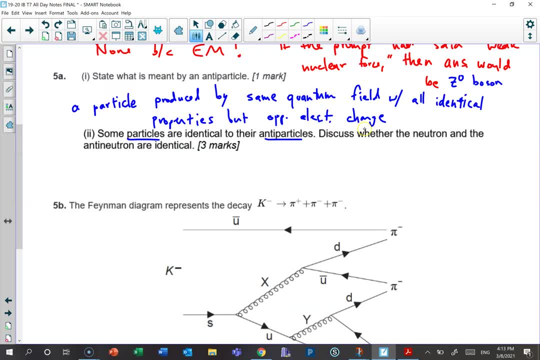 this is tricky. this is tricky. what is a neutron? a neutron is not an up-up-down, that's a proton bra. the neutron is the up-down-down. now you might be inclined to say this, which is wrong. maybe you think: oh, the neutron is neutral, right, it's got no charge. so the anti-neutron is also zero. 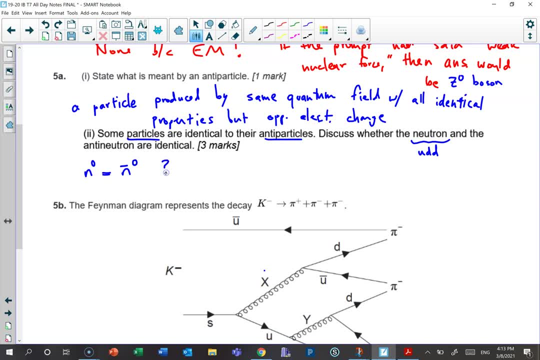 charge. so maybe they're identical? question mark: no, because think about what they're made of. they are not the same. while the neutron and anti-neutron has the same electric charge, when both are zero charge, the neutron- and you would say this in words- is made up of: 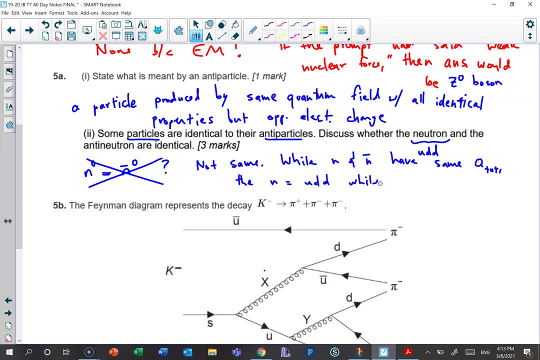 up-down-down, while the anti-neutron would be întrotron. choice is where the to make or count opposite current amounts to a force equal to zero. charge teachers in Camp P. ok, my right to double is to roll up to b and to 거� relating to B, as in where to 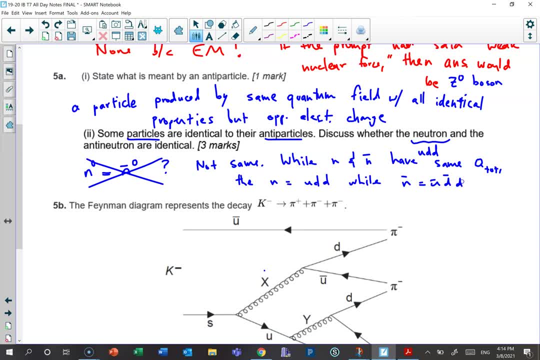 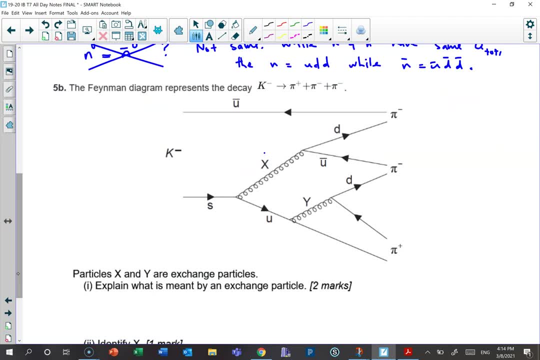 voz: Anti-up, anti-down and anti-down. There are two ways to get to zero. These are not the same. The Feynman diagram represents the decay shown there. Now, going into this video, my hope is that you remember that the positive pion is: 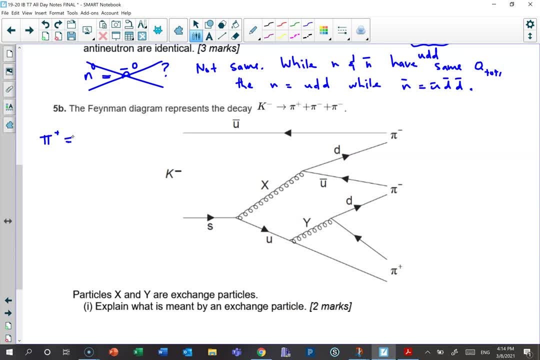 this doesn't matter for the problem, but my hope is that you would recall the positive pion. oh, they kinda showed, don't they Look? the positive pion is those two things together. That's anti-up and down. That's not right. that's the negative pion. 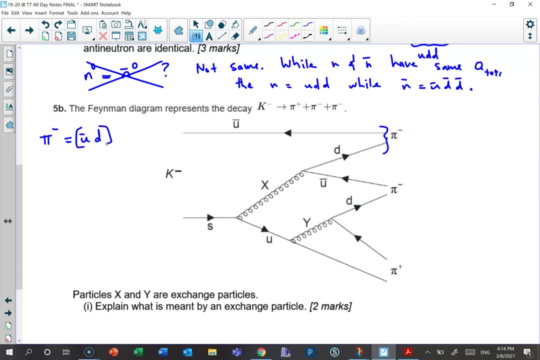 I'm not reading the diagram? Yeah, because those add to a total charge of negative one. Here's another negative pion, another anti-up and down collected together as an anti-pion, sorry, as a negative pion, pardon me. 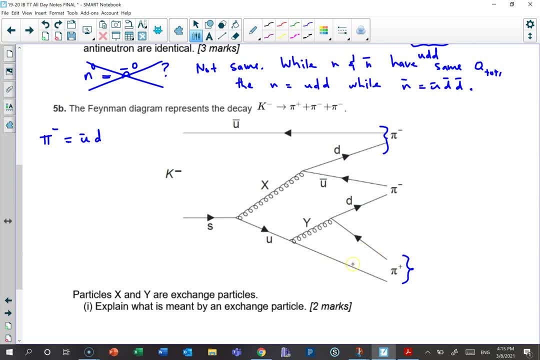 And then here's a positive pion, And so the positive pion. yes, they did not tell you, but you can figure it out. It's a combination of up and down. One is anti-matter, the other is matter. 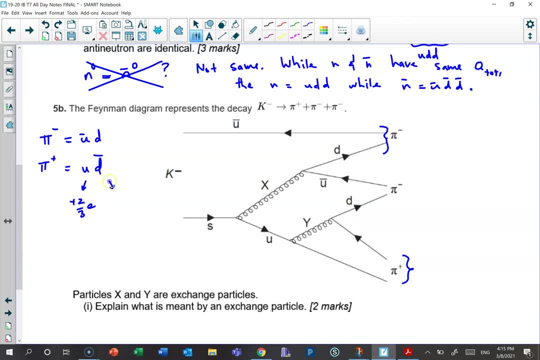 Just look at the charge. This is positive, 2, 3rds. your data booklet says Anti-down. normally down is negative. 1, 3rd. Anti-down is opposite and they add to positive one. So you already know part of what the answer's gonna be here. 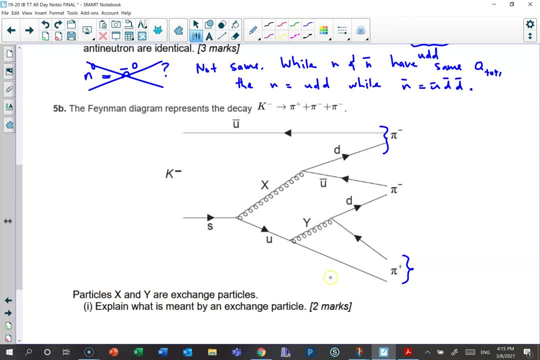 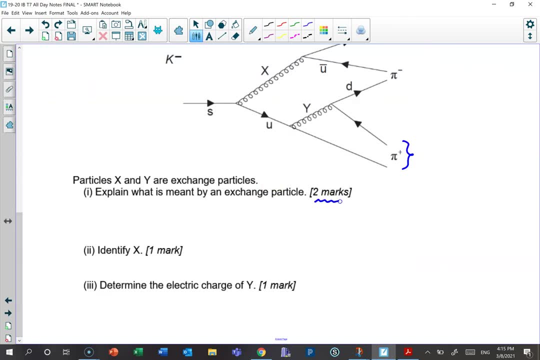 Okay, particles X and Y are exchange particles. All right, explain what's meant by an exchange particle Here. this is what IB wants to say: two marks. It is a virtual particle that mediates or carries one of the four fundamental interactions. 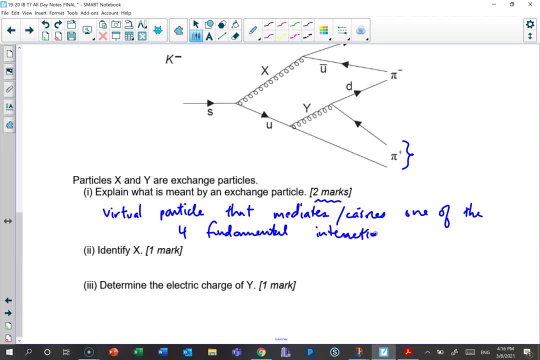 So it's like the force of nature, And by interactions we mean like the force, one of the four fundamental forces. The reason we don't say force but we use this new term, interaction, the reason for that is that forces could be like. 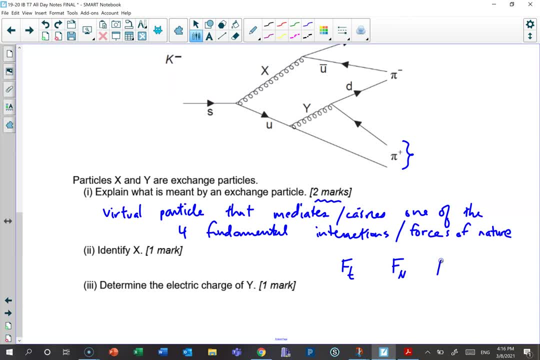 force of tension, normal force, force of friction. We're not talking about those when we talk about the four fundamental forces. so, to clarify, we use the term interaction. We like to use the term interactions for the strong nuclear force, the weak nuclear force. 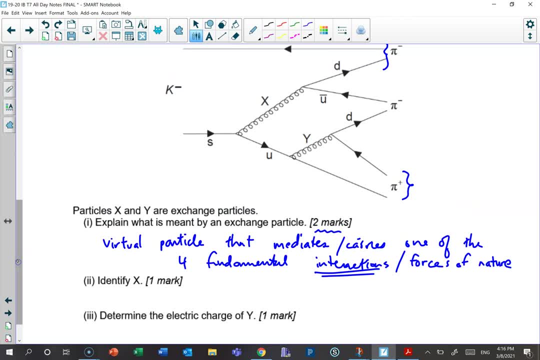 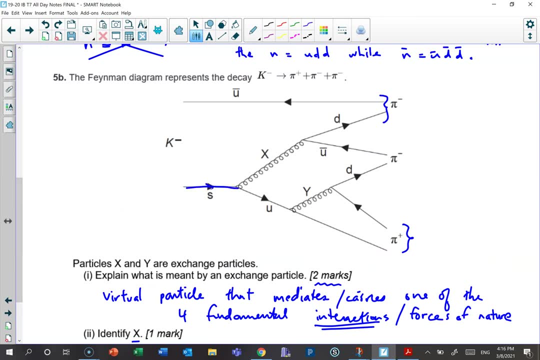 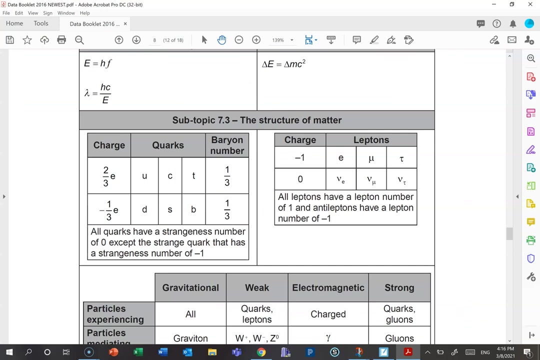 gravity, the electromagnetic force. Okay, identify X. Yes, as soon as I see this. and then this like strange goes: oh, pardon me, pardon me, As soon as I see this right here, strange changing to up. You may be inclined to check strange and up. 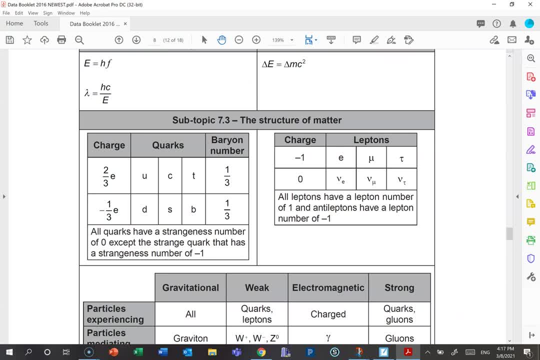 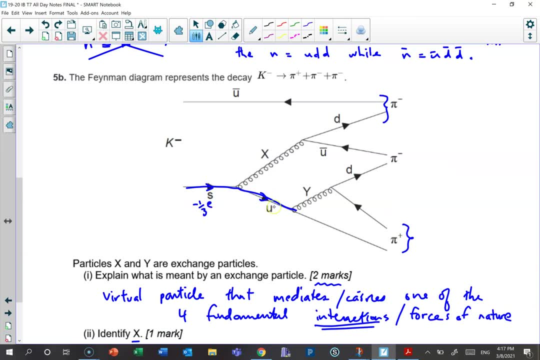 Okay, and you'll realize they have different electric charge, And that's enough, right there. negative 1, 3rd, and negative 2, 3rds, Positive 2, 3rds, rather. That's enough to figure out what this thing is. 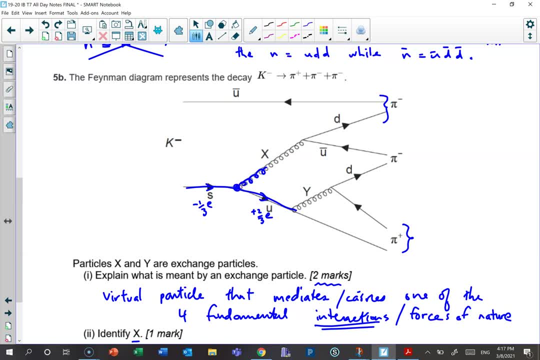 But there's another hint: There's a general rule that the strangeness, the total value of strangeness, going into a vertex is equal to the total value of strangeness exiting the vertex, unless you are dealing with the weak force, unless it's a weak interaction. 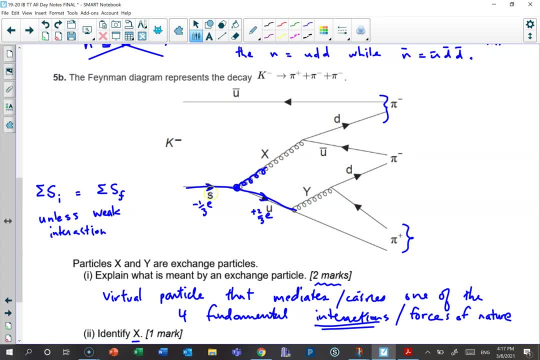 And so immediately, because we have a total strangeness here, initially of negative one and a total strangeness at the end, here and here of not negative one, that's zero. there are no strange quarks exiting this vertex Because of that, we know we're dealing with. 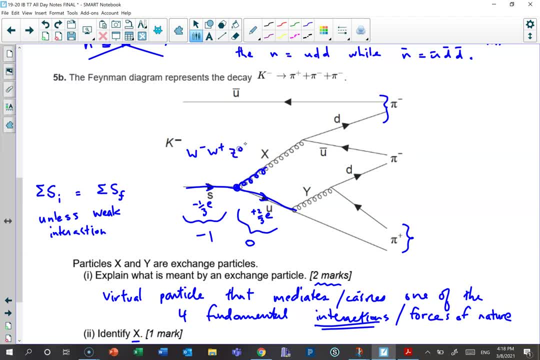 x is either gonna be w minus, w plus or z zero. And then to get to the final answer between those three, you look at the charge, The total. if you consider the total, time has to be pointing this way, because anti-up would have to be pointing against time. 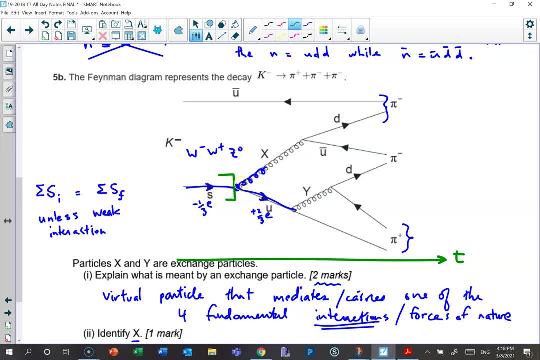 So okay, the total charge entering that vertex is negative one, sorry, negative one-third, which means the total charge at the end has to also be negative one-third, which requires x to have a charge of negative one, Because when you add these, 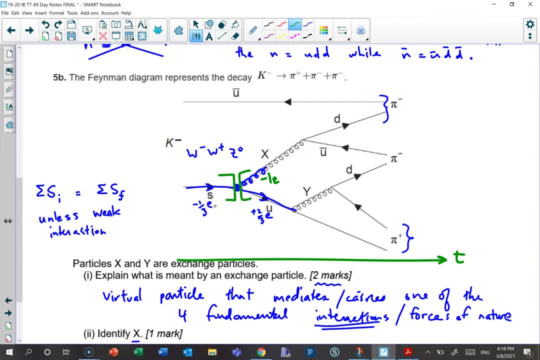 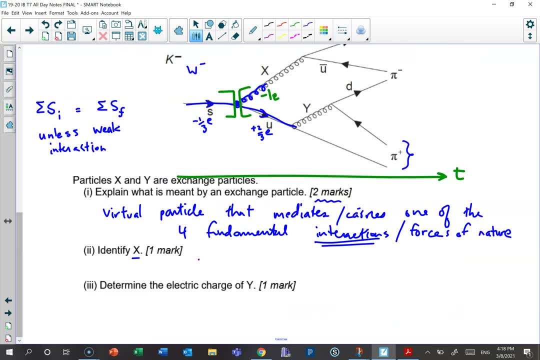 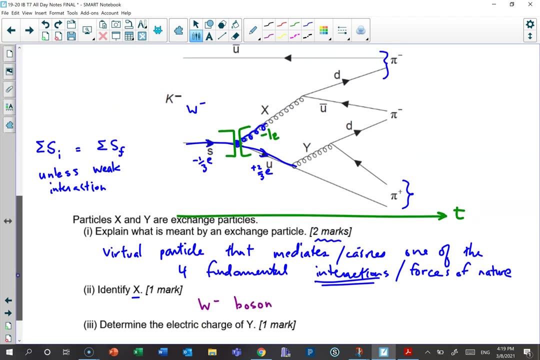 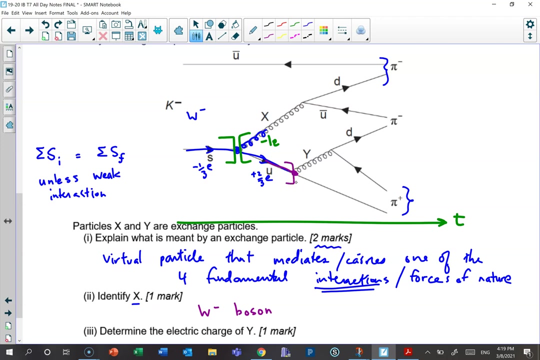 now you get the correct total negative one-third. So this is a w minus boson. So you can take the w minus and then you can sum that in place with positive one-third. Determine the electric charge of y. Okay, I've got the up quark coming in. 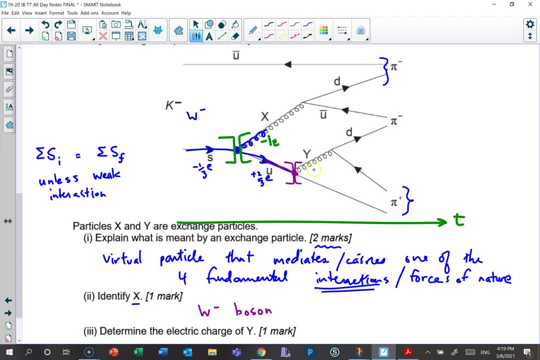 with positive two-thirds. So the total charge entering this vertex is positive two-thirds. That means the total between the two exiting should also be positive two-thirds. Oh-ho-ho, What a problem. Look at this. The pion is nothing more than an up and anti-down. 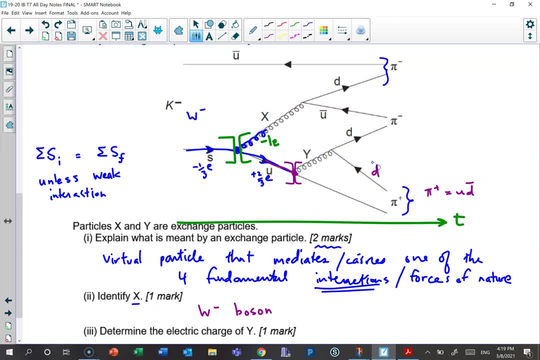 Why is that important? Because this here must be anti-down. That means this is up. So if you balance, you've got positive two-thirds electric charge coming in, and then you've already got your whole positive two-thirds right there. So the charge has to be zero for this exchange particle. 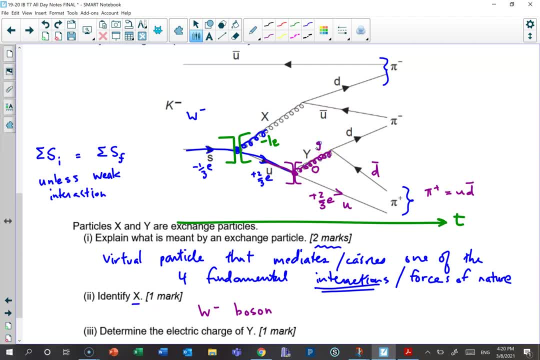 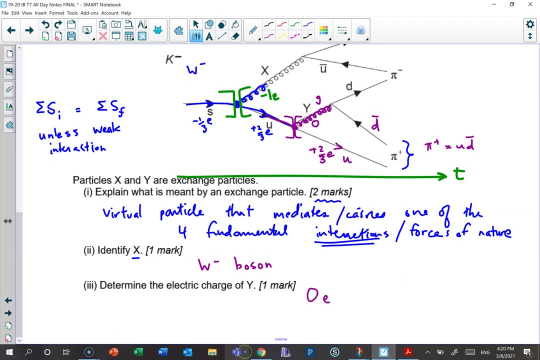 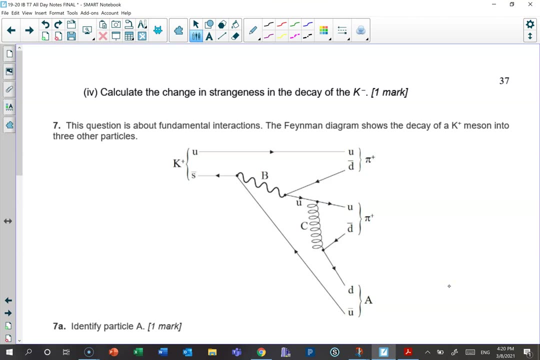 When they draw the squiggly like this, that's usually a gluon, That's usually the strong force Zero of the fundamental charge, the elementary charge. Calculate the change in strangeness in the decay of the k-. Let's go back. 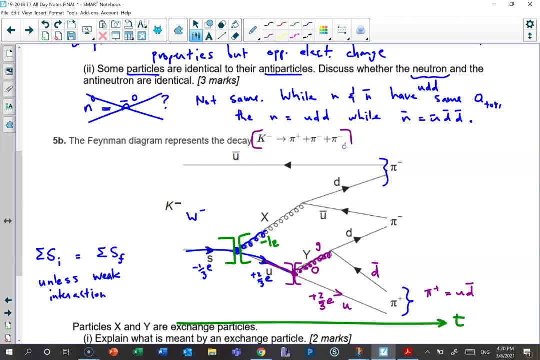 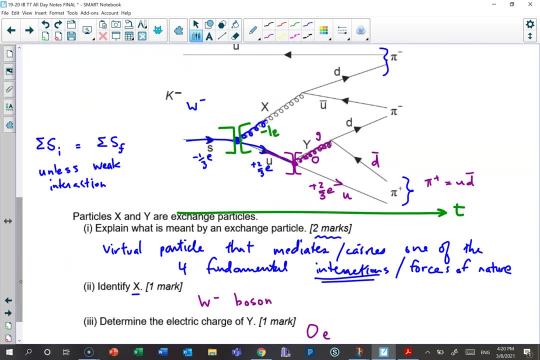 So when they say the decay of the k- they're really talking about from the very initial moment to the very final moment. And so from the very initial moment- jeez, I've got so much stuff here like from over here- initial, initial, initial. 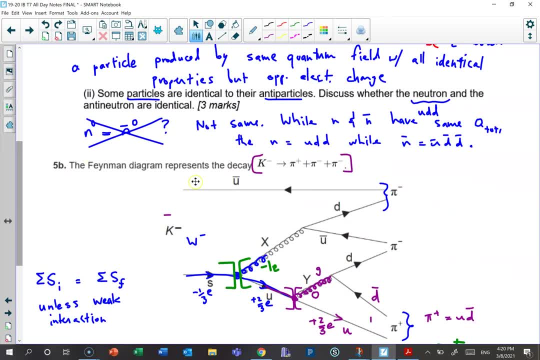 the k- particle is the up. It's this combined with this, And so the strangeness there. initially, if you add up, you only have one strange quark. It's matter, It should be positive, but for strangeness when you're counting strangeness. 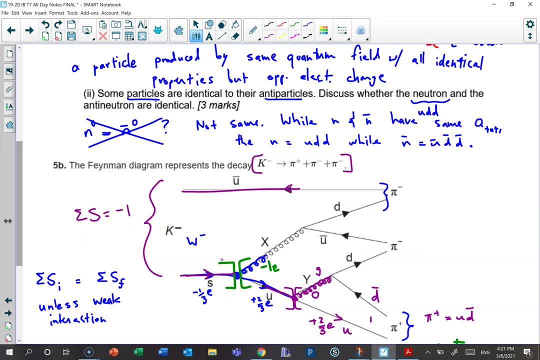 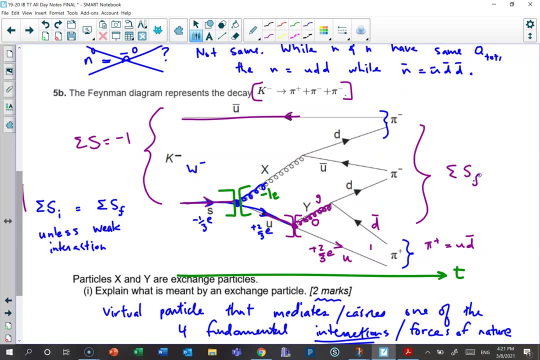 we make it negative, And so that's negative one initially, And if you look at the end, no more strange quarks Zero. All right, that's an up at the end, at the very very end. Forget all the intermediate stuff. 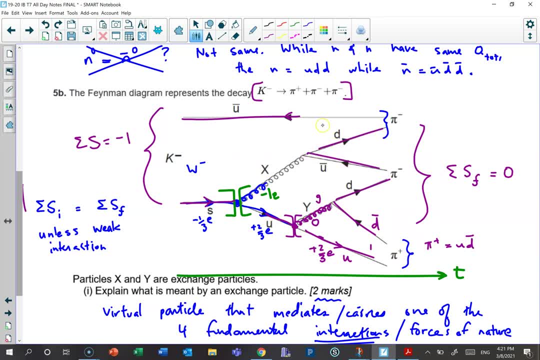 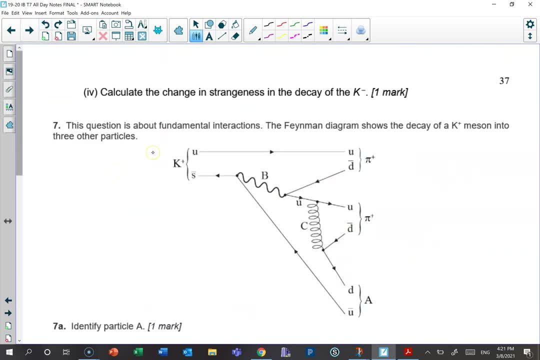 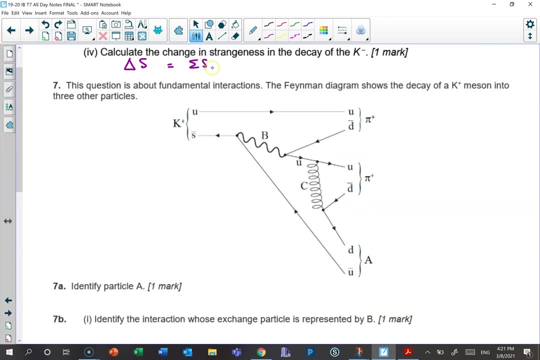 We've got an up, a down, a down, anti-up, down and anti-up. So no strange. So what would you say? The change in strangeness equals the total strangeness. final minus initial. right Change is always final minus initial. 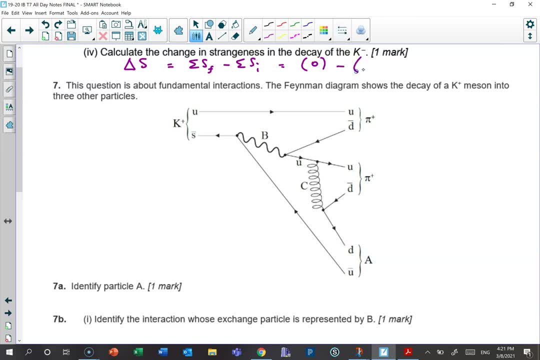 There's zero at the end. You can see where this is going. It had to increase one because you started at negative one. You ended That's zero Seven. So here we've got the decay of a K-positive, K-plus meson into three other particles. 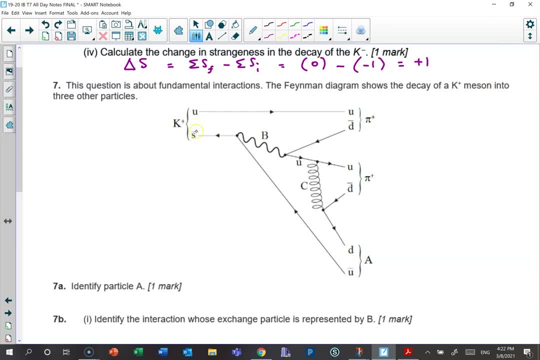 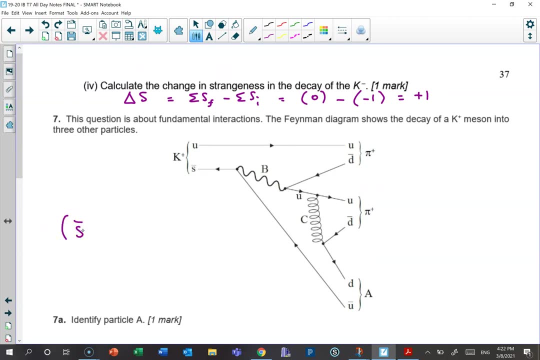 Meson should only be two: a quark and an anti-quark. Yes, that's right Up and anti-strange, Anti-strange. I think I'm anti-strange. No, I'm not, though I'm like anti-anti-strange. 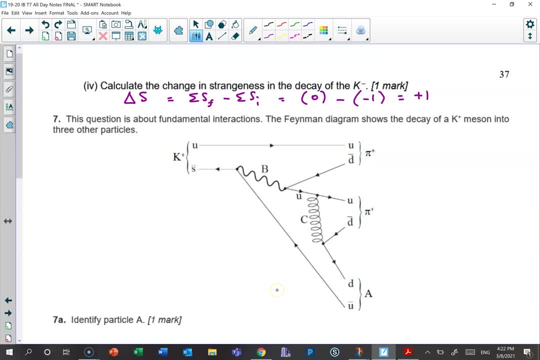 And so what do we need to know? Identify particle A? Here it is. You don't have to look, Look at the diagram. All you have to do is say up and down. Remember combinations of up and down. These are all pions, right? 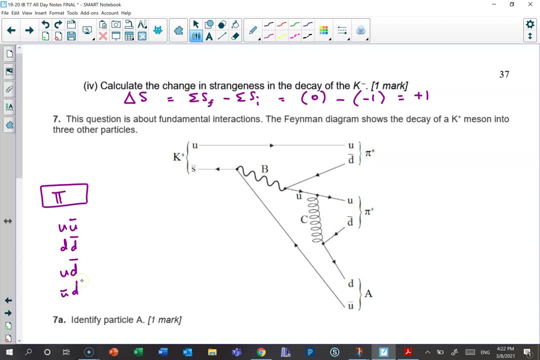 There are only four possible combos and I just listed them all. These two are neutral. This and this, I literally forget which is positive and which is negative. I mean, let's look at the charge. That's positive. two-thirds Anti-down is negative. 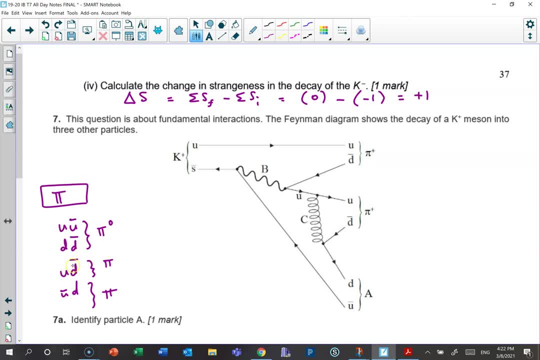 Down is negative one-third, but anti-down would be positive. You had two-thirds with one-third. This is positive. So that's the positive pion with its charge. positive one. This is the. what is this? This is negative two-thirds because you flipped the sign for anti-matter. 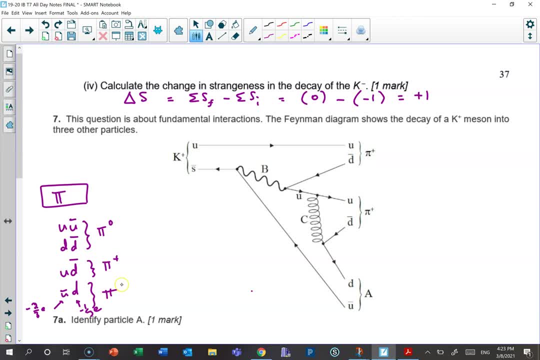 That would be negative one-third. That's its normal charge. Add them up and you get the negative pion. IB loves pions. Maybe they just like pi, Maybe I just like pi. Okay, so down and anti-up. What is it? 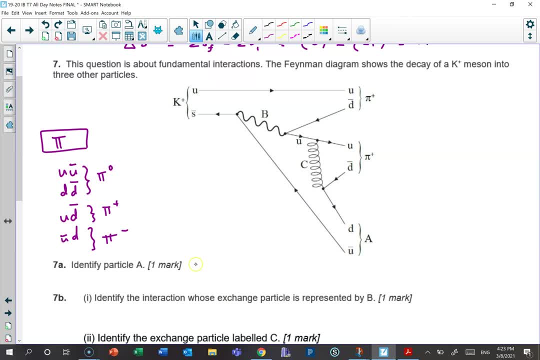 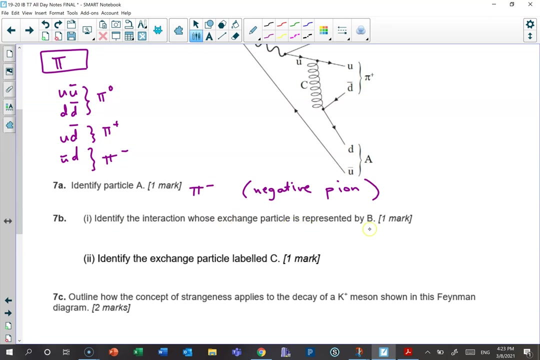 A negative pi particle with a negative pion, Not to be confused with the pions, right? Aren't those the proteins that form in the brain when you have mad cow disease? I think so, Okay. identify the interaction whose exchange particle is represented by B. 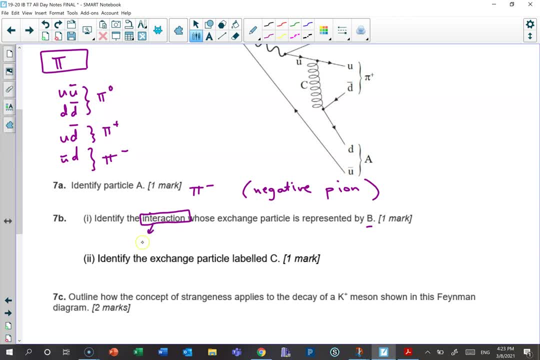 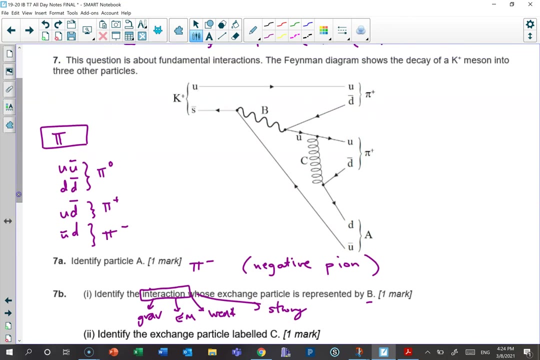 The interaction so they're talking about like: is it gravity? is it the electromagnetic? It's not going to be gravity. You'll never see gravity in these pictures, The weak nuclear force, or the strong. Let's see B. here it is. 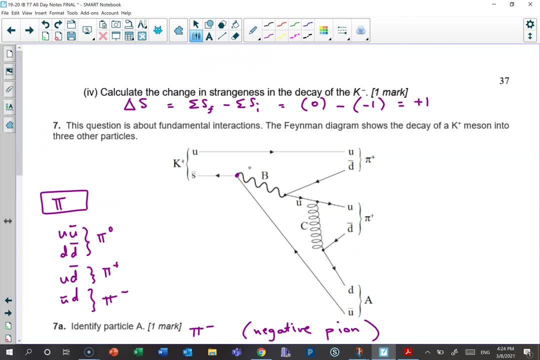 How do you figure this out? Well, here's my first thought. Maybe I can look at the anti-strange: What's going to happen? What's going to happen? What's coming out here? Oh my gosh, It goes all the way down. 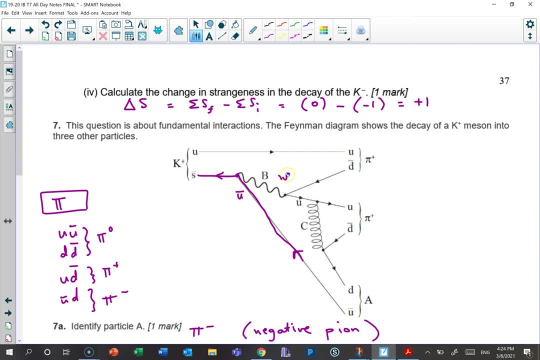 Anti-up, And maybe I can figure out like this has to have a positive charge, because if so, it has to be the weak interaction, right? Although as soon as I say this, that right, there is enough to answer the question. 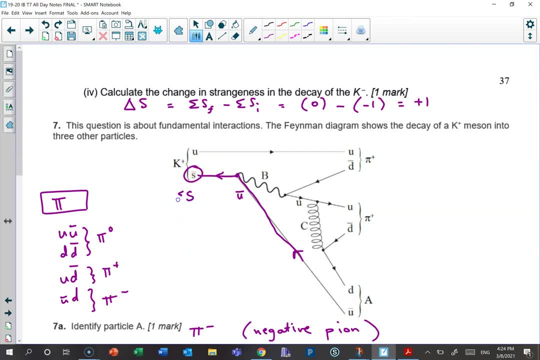 You have initially a strangeness going into this vertex right here. The total strangeness entering is positive one. Okay, Positive one, It should be negative one because it's anti-matter. But for strangeness, when you're counting strangeness, you flip it. 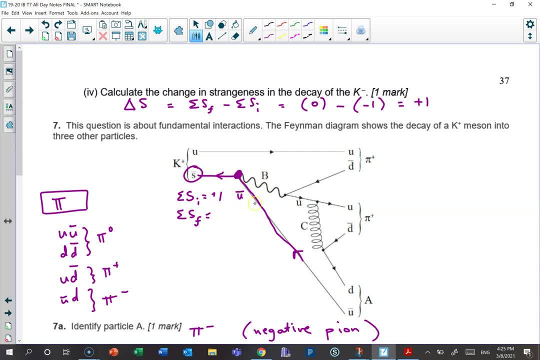 The total strangeness. exiting how many strange quarks or anti-strange DSE later in time, after this interaction, after this vertex, rather like exiting the vertex, I should say There are no strange quarks exiting the vertex. Even if there was a strange quark over here somewhere, it wouldn't count because it's. 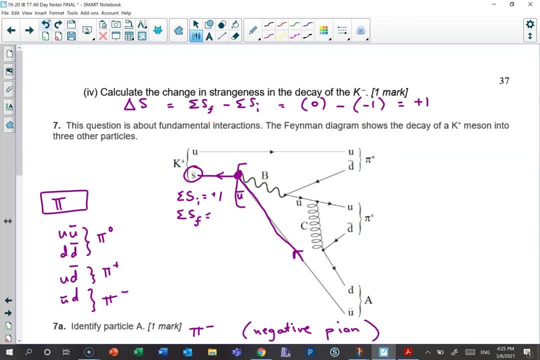 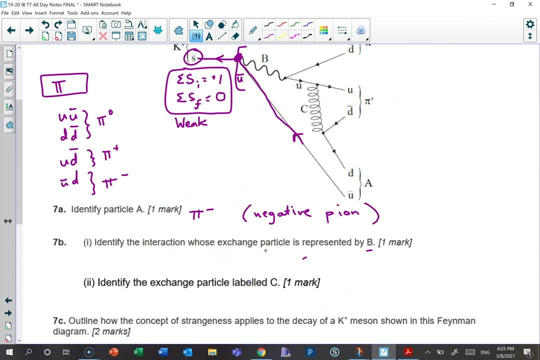 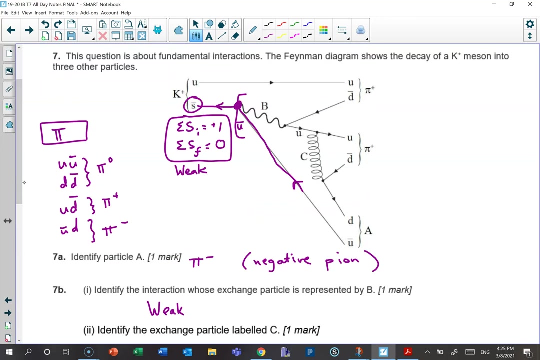 not touching this vertex that I've drawn. Okay, So the total is zero at the end, and this is only possible for weak interactions. You only violate strangeness conservation with weak interactions. Could you use electric charge to answer that question? Let's see. 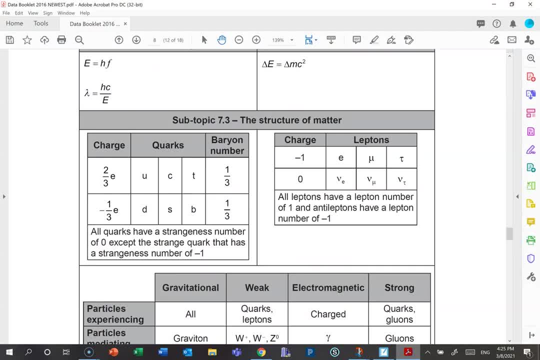 Entering the vertex is anti-strange, Exiting is anti-up. Anti-strange would be positive. Okay, So anti-strange would be positive. two-thirds Anti-up would be negative. Yeah, So you could figure it out using electric charge, right? 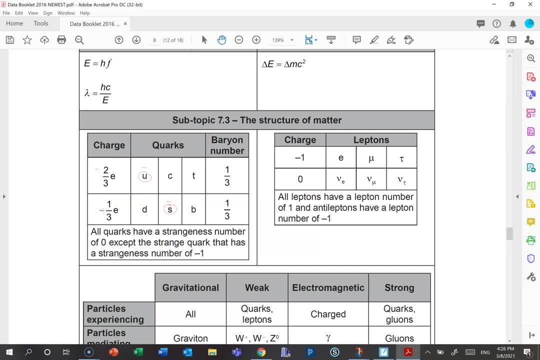 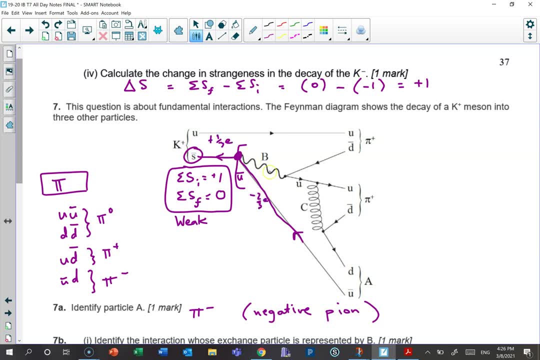 You would have positive one-third going in and negative two-thirds going out. And so what does this have to have? Positive one of electric charge, Positive one times the elementary charge. It would have to be the W plus boson, But don't put that down. 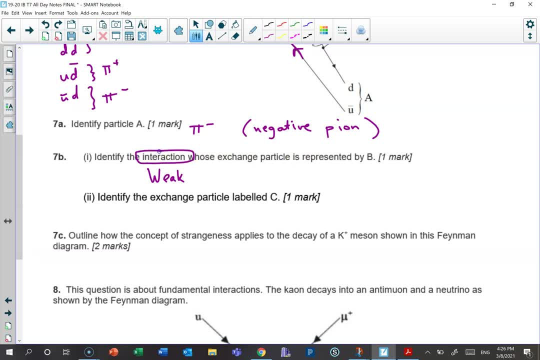 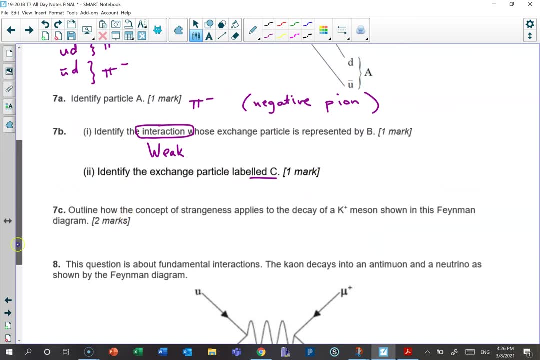 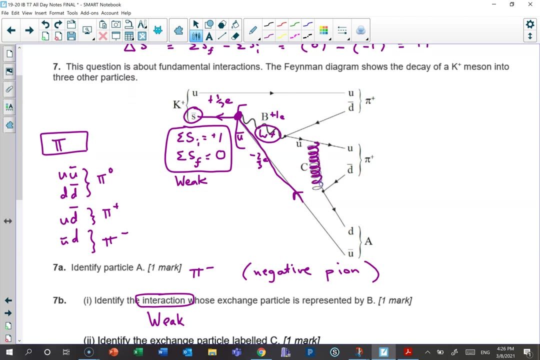 They're just looking for which interaction? Yeah, Identify the exchange particle labeled C C Again. as soon as I see that squiggler, the squiggly line, this is squiggles. As soon as I see that, I think gluon. but let's look and see. 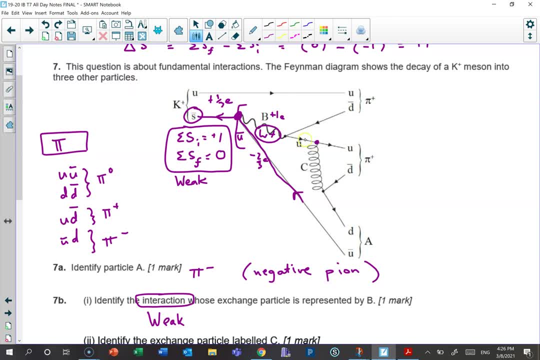 Okay, Okay. So you have this up, stays up, and this pops out, and then it turns into anti-down and down. Hmm, This is tricky. I'm going to be honest with you here. I'm pretty sure it's a gluon, because that's just. I don't even know what this is based. 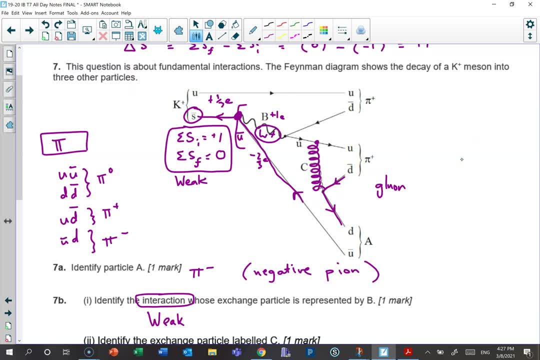 on my own understanding. Okay, So I'm going to go with this. Is it a gluon? Hmm, Maybe it could be When you look at charge, electric charge. there's no help here. Oh no, It's going to be a weak interaction, I think, but I'm not sure how you know that. 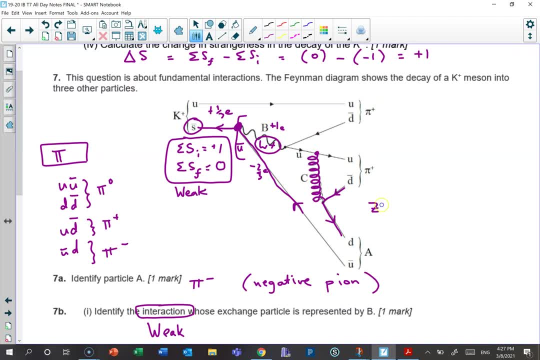 Yeah, Let's skip this one. The problem is it could be Z zero, But you can easily figure out that it has zero electric charge, zero times the elementary charge. but that leaves you three options. g here is gluon, not graviton. it could be the weak. 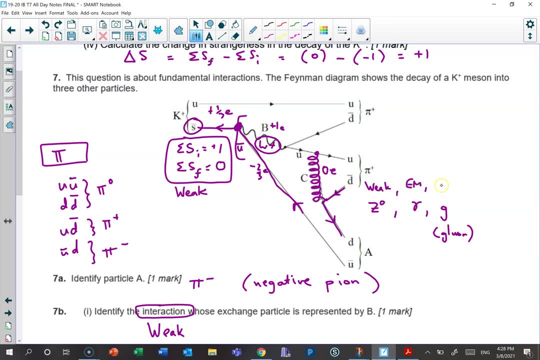 it could be em, it could be the strong nuclear force. my initial reaction was it was a strong nuclear force, but i think that mostly acts when you're looking at um, like taking a cork and pulling or a uh, a meson or something and pulling it apart. 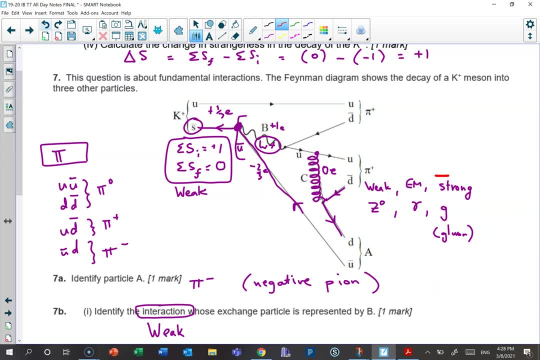 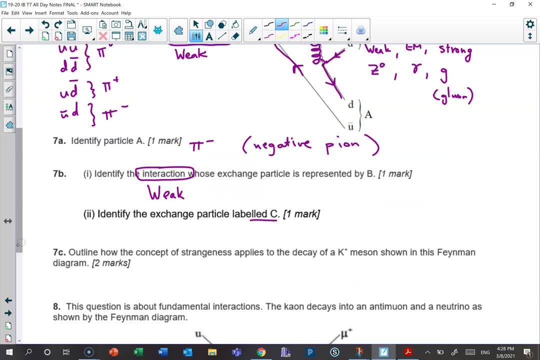 i think that's primarily where ivy's going to show you this. but the fact that there's a squiggly line, i'm not sure it makes me think gluon. yeah, i'll have to. i'll have to get back to you guys and post something in the um. 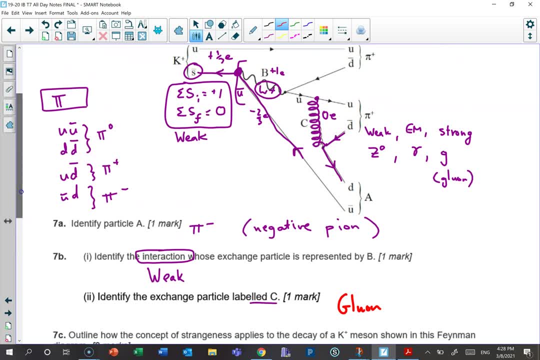 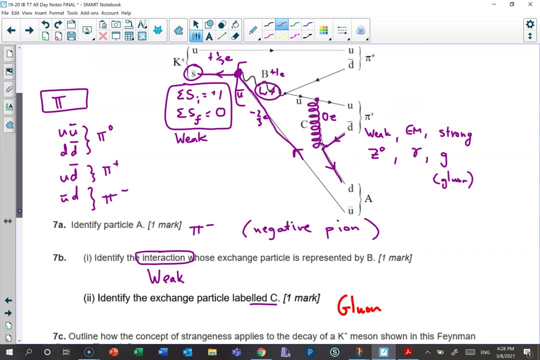 i'll look at this. this was a. this was an ivy test question at some point, so i'll look and see what they said and how they- how they think you're supposed to know. but, um, i'll post something in as a comment or in the description. 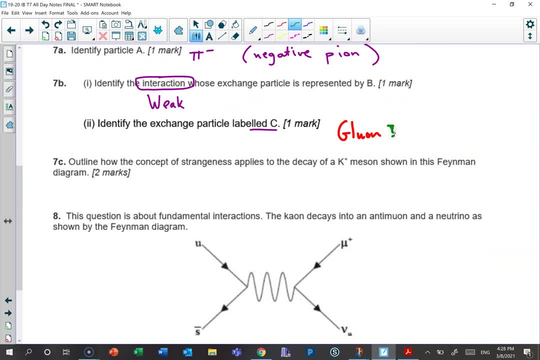 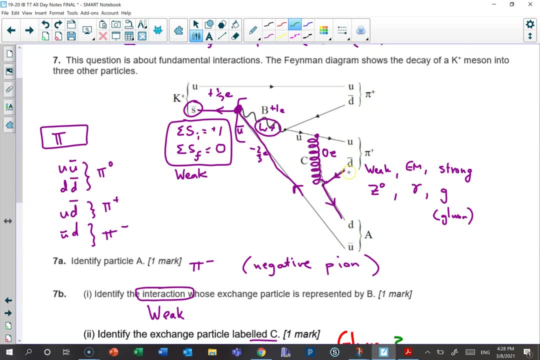 oh, it doesn't violate. there's these other things the same way. strangeness can't be. uh, has to be conserved, except with weak interactions. um, you also have to conserve, like the the up core, the number of up quarks. we don't learn these rules. you have to conserve the number of down quarks. 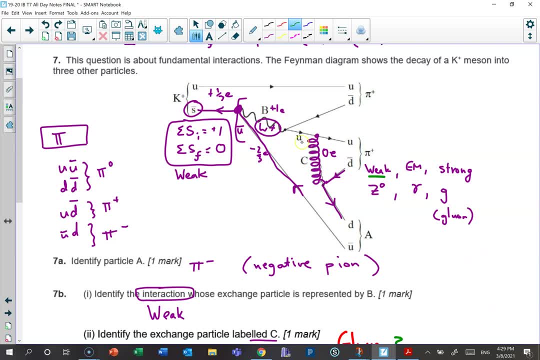 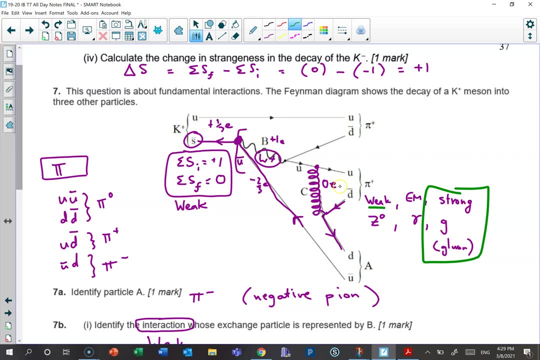 all this kind of stuff is is still true, unless it's weak interaction, but you do. those are all conserved. so i'm pretty certain. then i'm pretty positive it's. it's gluon. but i'm not sure how they think you're supposed to know that, except maybe because of the squiggly lines which are 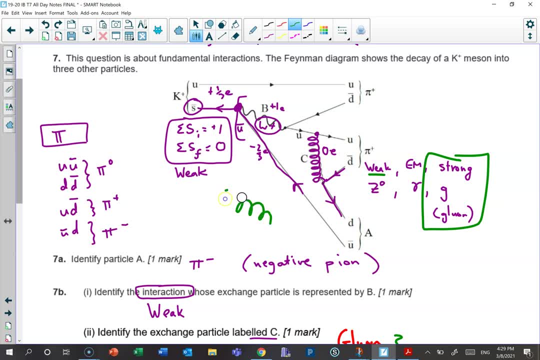 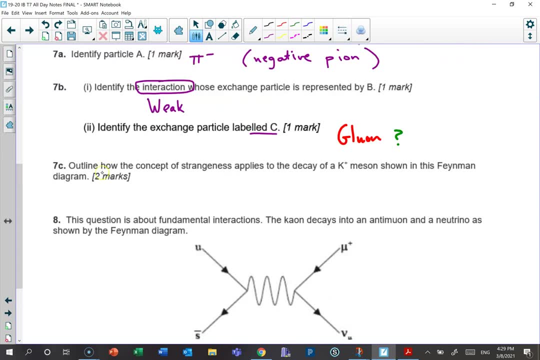 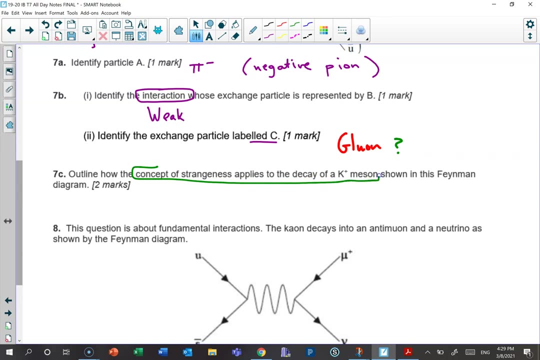 usually that kind of loopy line is usually the gluon. yeah, hard question. maybe that's not a fair one to ask, probably not? i mean, it is ivy physics, right? okay, how the concept of strangeness applies to the decay. when you see that you want to immediately think strangeness is conserved. i haven't even looked at this. 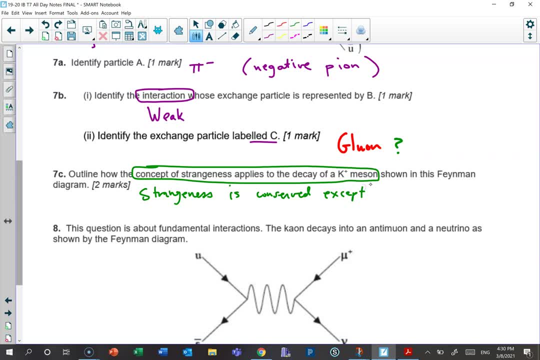 um, except strange, how you say. the strangeness must be conserved, except during weak interactions. that's the rule about strangeness, that's the concept of strangeness. so i've stated it. it's a two mark question. how does it apply? how does what i just wrote apply? i'm guessing the 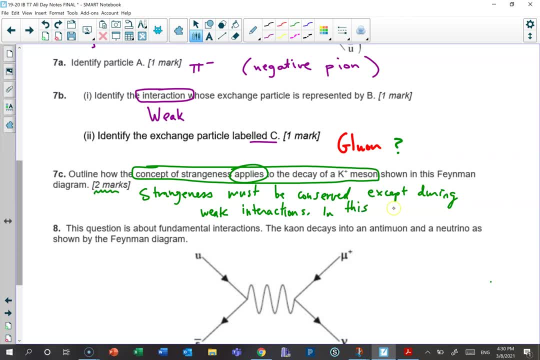 answer is in this interaction. let me apply it. so what happens if i'm going to pass up a string? so i go strangeness and i'm going to reveal it. let me solve a string Zombie. so I'm gonna go with get strangeness and I guess it changes. 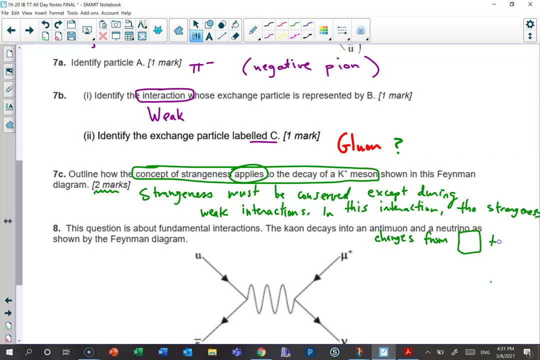 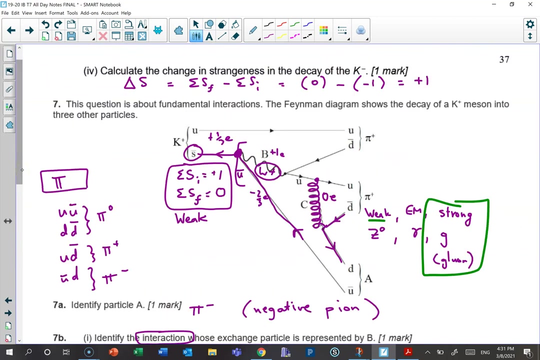 you can typeyard the strangeness and I'm guessing it changes. you can type strangeness changed from and I'm going: Maybe due to the weak interaction. Let's look and see. Am I right in my guess? Yeah, Look at the total strangeness at the beginning moment. 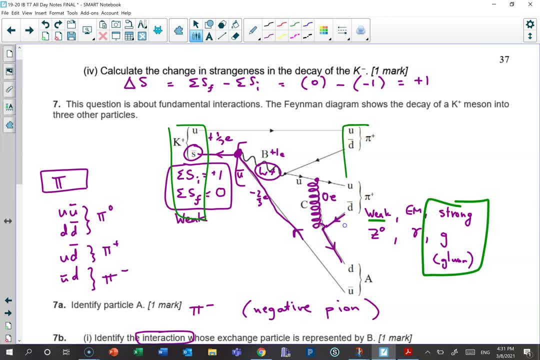 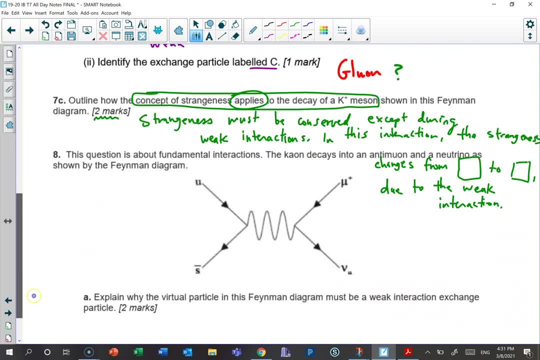 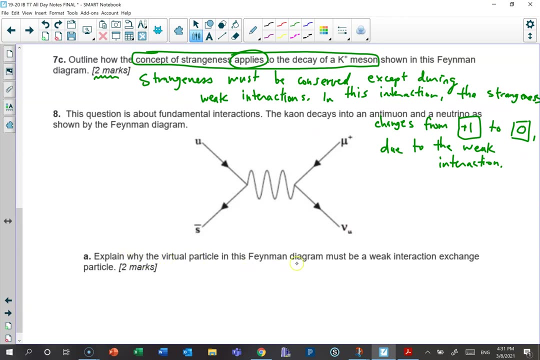 It's positive one. I said earlier, What do you have at the end? The total strangeness at the very, very, very end is zero. So let me add that in Explain why the virtual particle must be a weak, It's the same question. 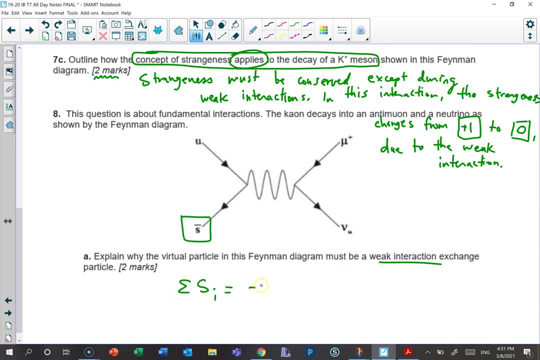 The strangeness initial is: You would think it's negative one because it's antimatter, but for strangeness you flip it. At the end it's this: There are no strange particles at the end. How do I know time access is going this way? 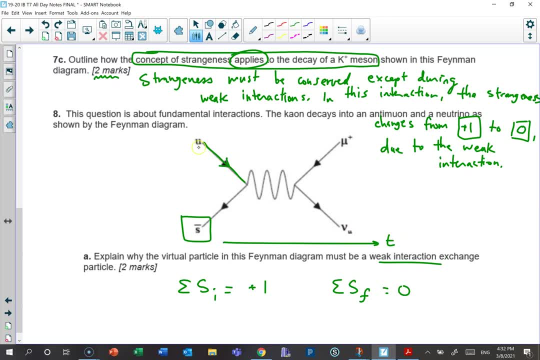 Because I see the up quark and I say it has to point with time, Because it's matter, not antimatter. And that clues me in to where the time access points. I guess this could also work right, But if you drew your time access this way, 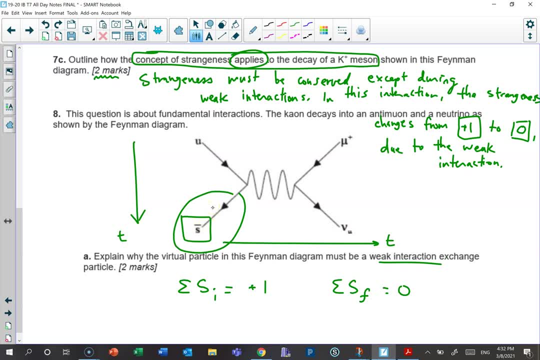 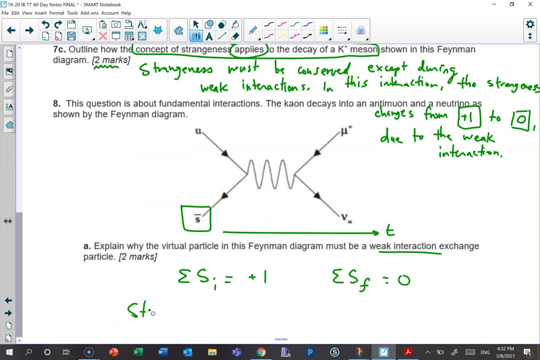 now, anti-strange is not against time and that's problematic. So this is the only possible time access. And so what are you saying? Strangeness, must It, can. It can only change during weak interactions. That's how you know. 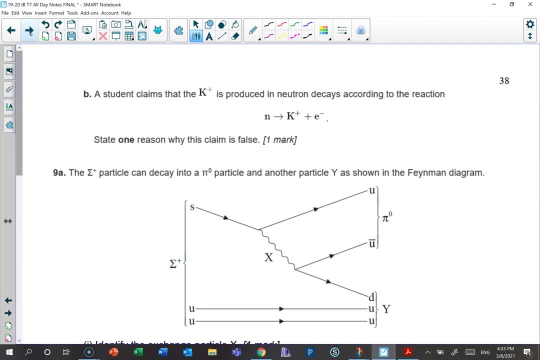 A student claims the K plus is produced in neutron decays. Huh, can the neutron decay? What's one reason why this claim is false? Well, there's an obvious thing. First of all, let's go look at what the K plus. 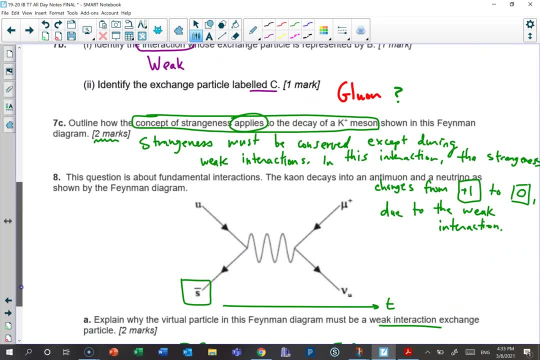 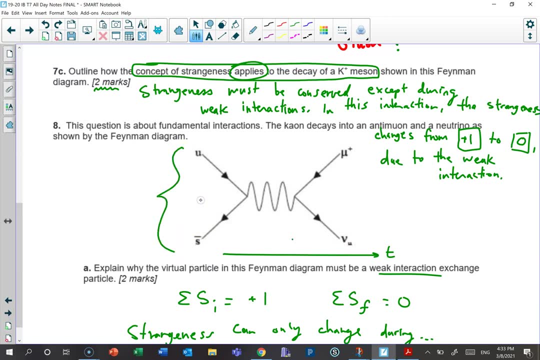 is again. Let's see, The K plus is Okay. so this is the K plus Those two things together up with anti-strange. See, they don't tell you that. You have to infer it from the picture. 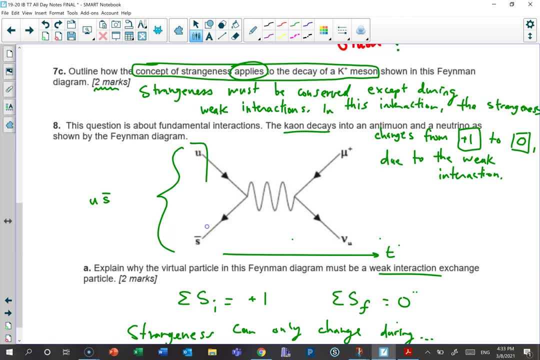 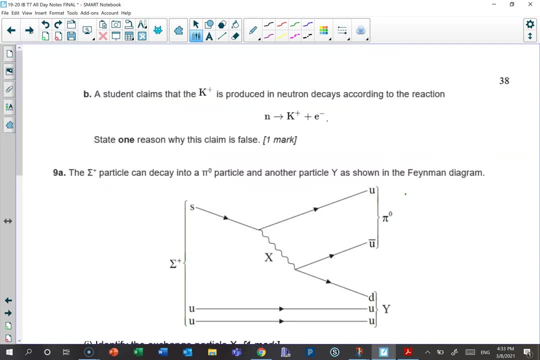 The kaon. Did you catch that? The kaon decays. So they're implying that these two particles together are a kaon. Okay, so the kaon they're saying is They're saying neutron changes to. Oh, I've already forgotten. 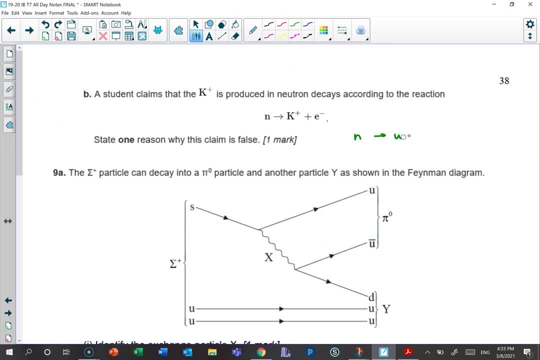 Up and anti-strange, isn't it? Plus electron. My dog is whining for my pets, So there it is. If I break up the kaon, I have this: What's the neutron? Neutron. The neutron, it's not a proton up up down. 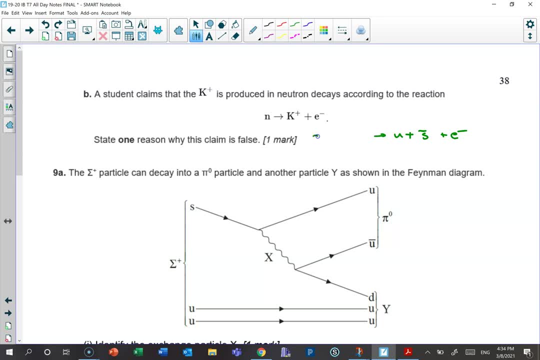 It's the opposite: Down, down, up, So down, And you can pretty clearly see the problem here. The total quark number: there's a lot of reasons. The total quark number at the beginning is three And at the end the total quark number is zero. 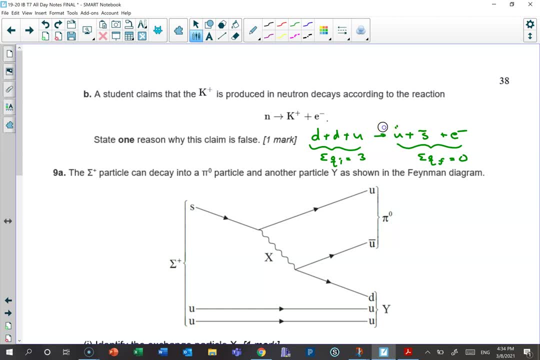 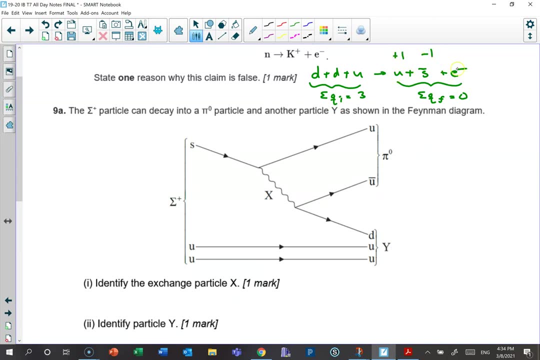 That counts as positive one quark And the anti-quark is negative one. This is a positive quark, That's a quark, That's an anti-quark. So you add them to get zero. That's not a quark. 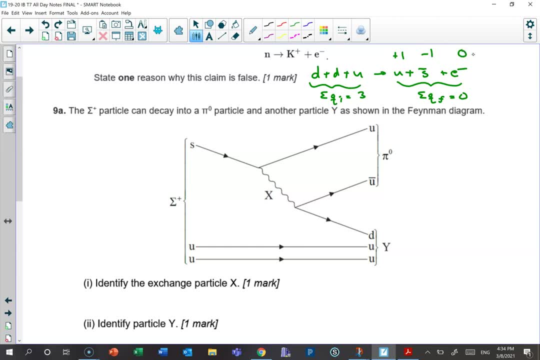 So it doesn't count for anything when you're doing quark tallies. So that's one reason you could explain. What about charge? I'm betting the Oh no, the charge is zero, The charge here is zero And the total charge at the end is zero. 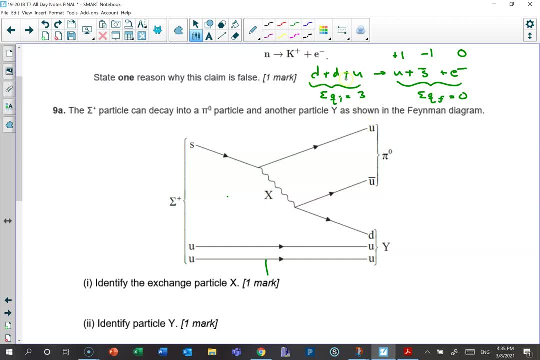 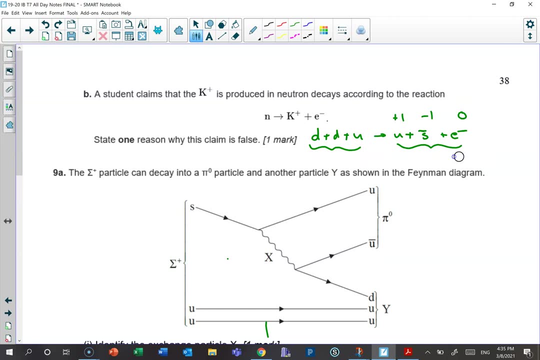 So that's not it. What about lepton number? That's the other one you could look for. The total lepton number should be conserved And you can choose the electron family. There are no electrons or electron neutrinos initially. At the end, the total lepton number in the electron family. 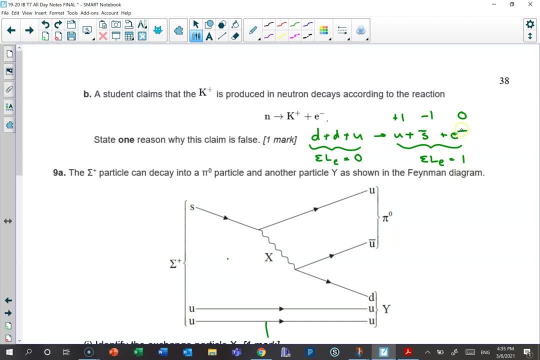 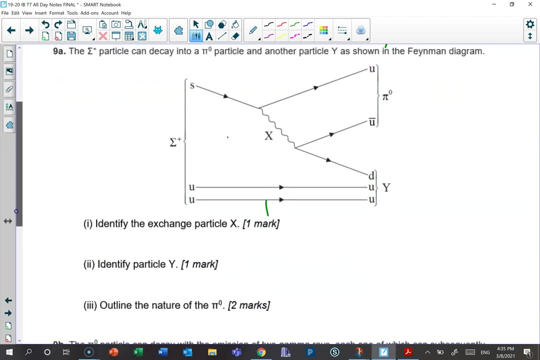 well, you've got one right there. It's a regular electron, It's not an anti-electron, So it's positive one, not negative one. And so you violated that conservation law, also The sigma particle, right? No, what is that? 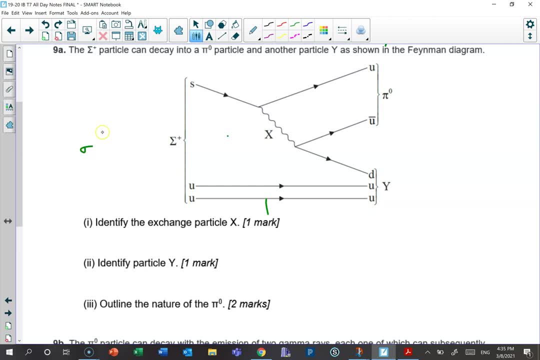 Some sigma. Yeah, this is lowercase sigma. right Capital sigma Can decay into a neutral pion. My dog is going crazy. And another particle y? Oh, look at how sneaky they are. What's y bruh? 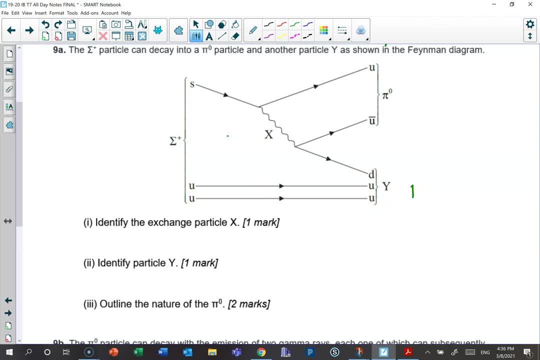 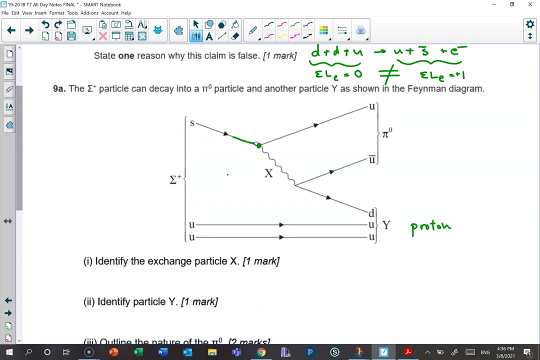 Up, up down. It's a proton bruh, You can't fool me. IB, As shown below. Identify the exchange particle x. Okay, The first thing I see, the total strangeness entering the vertex is negative one. 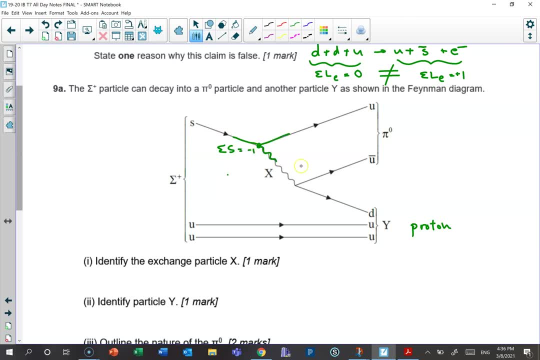 And the total strangeness exiting. neither of these are strange. So I know x has to be one of the force particles for the weak nuclear force. How do I know? Because the strangeness is not conserved, Only the weak force does that. 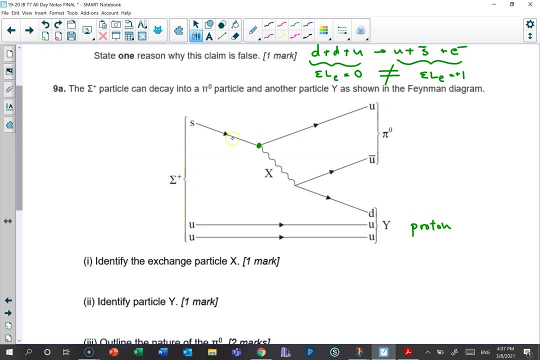 Changes the total strangeness. All right, Let's look at our chart. Strange is negative one-third of electric charge. I just have a hunch that the electric charge is not going to balance Up when I don't know what to do. usually that's what I go for. 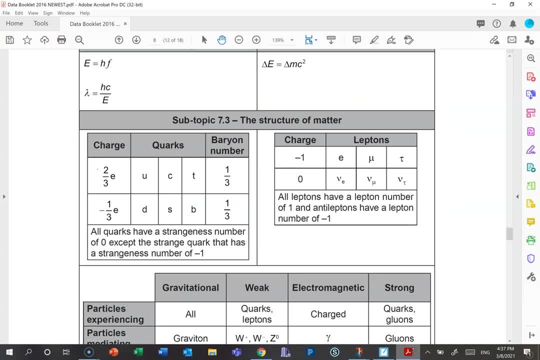 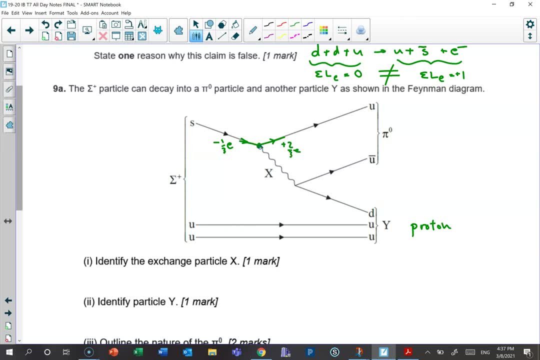 Does the electric charge not balance Up is positive two-thirds e, Yep, So currently it doesn't balance. How do we get it to balance? This guy must be a total charge of negative one e, because then you add and the total charge exiting now equals the total charge entering. 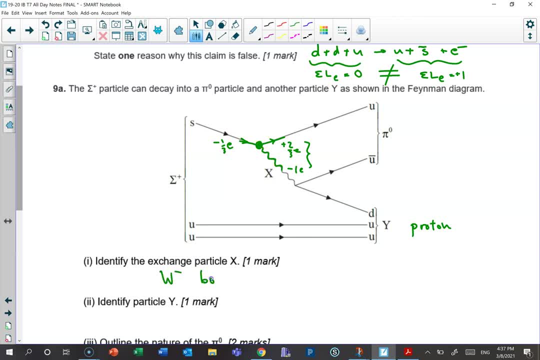 So what is x, x, W minus boson? Identify particle y Proton. We already did that. As much fun as it would be, please do not on your IB exam. please don't write proton bruh With like. 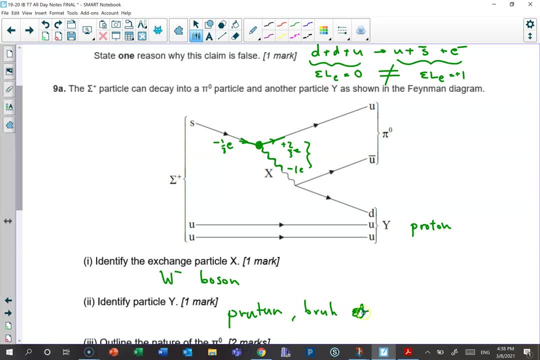 bruh giving a thumbs up In his baseball cap. That's what bros wear. Here's our bro. Don't do that, As tempting as it might be, Maybe double thumbs up. Oh, that's really doing it, Bro. scale is off the charts. 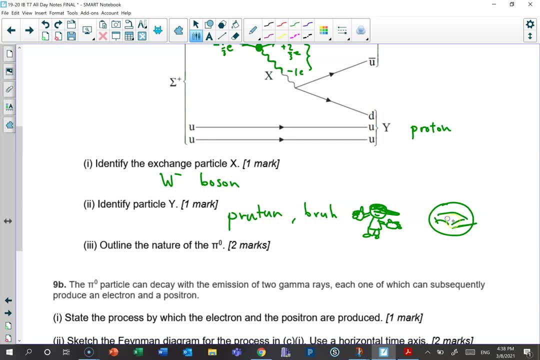 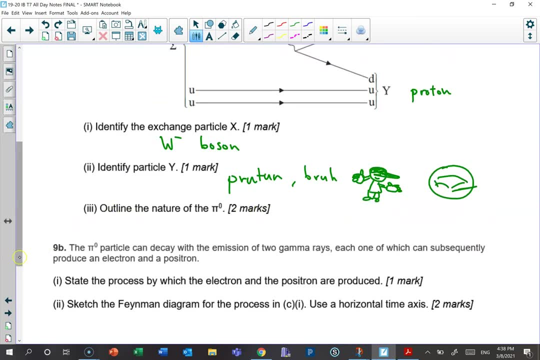 Breaking the bro scale. Okay, I need to move on. Long video: Congrats if you've made it this far. Outline the nature of the pi zero. What are they saying? Nature, What do they mean? It's a meson. 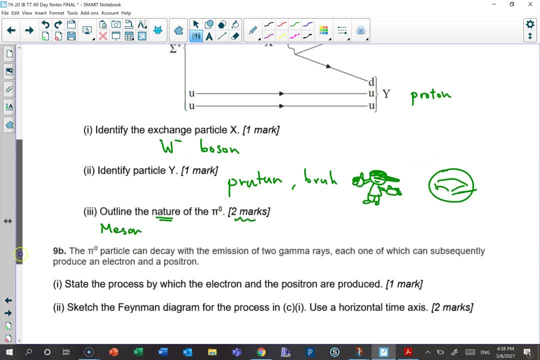 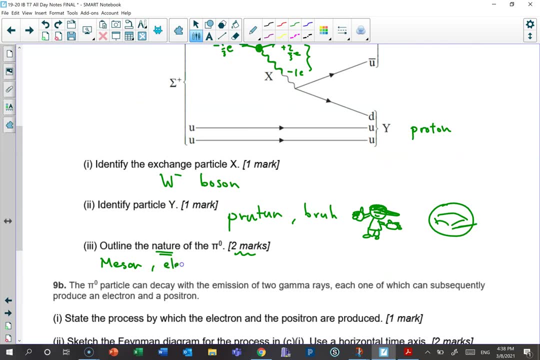 That's got to be one of the marks, right? It's a meson. It's neutral, Electrically neutral. Oh, I wonder It's electrically neutral? It's very short-lived because it annihilates itself. It's hadronic matter. 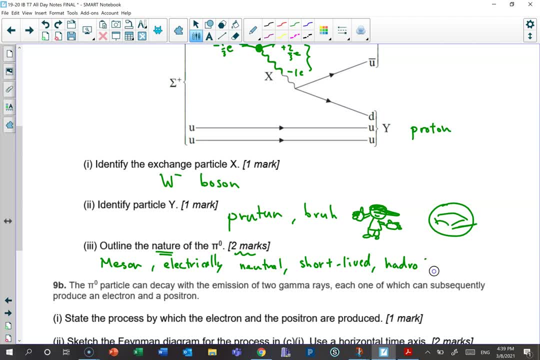 because it's made up of quarks and anti-quarks. You could just say it's a hadron. That's kind of the simpler way to do it. What is this still doing here? It's a hadron because made from quarks. 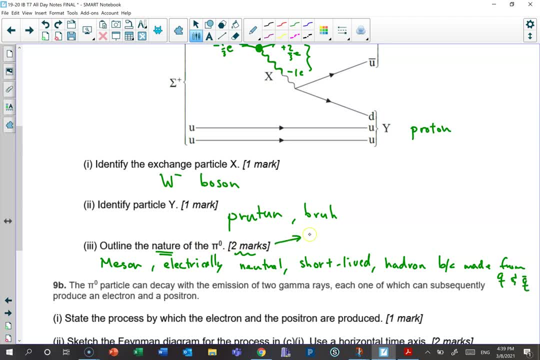 The nature. You could also probably say, as a potential answer, it mediates. Do you know this? There's a video on it. It mediates the nuclear force between protons and neutrons. If that doesn't make sense to you, 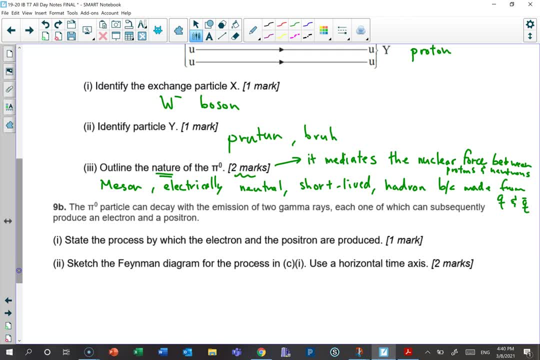 go watch my other video. Like comment, subscribe. I'm just getting you to watch more videos. Of course, a two-minute video is not the way to achieve that, but anyway, I think any two parts of this would earn the mark. 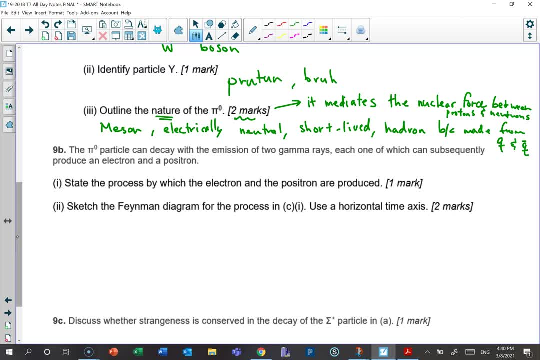 The neutral pion can decay with the emission of two gamma rays, each one of which subsequently produces an electron and a positron. Wow, That's cool. We're going to get to draw it in part two, But first, what is the process called of producing the electron and a positron? 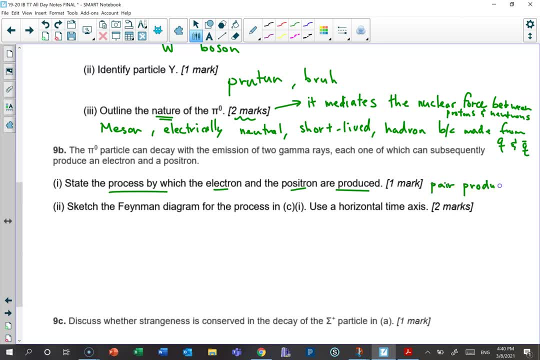 Producing the pair is called pair production. We are fancy. We give ourselves smart terms, smart-sounding terms, so we can impress our friends at parties. Pair production: Okay, Use a horizontal time axis to sketch what they've just described. 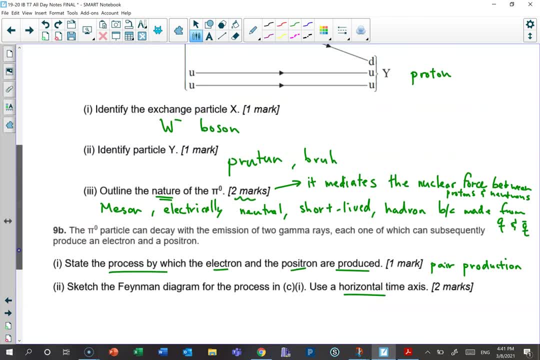 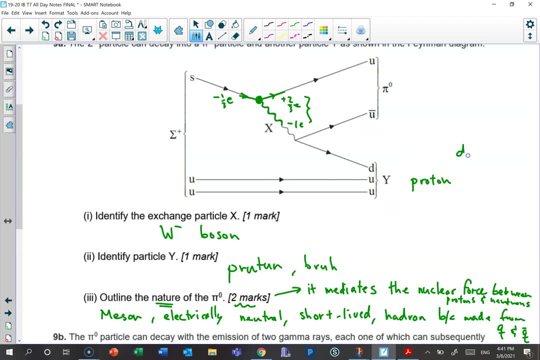 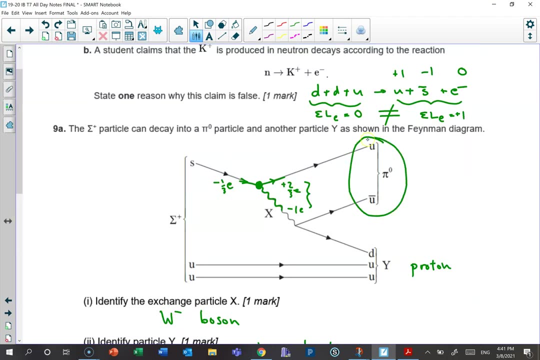 You start with a neutral pion And did they tell you which one to use? Yeah, Up and anti-up, Down and anti-down would also be acceptable. But because they told you the pion is up and anti-up, we'll use that. 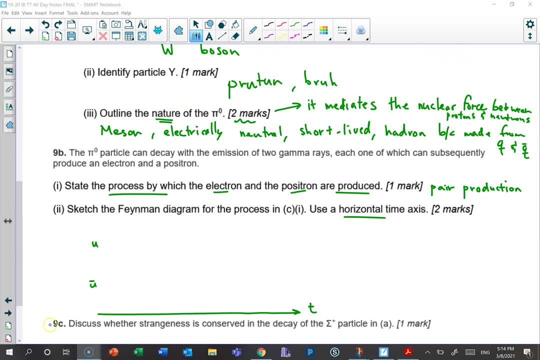 So I'm going to start with up and anti-up Now. I'm guessing that you're probably going to do something like this: the first attempt you make Up and anti-up. you know that they have to annihilate right, And then they will pair produce. 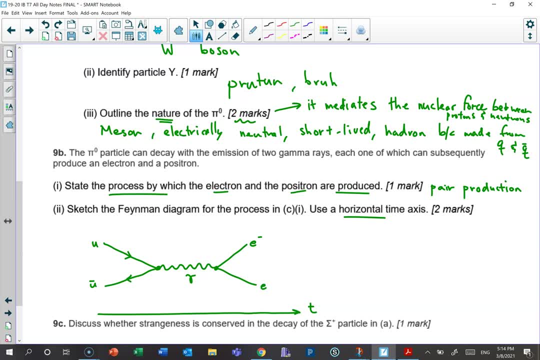 But hang on, We've only got one photon. Here's the electron, There's the positron. The electron is matter, The positron is anti-matter, But we need a second photon, right? And where does that second photon get created? 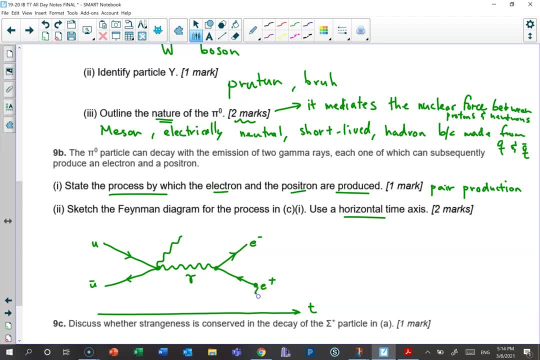 You can't do something right here, You can't have it come off right here, because now the electron is no more And so actually it doesn't take too much. You know, you have to have seen this kind of thing before in order to get it. 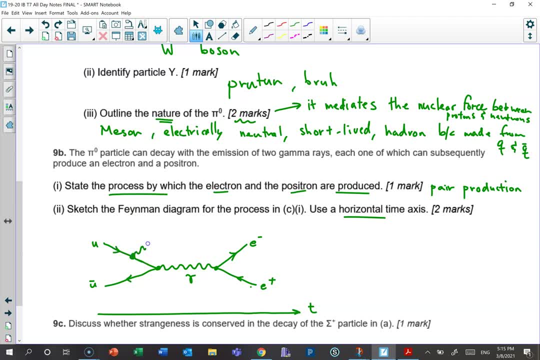 But you can say: well, hang on, What if the up quark emits a photon just like this, and then that photon does pair production, And that's right. That's the answer. Now you can actually take that extra photon and you could put it right here if you wanted. 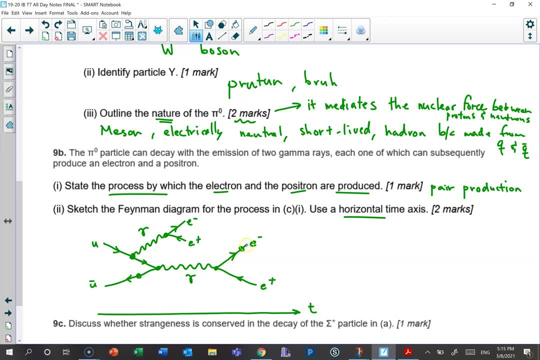 Or even right here. Maybe this electron has a little extra energy at the end, Or you could do it right there And in fact all of those would be acceptable answers. And when you do different drawings like that, we haven't talked about this. 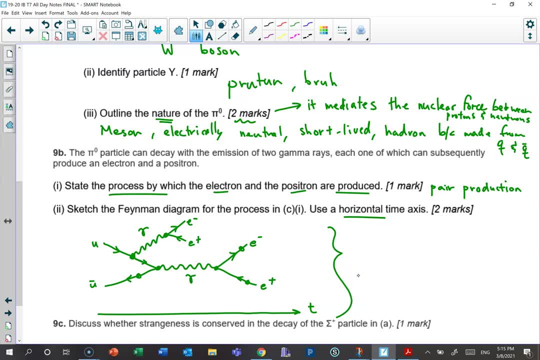 but literally Feynman diagrams are visual representations of equations. Every diagram is an equation And those different possibilities I just showed you, you would have to add those all together, weight them according to their probability, do some integrating. I think this is correct. 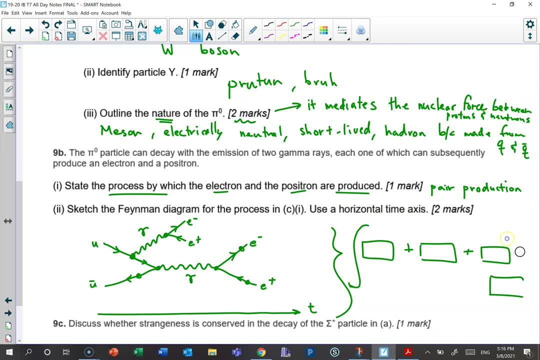 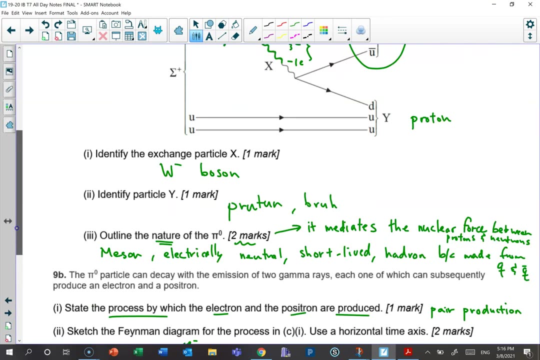 But there's something along those lines. So you use those equations for additional math. But the genius of these diagrams is that you can represent equations with a picture. Okay, Discuss whether strangeness is conserved. How many times are we going to do strangeness? 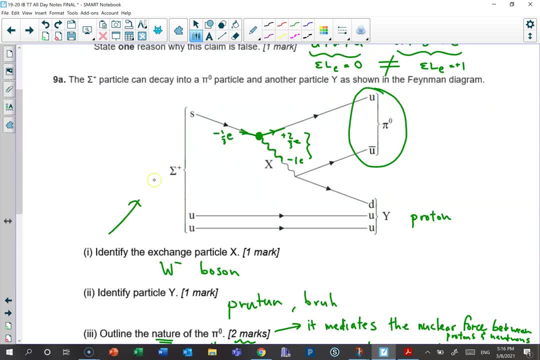 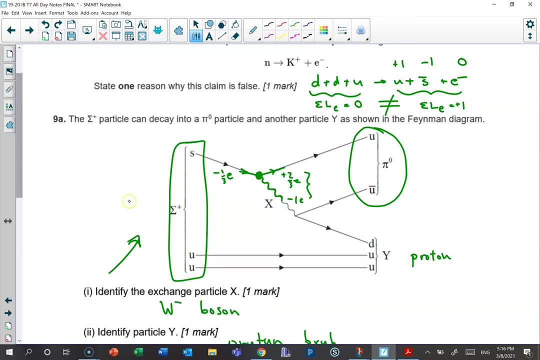 Ugh, Here it is, This one here. Is strangeness conserved? Well, probably not. I'm just going to take a wild guess here and say: Let's look though The strangeness. initially you would think it's positive one. 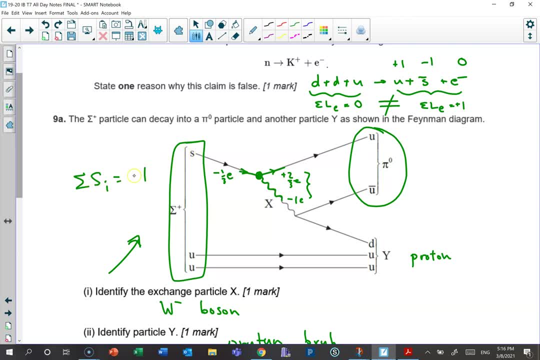 but actually because this is just regular matter. but with strange particles, strange quarks, we do the opposite sign And at the end, if you look at all the particles at the end, up, anti-up, down, up-up. 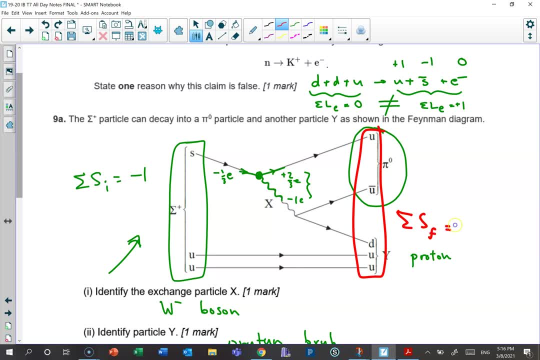 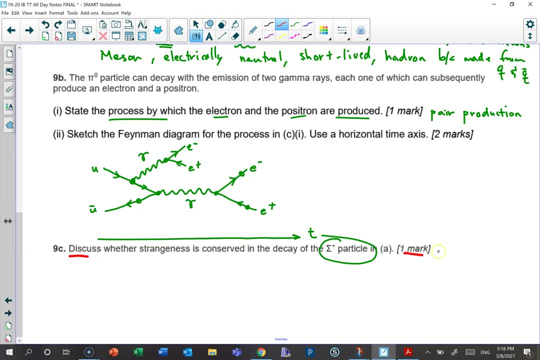 there are no strange particles there. So first, if they say discuss, I'm already expecting two points, It's only one, but you know. But if they say discuss, you have to say the initial strange value, and you say this with words. 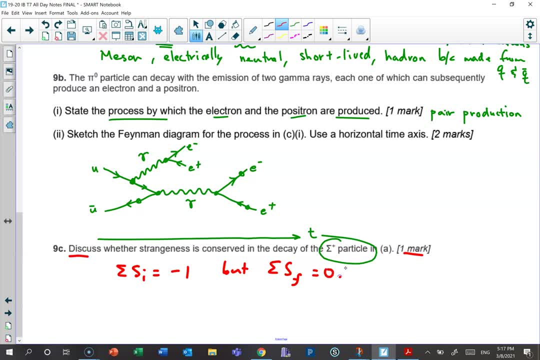 not just symbols, not conserved. That's worth pointing out. When they say discuss, what are they looking for? Just to be safe, I'm going to also say not conserved, and thus the interaction, you know, thus this decay. 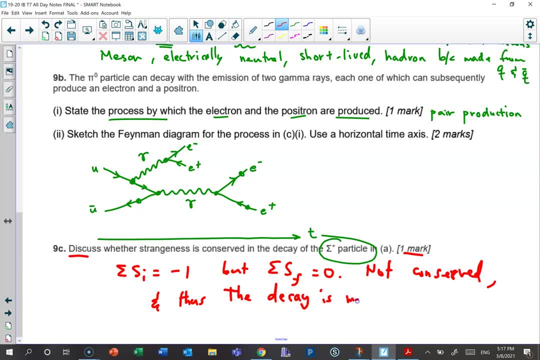 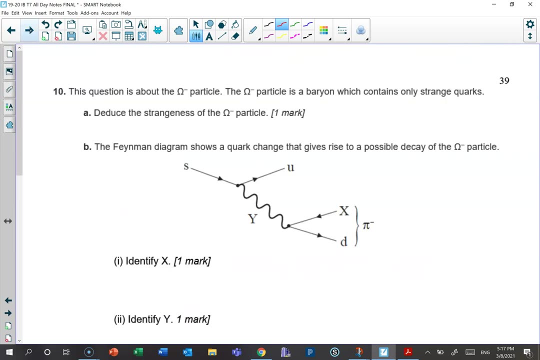 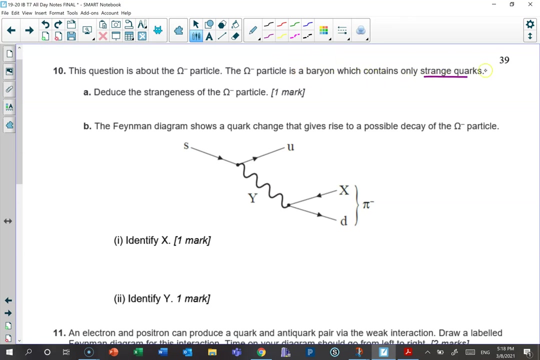 is mediated by the weak interaction. Okay, Next one, Let's go to purple. So we've got the omega minus particle. It's a baryon. So we know already that it has three quarks or three anti-quarks. What do they tell us? 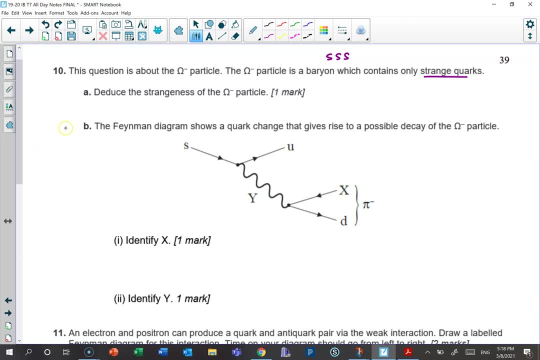 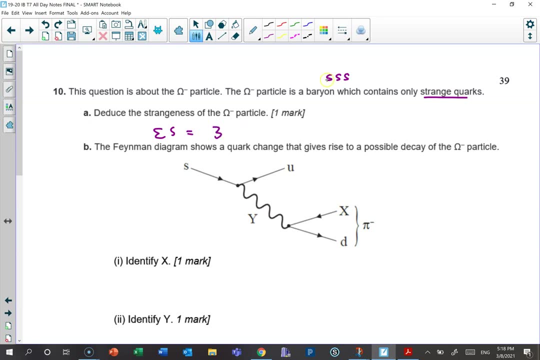 Three strange quarks. What's the strangeness? Deduce, What a fancy word for add. Okay, You would think that it's three, because they're matter. but strangeness is strange, so you add the opposite sign, as what you would normally expect. 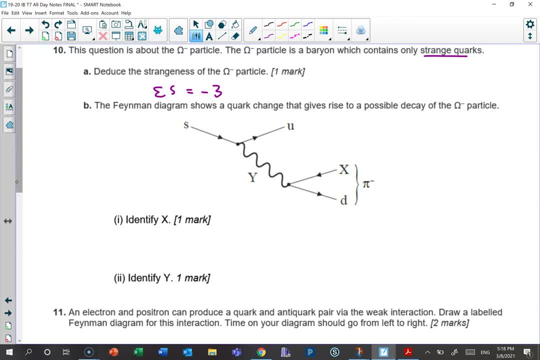 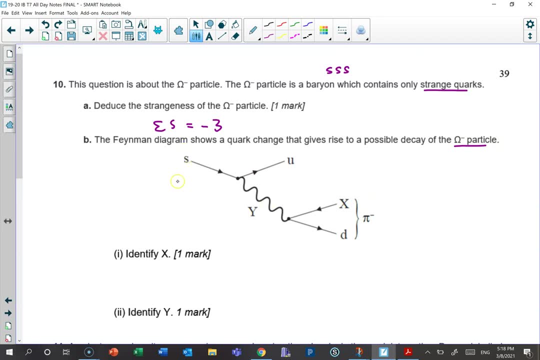 Okay, So here's our diagram for possible decay of this particle, The omega minus particle. Well, I thought there were. I thought the omega minus was three strange quarks. Where are the other two? Did something get removed from this diagram? 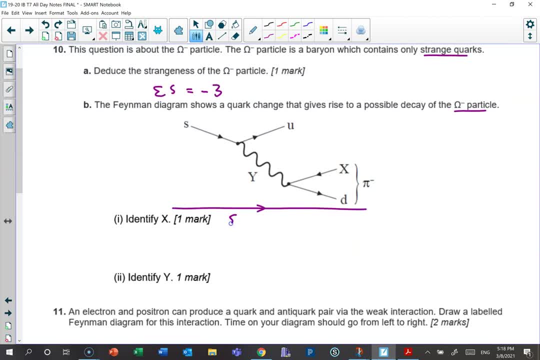 I don't understand. Is there supposed to be another strange quark that stays strange and then another, Or does this happen for each of the three strange quarks? This is confusing. I don't like this. Anyway, we can deduce that the time axis points this way. 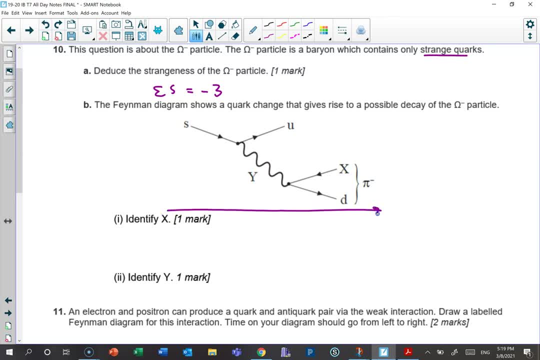 that we know and identify x. Here's x. Oh, it's a pion. You remember? pions There are. it's just a meson. so it's a meson composed of up and down, but one is anti-quark. 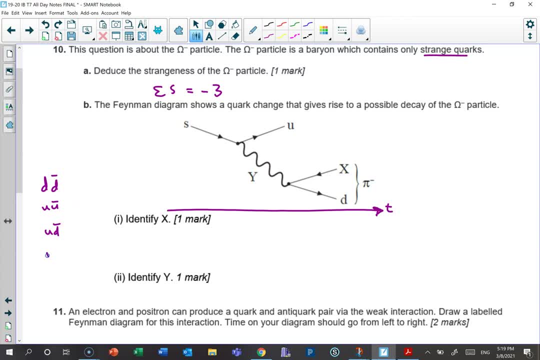 the other is quark, So you can literally write them all. There's only four possibilities. These two would be neutral. what's this one? Okay, that's up is positive two-thirds. Anti-down would be positive one-third, so that's the positive pion. 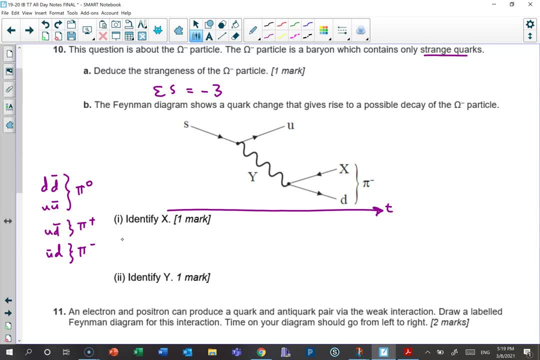 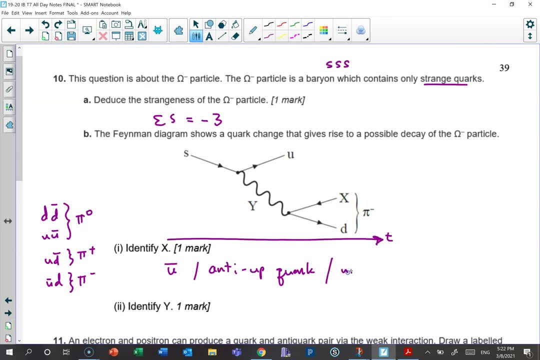 This one must be the negative pion. Yep, And so what's x? The anti-up quark. You could also call it the up anti-quark. That might be something you see. Lots of fun names. Okay, identify y. 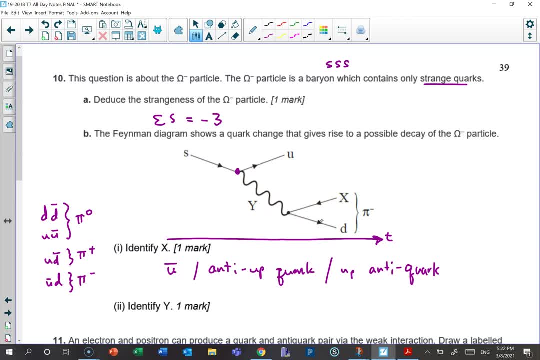 Y, we see, is an exchange particle. So you've got. I'm going to look at this vertex here to figure out what y is. By the way, let me just step back for a moment. Did you see that arrow? Because I didn't pay attention to that. 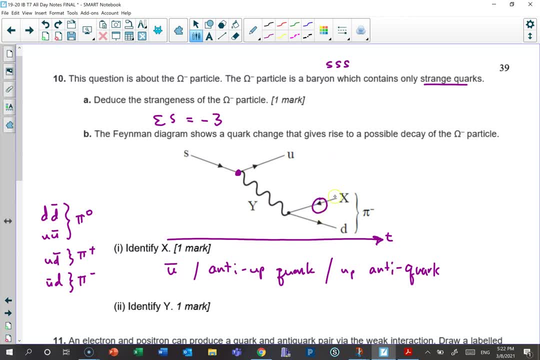 the first time I answered this question. As soon as you see that arrow, you say: well, x is either anti-up or anti-down, because pions are just a combination of ups and down quarks. So as soon as you look and say 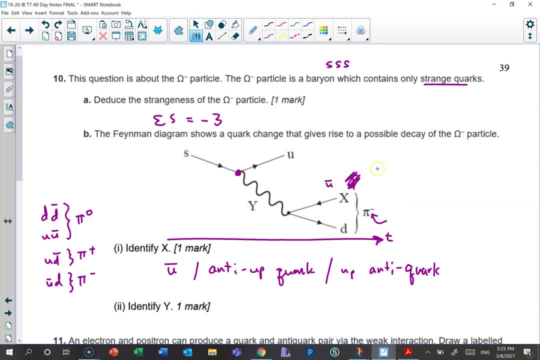 oh well, it's negative charge. you know that it can't be anti-down, because down and anti-down would be neutral, So that's maybe an easier way without going through all this business. Okay, identify y. If you look at this vertex. 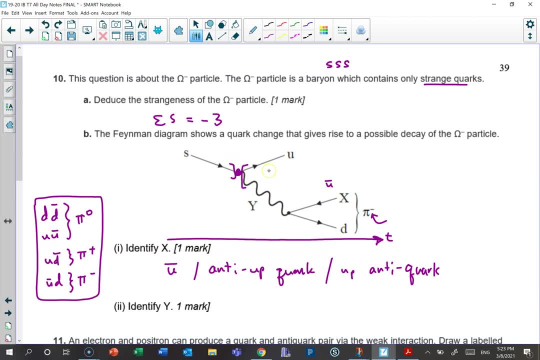 you'll immediately realize, strangeness is not conserved. So y then has to be a positive w boson, a w minus boson or a z. It's got to be the weak interaction. Let's look at the electric charge of strange and up. 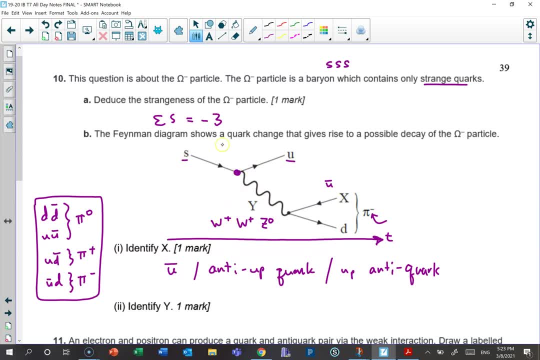 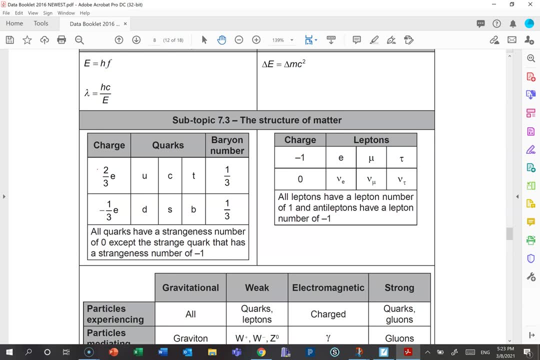 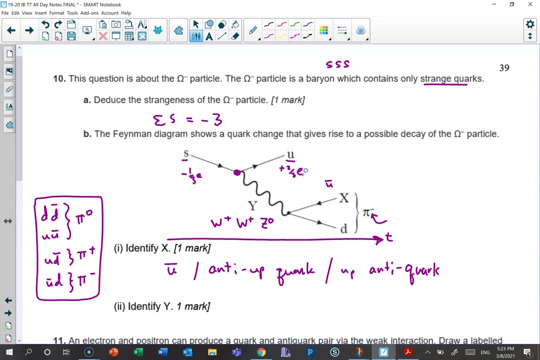 because if you can't hone in anymore, balancing electric charge is a great way forward. Okay, strange is minus a third, Up is positive two-thirds. So if you look at the incoming charge going into the vertex, it's negative one-third. 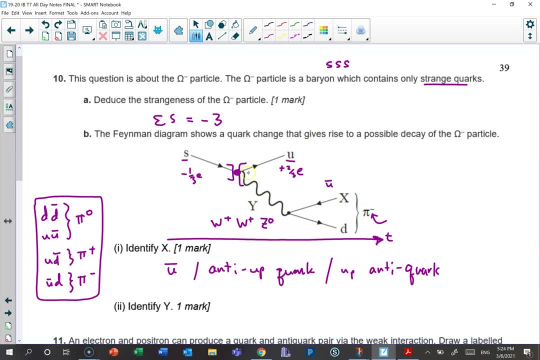 The outgoing charge exiting the vertex has to also total up to negative one-third. So if it's going to total at negative one-third and this is positive two-thirds, what's that charge got to be? Minus one, because now they add. 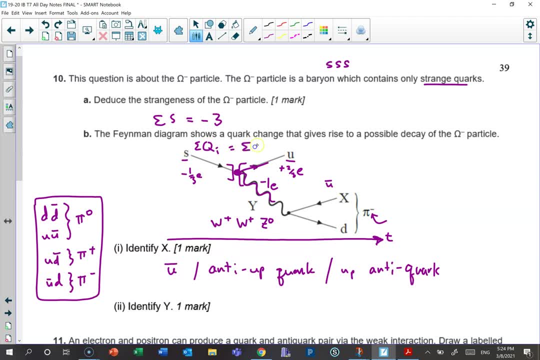 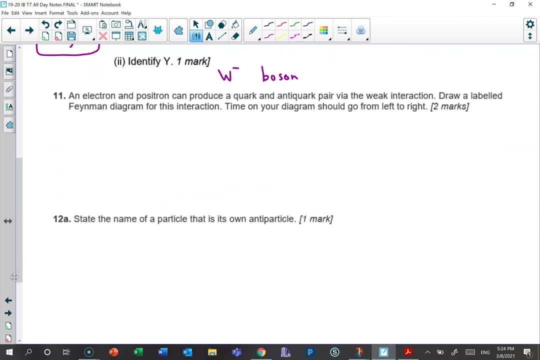 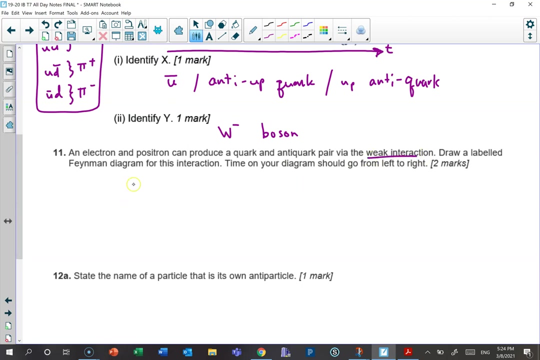 and now the total initial charge will equal the total final at this vertex. So it's a whoops. it's a w minus An electron, and positron can produce a quark and anti-quark pair via the weak interaction, The weak interaction. 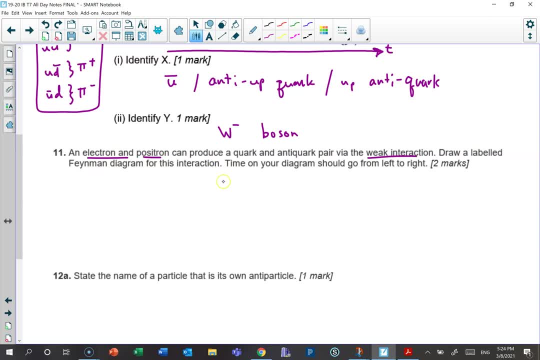 Electron and positron. draw a labeled diagram for this interaction. Times should go from left to right. This is probably pretty simple. Electron, oops, not particles, they're waves. Electron and positron, I mean, usually I think they annihilate right. 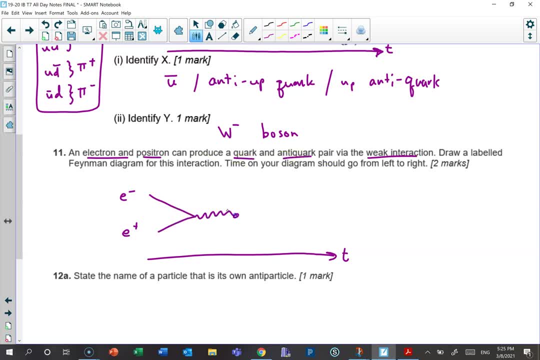 But what are they turning into? Quark and anti-quark? Does that work? Yes, Here's the quark, here's the anti-quark. We're not going to say any more than that, because they didn't say it's up or anything else. 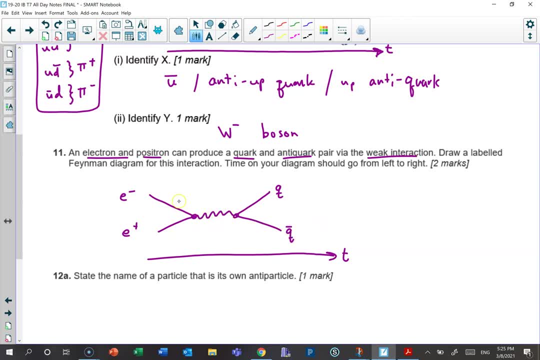 Cool. That's the weak interaction, so we have to label this First. let's add our arrows. Matter goes with time. Anti-matter points opposite, just as a way to say, hey, I'm anti-matter, right. 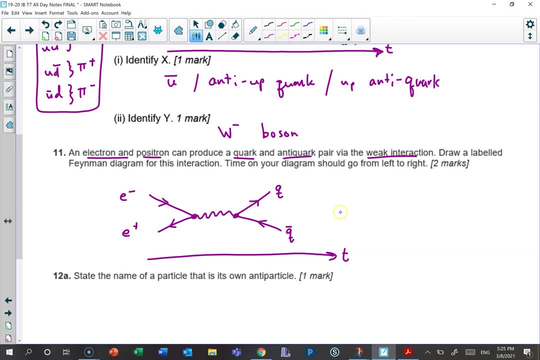 That arrow doesn't mean it's moving backwards in time, Although there's an interesting. there's an interesting way to say that, like the anti-electron, the anti-electron actually does behave as though it's well, I don't want to. 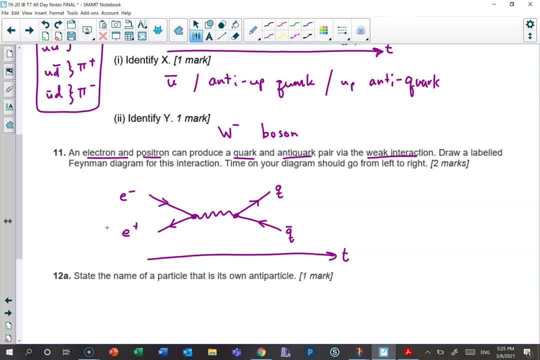 okay. so if there was a way for an electron to move backwards in time, it would look like the anti-electron. There's something in physics called CPT- parity Charge, or CPT transformations, rather, Charge, parity and time. 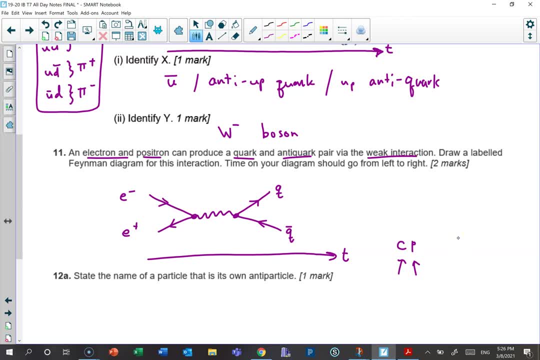 And if you do charge and parity transformations, you get an anti-particle. I think I'm remembering that correctly. There's a great PBS Space Time video. Check it out. So anyway, it's the weak interaction. so is this W plus or W minus? 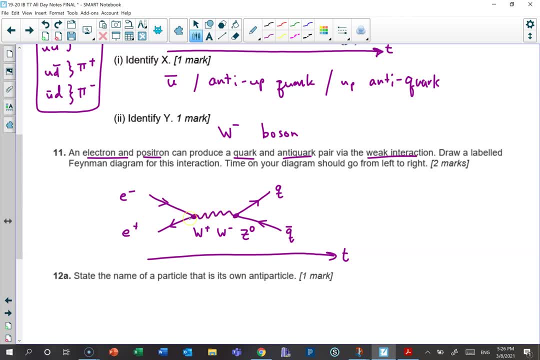 or is it Z zero? Well, look at your charge. This is minus one of charge, That's positive one, And so the incoming charge going into this vertex adds to zero. What's the charge gotta be exiting the vertex Zero. And so now I've finished my diagram. 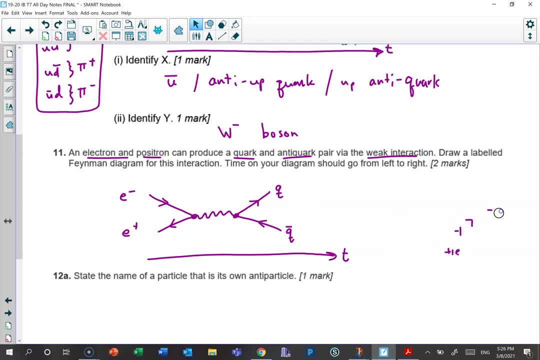 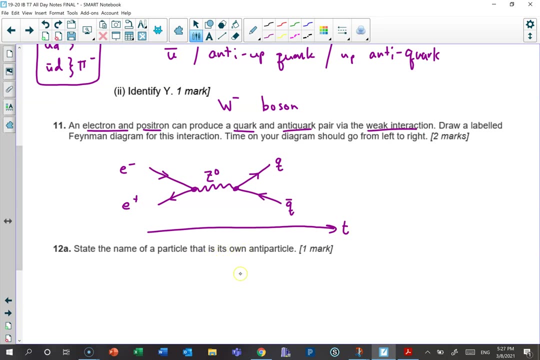 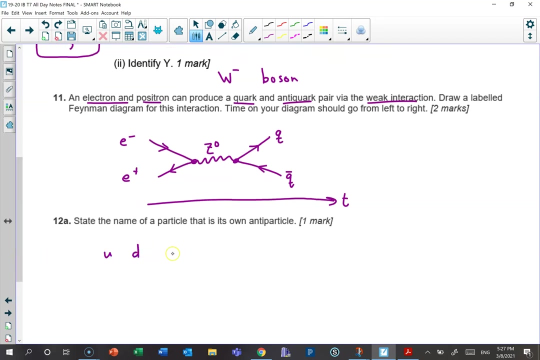 Just gotta remove that. Add my Z zero once more. Here we go, State the name of a particle that is: ooh, that is its own anti-particle, Ooh. What are all the particles you know Up down? top bottom charm strange: electron, muon, tauon, electron neutrino, muon neutrino, tau neutrino. those are all the particles, So one of them is the same as its anti-particle. What could it be? 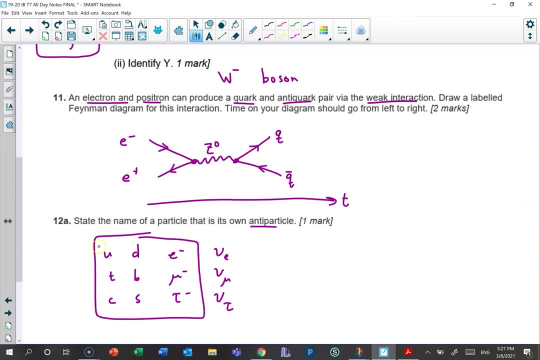 Well, look at all these. These all have electric charge, So the up is positive two-thirds. You probably see where I'm going with this, And so anti-up would be negative two-thirds. Those are not the same. This argument applies to top charm. 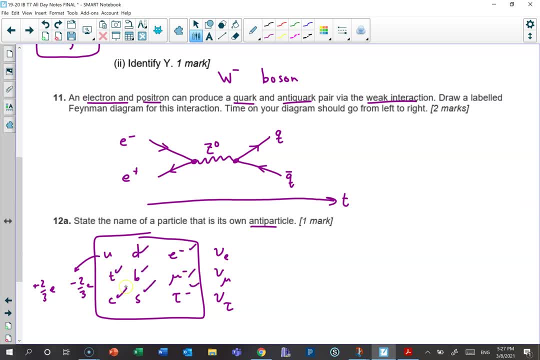 down bottom. strange, It applies to everything. They all have non-zero electric charge. But what about the neutrino? It has zero electric charge and basically zero mass. It's a tiny, tiny, tiny, tiny mass. Everything is zero for the neutrino. 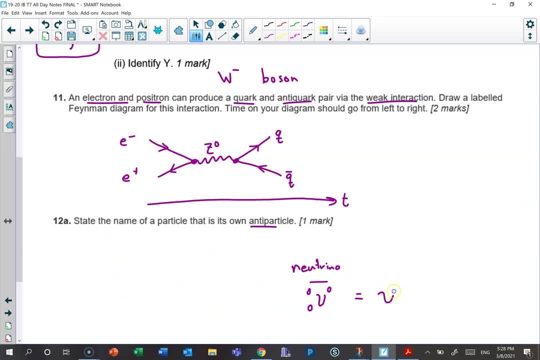 And so in fact, they think it may be its own anti-particle. All three types. that might be true. This may not be true. This is a bit speculative as a question. I don't think we know that with certainty just yet. 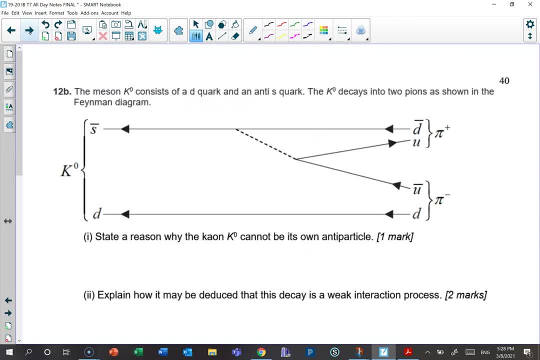 Anyway, 12b. The meson K0 consists of a down quark and anti-strange. K0 decays into two pions as shown in the Feynman diagram. Okay, Two pions. Vertex. There's a vertex. 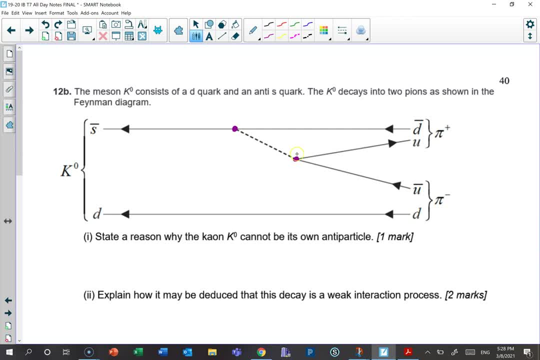 I like to put dots Okay State a reason why the kaon cannot be its own anti-particle. Why can't the kaon be its own anti-particle? They're saying, look, it's still neutral, isn't it? 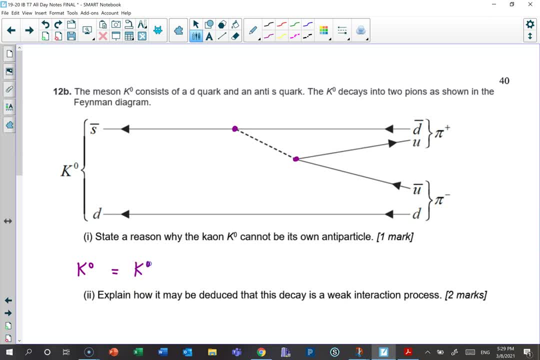 Whoops. If you make it an anti-particle, it's still electrically neutral, So they have the same charge. Why can't it be its own anti-particle? Well, if you look at the structures from which it is made. 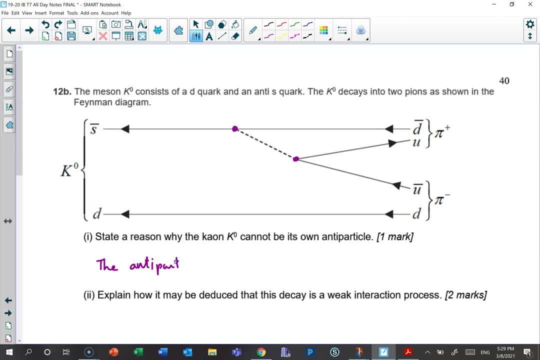 the anti-particle of K0 is strange and anti-down. So what's different? How is that different from anti-strange and down? For one? well, maybe the only difference: they do not have the same strangeness, Right, This, you would think the strangeness. 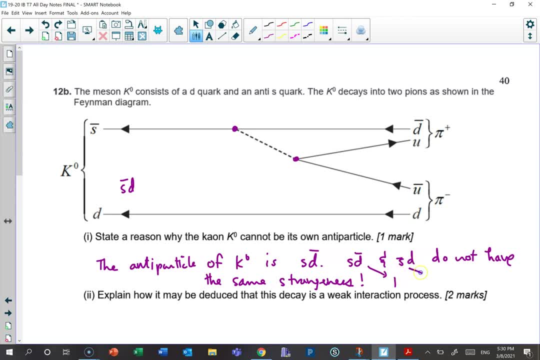 is positive one because there's one strange quirk And you would think the strangeness here is negative one because there's an anti-strange. But remember, when you're tallying up strangeness you do the opposite sign for both. The point is they're still not equal. 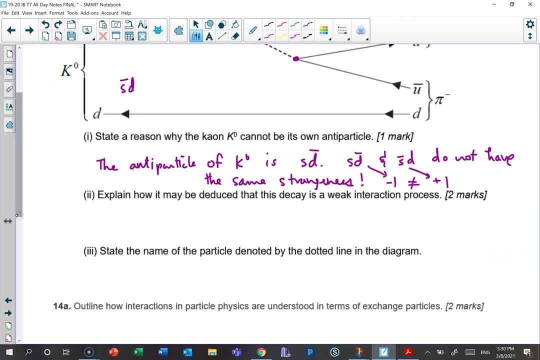 And that's a good reason why it can't be its own anti-particle. Different behavior when it comes to strangeness. Explain how it may be deduced that this decay is a weak interaction process. You see that and you think strangeness. 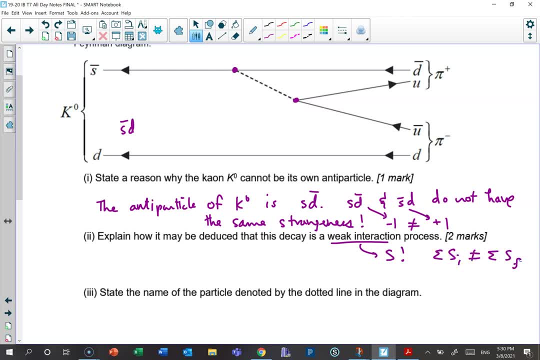 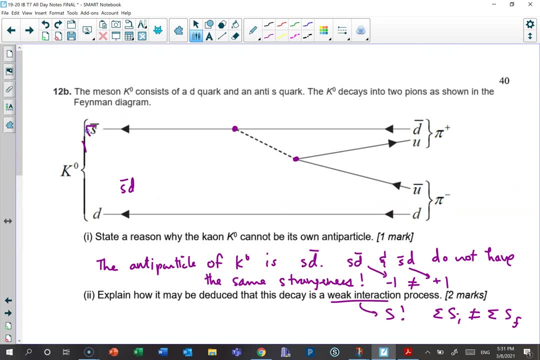 Is strangeness not conserved? Let's look and see if that's what they're asking about. Yeah, Look at the particles. initial You've got strange and down, initially anti-strange and down, pardon me. So the initial particles: 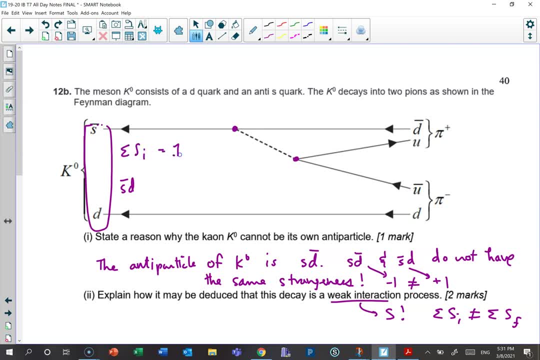 the strangeness is one you would think, oh, you would think it's negative one because it's anti-strange. But with strangeness, when you are tallying up the strangeness, you do the opposite sign Here at the end we have anti-down up. 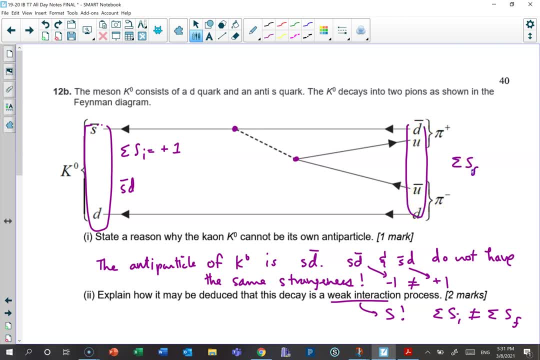 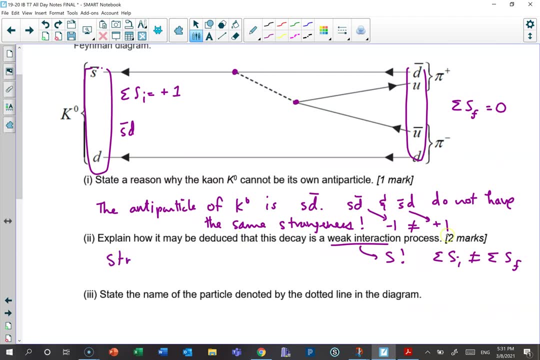 anti-up and down. There's no strangeness there at all, No strange or anti-strange quirks. Strangeness- look, it's two marks. So I would start by saying: explain that the strangeness initial is positive one. 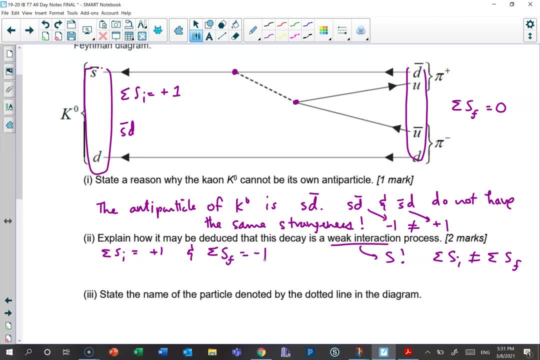 You don't want to just put symbols, You need to explain it. Whoa, the strangeness? final is zero, because there are no. you know like? write it out with words: Strangeness is not conserved. Positive one does not equal zero. 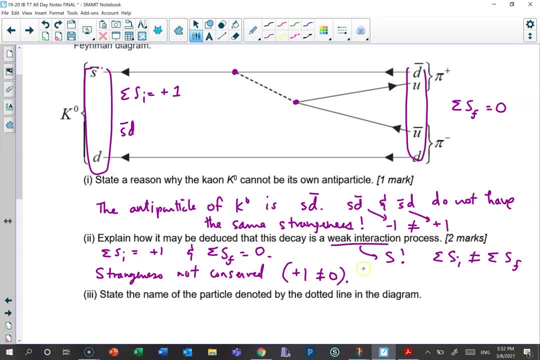 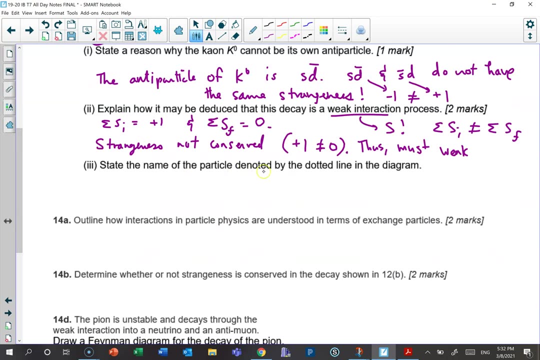 That much I know. Therefore, it must be a weak interaction. The weak interaction is the only one that can break the strangeness. conservation law State the name of the particle denoted by the dotted line. All right, should we just look for charge? 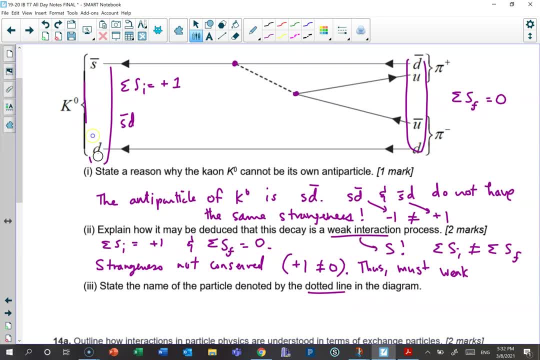 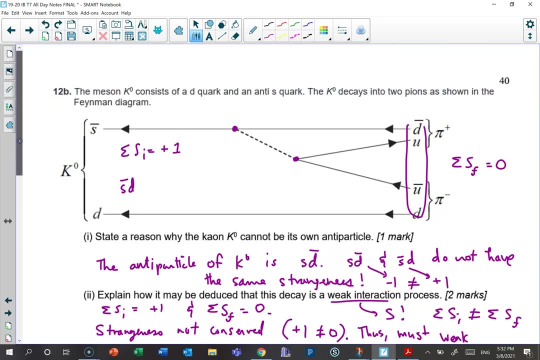 I mean you know it's. if it's changing the strangeness, then you know it's going to be one of the particles for the weak force. It's either W plus, the W minus or the Z boson. How do I know that? 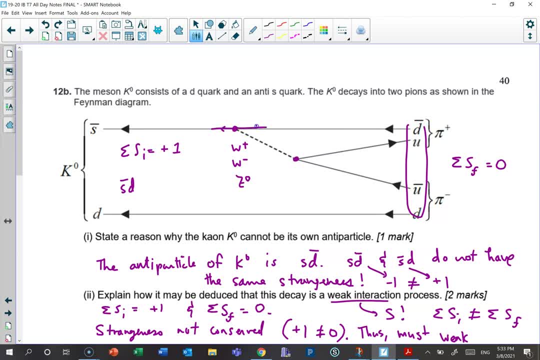 Because the strangeness going in is positive one and the strangeness going out is zero. It's this weak interaction. It's got to be All right. so let's look at charge then Anti-strange. do you have those memorized yet? 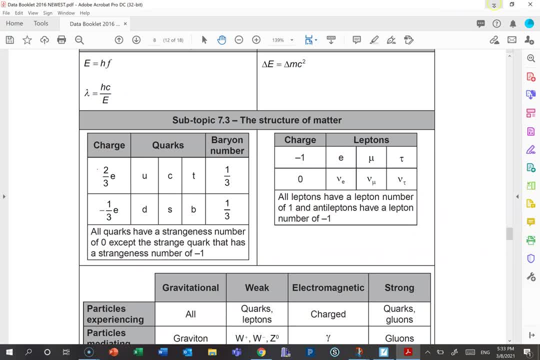 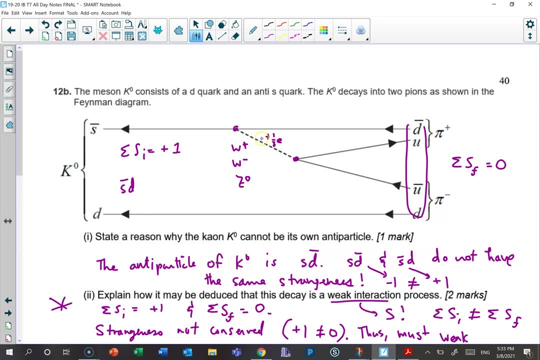 It's going to be not negative one-third but positive because it's antimatter. So that's the total charge entering. oh, wait, wait, wait, I'm in the wrong spot: Positive one-third going in. Let me take out that other vertex. 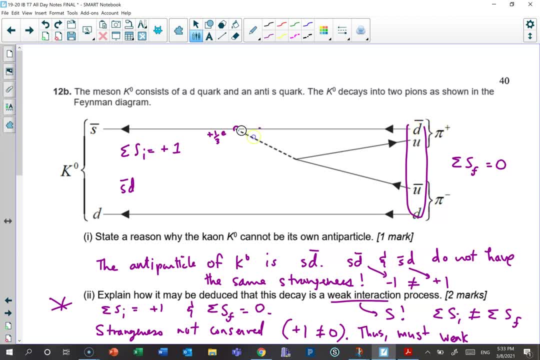 And exiting anti-down. if you look back, regular down is minus one-third, so anti-down is positive one-third. Okay, And so what does this virtual particle have to have for its charge Zero, Because the total charge going in is positive one-third. 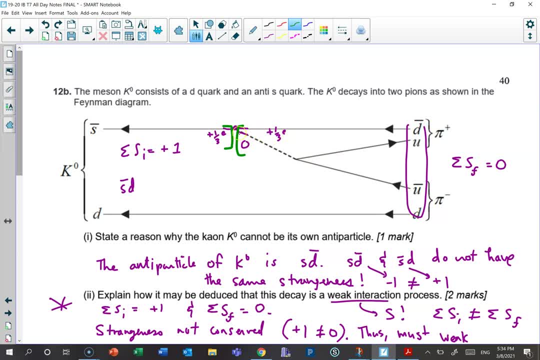 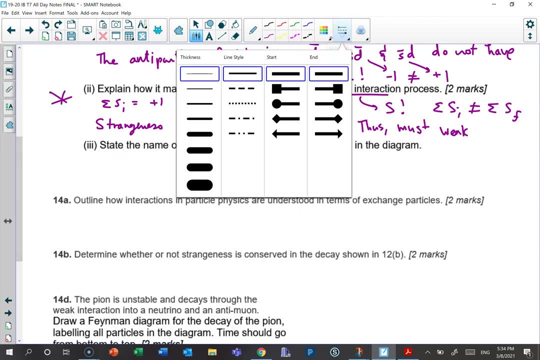 and the total charge exiting that vertex has to also be positive one-third, And you already have your positive one-third from the anti-down. So this must be the neutral. let me go down there. It's got to be the neutral force particle of the weak force. 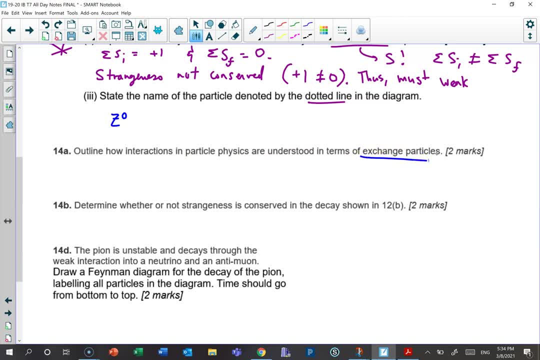 Outline how interactions in particle physics are understood in terms of exchange particles. Okay, So what are they looking for? Exchange particles are virtual, virtual, non-real particles. Is that what they want? You could say they're a quantum of energy in a field. 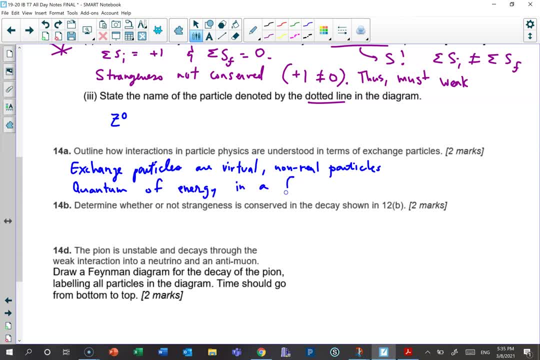 Okay, In a force field You could say: we use them, You probably, you definitely want to say they mediate or carry the force between two real particles. Those are all good things to put in If you want to get really deep. 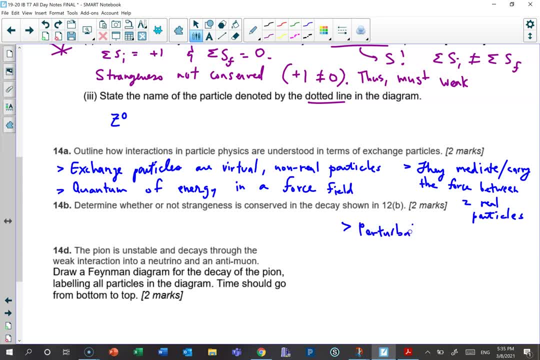 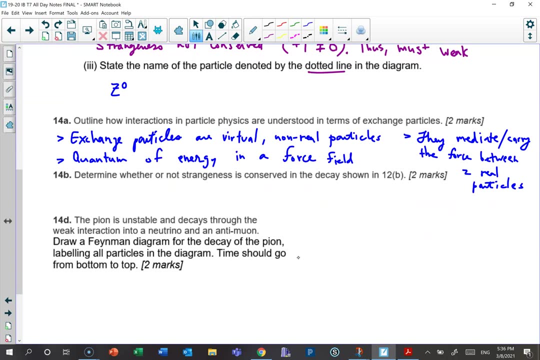 say: mention perturbation theory. Go look that up. Go look up the PBS Space Time video on virtual particles. That will tell you so much more than anything else you could learn. Don't mention perturbation theory, You won't get points. 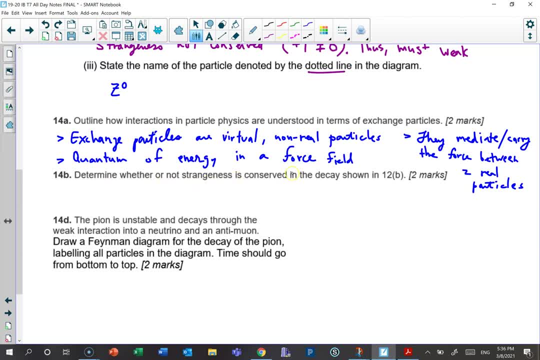 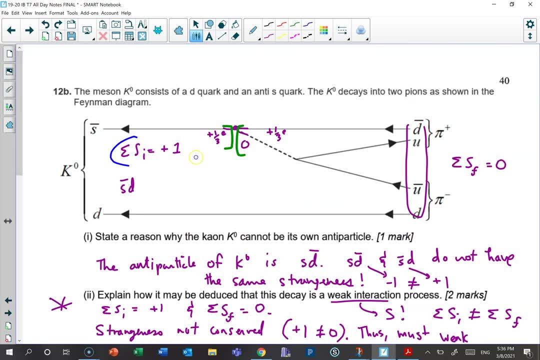 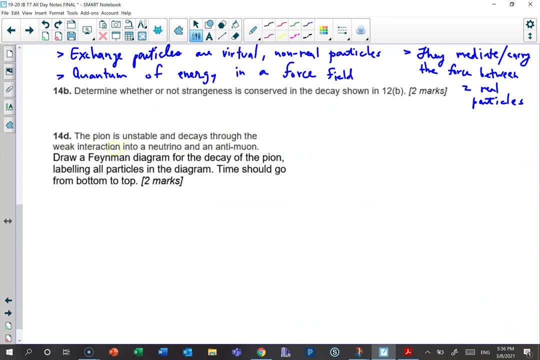 Even though you'd be right, Determine whether or not strangeness is conserved. Okay, Kind of getting bored of strangeness. No, it's not. We already talked about that, So I'm not even going to write it down. The pion is unstable and decays. 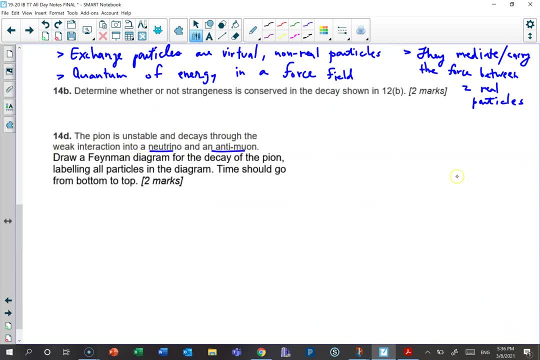 through weak interaction into a neutrino and anti-muon. Ooh, this is fun Neutrino, so let's write that. Let's just say: pion Which pion, Positive neutrino and anti-muon Which is the positive muon. 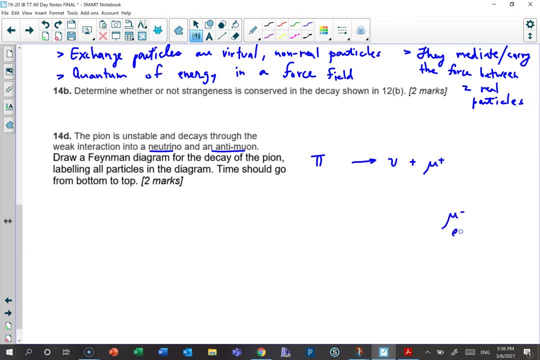 because the muon, you might recall, is just the same as an electron, but heavier. So what's the antimatter particle? The positron and the muon, which is just the positive version. That's how you know to write it this way. 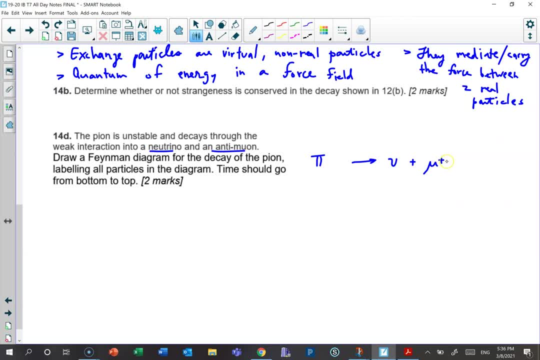 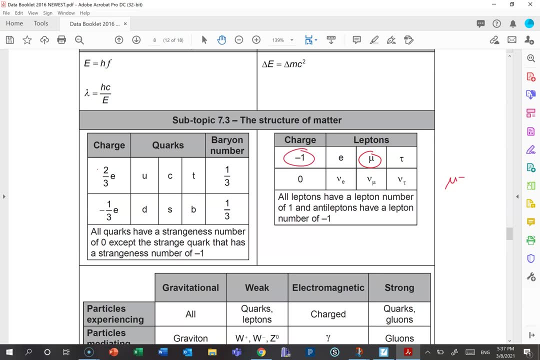 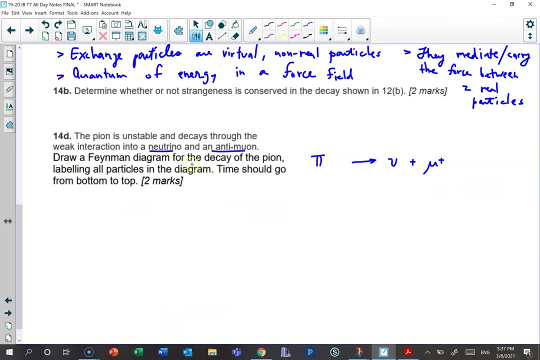 and not like this. That's also how you know it has positive charge. But you could look at your data booklet: Right Muon: negative one. So the anti-muon would be positive one. Hooray, Okay, Draw a Feynman diagram. 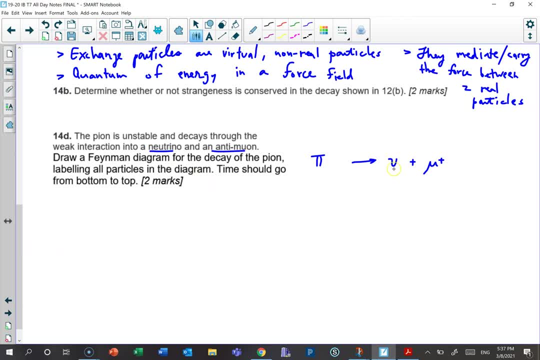 for the decay of the pion, labeling all parts of the diagram. So this has no charge, Right? This has charge of positive one. So what's this got to be Positive one, And so what's the quark composition of a positive? 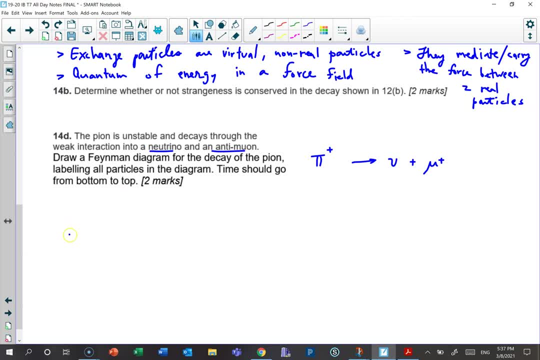 pion: Positive pion. What are the pions? It's this, this, this or this, Oops, And if you look at the charges, that's the one that has positive one as its charge, Up and anti-down. 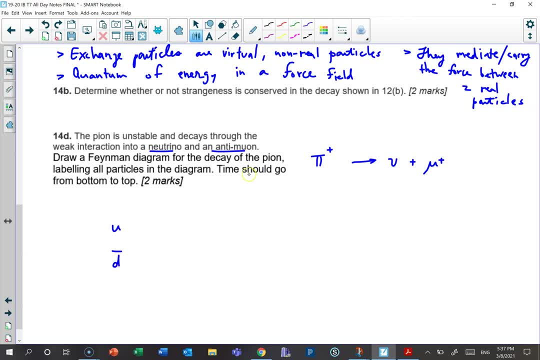 So I'm going to write up and anti-down. Uh oh, time should go from top to bottom. Up and anti-down. What do mesons do? They decay. They annihilate themselves. So you generally want to start out if you have a meson. 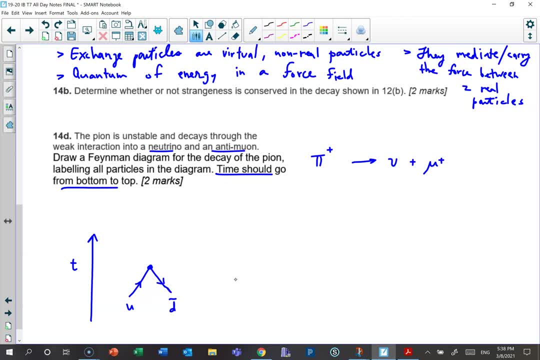 try to annihilate it. This is kind of fun stuff. This is fun to talk this way, And so when they annihilate, there's going to be a weak interaction. You can use not a z particle, pardon me, If you look at the charge. 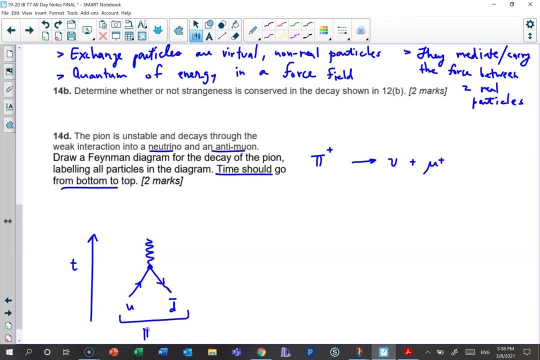 this is positive one. This is the pion, so its charge is positive one. So this has to carry that positive charge away. If you balance the electric charge at the vertex there down below, Balance the charge here, This is W positive. 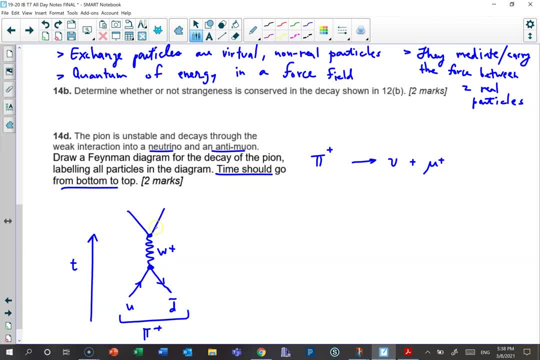 And can you do pair production after that? This and this? Here's our anti-muon, Because it's anti-matter, it goes against time, It's a neutrino And it's not an electron neutrino, It's a muon neutrino. 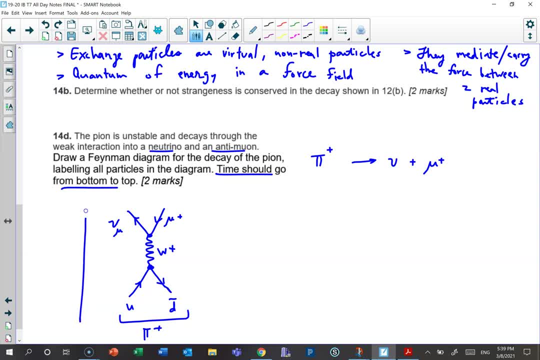 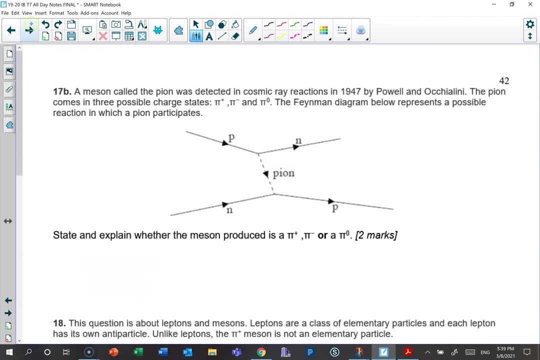 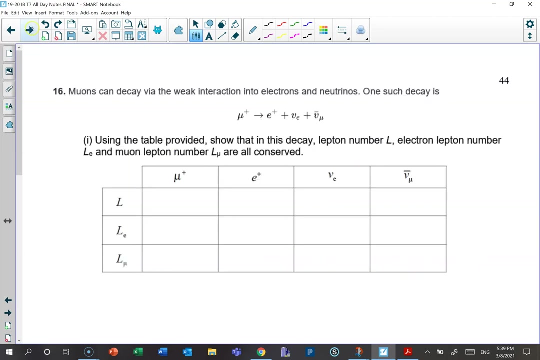 Because that's what it was created with. And we're done. Is this a composite particle? No, Nope, Okay, How many more are there? I was going to do all these. Good, I don't need to do that, Okay, I'll just do. 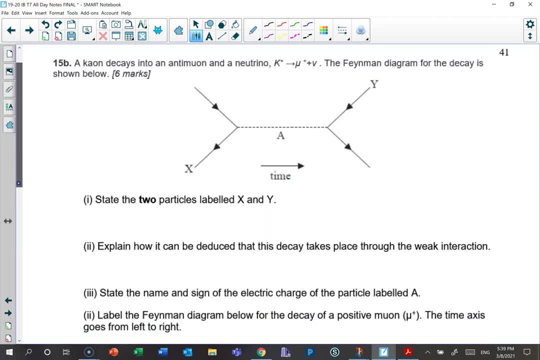 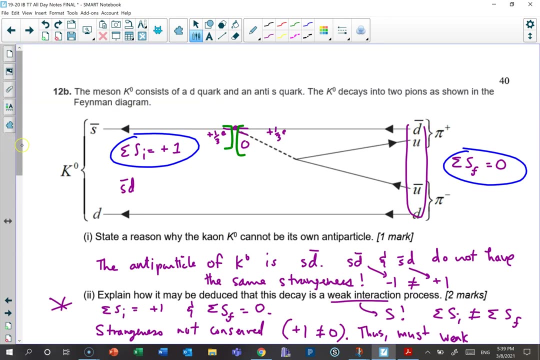 the last two. A pion decays into an anti-muon and a neutrino State. the two particles labeled X and Y, Ooh, How are you supposed to know what a pion is? That's part B, Did they tell us in part A? 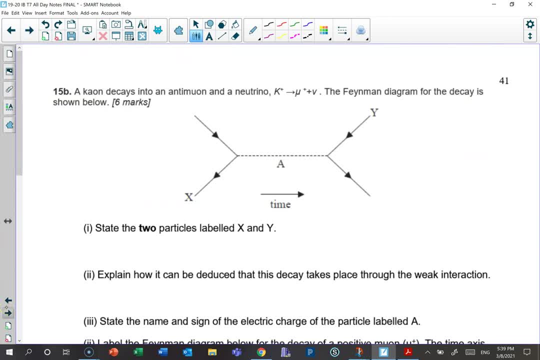 Uh-oh, uh-oh. Well, hang on, let's see if we can figure it out. I don't think we can. I don't think we need to know what the pion is, But Y is def- like look at what's here at the end. 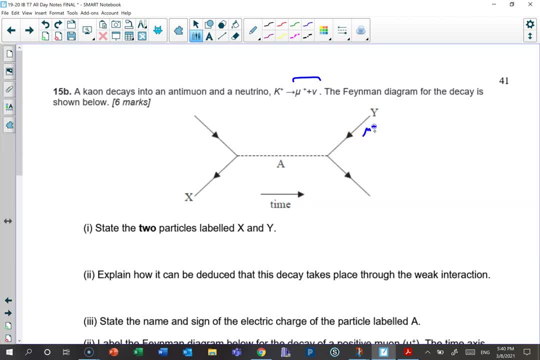 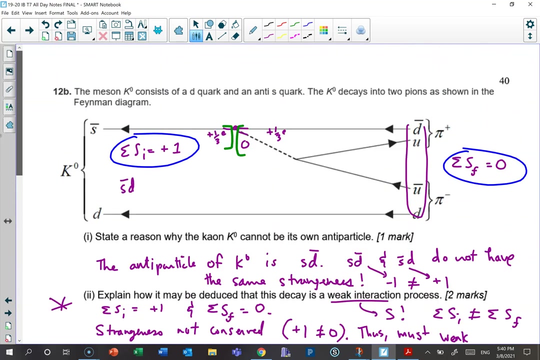 Y has got to be the anti-muon And this is going to be the neutrino, A muon neutrino. And let's look up what a pion is. Are we supposed to know that? Was that given? There must be a part A. 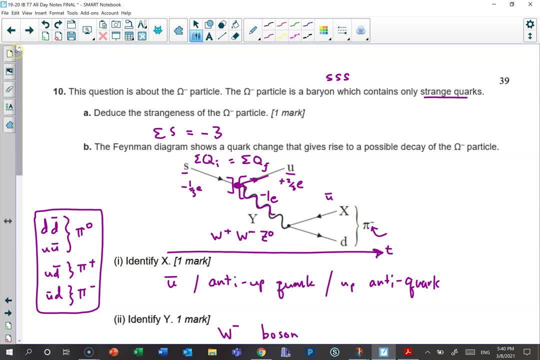 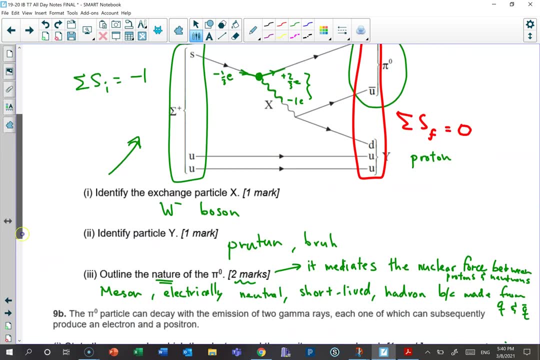 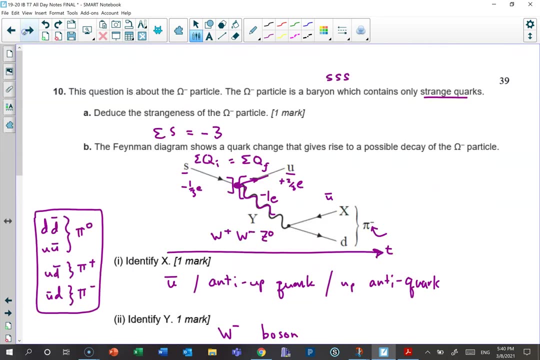 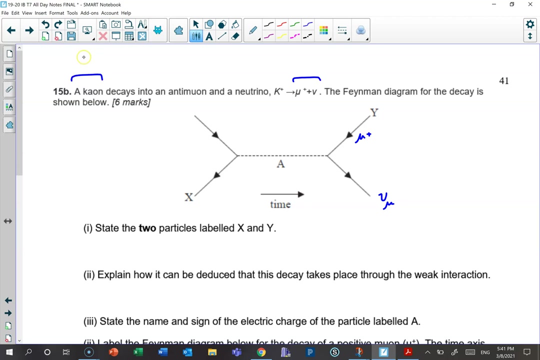 that we missed. Did it say earlier What's the kaon? We'll find it somewhere in our notes Up and anti-strange, We don't need to know that. We're supposed to have memorized. So the kaon I bet they said earlier in the problem. 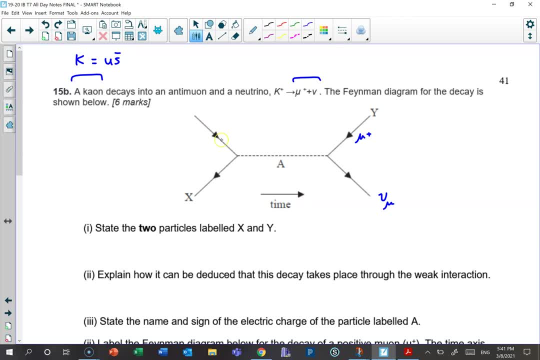 I bet they said this, And so now you need to realize that's pointing with time, That's the up quark, This is against time, So that's the anti-matter. So X is an anti-strange quark And Y. 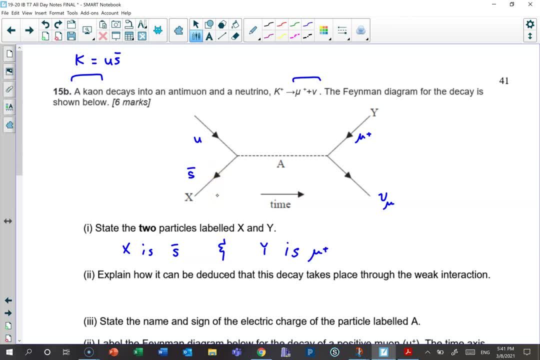 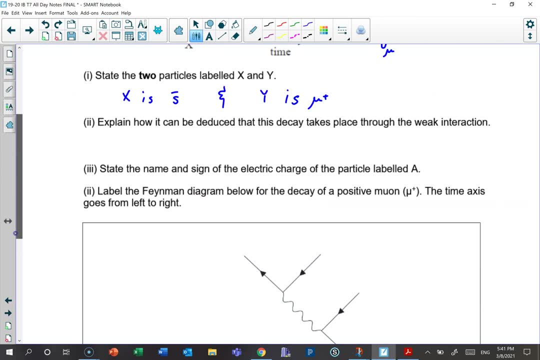 Yeah, that's what they're testing here. That's where the zero is pointing. And do you remember that this anti-muon is anti-matter? Explain how it can be do. Okay, we've done this problem like 15 times. 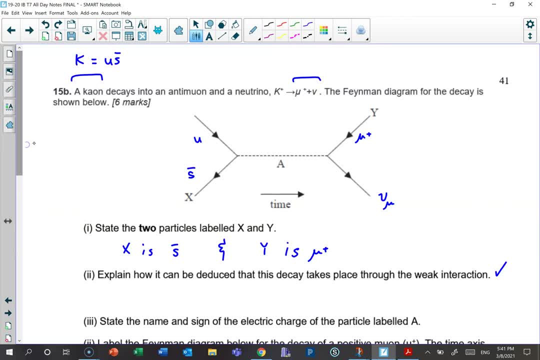 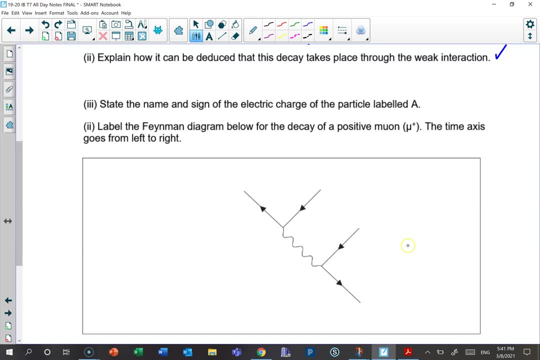 Feels like the only thing we've been answering You. look at strangeness, Yep, strangeness State the name and sign of the electric charge of the particle labeled A. Okay, Which particle is A? It's the exchange particle, The virtual particle. 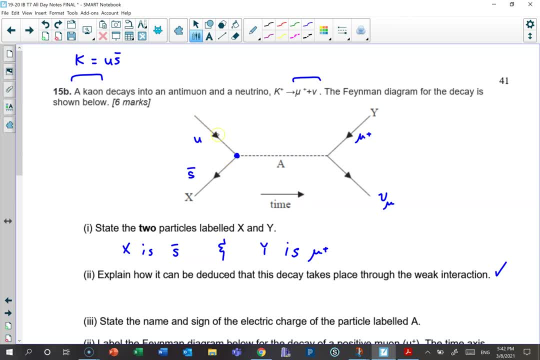 We know it's the weak force. So, by the way, just in case you're skipping ahead, this is what you do as you say: the sum, the total strangeness. initial, like: look at the very, very, very, very beginning. look at this part of these two particles. 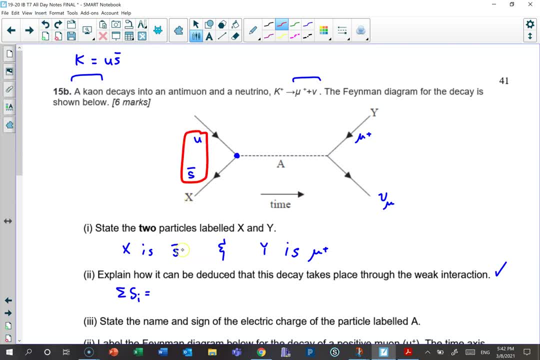 up and anti-strange, aka as the kaon The strangeness, you would think it's negative one because it's anti-matter, so anti-strange should be negative, right? Well, for strangeness, we do the opposite. What's the strangeness at the end? 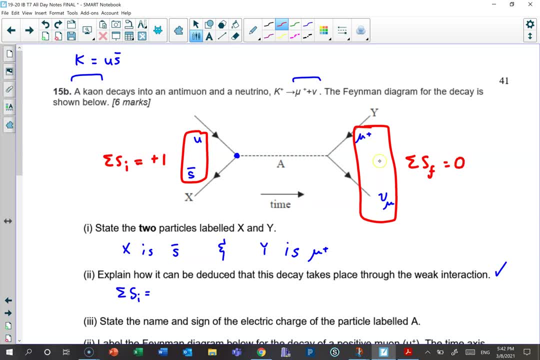 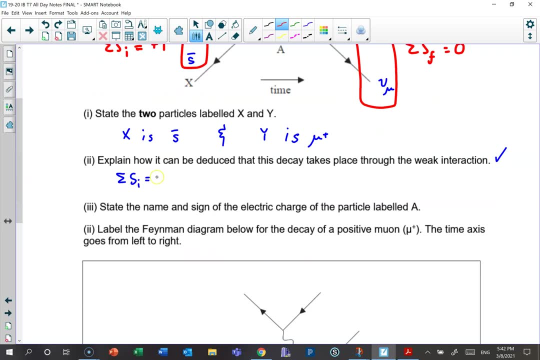 Zero Because there are no strange particles. and so when you count strange and anti-strange, there are none. And the only way to change- and so you say that, you explain that, you say it in words- the strangeness initially is zero. the strangeness at the end is: 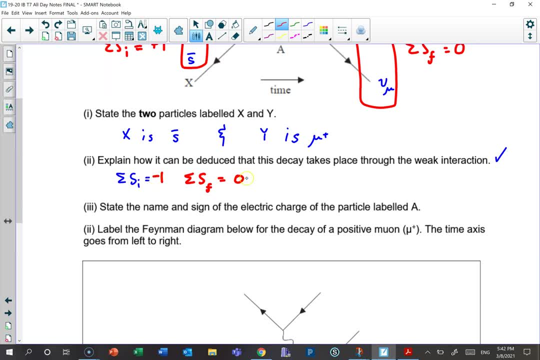 oops at the end is zero, at the beginning is negative. one strangeness cannot be. it must be conserved. strangeness is conserved. strangeness is conserved except except in weak interactions. that's how we know. that's how we know. state the name. 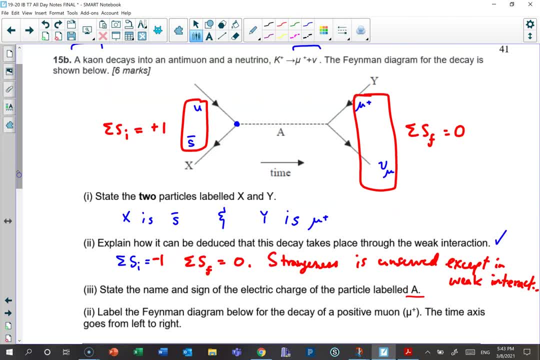 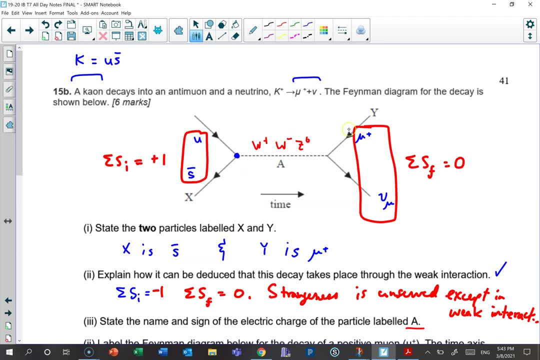 and charge, yes, of the particle labeled A. so because it's the weak interaction we know it's either the W plus boson W minus or the Z. the only difference is the electric charge. so balanced charge. I will choose this vertex. the up quark has a charge of positive. 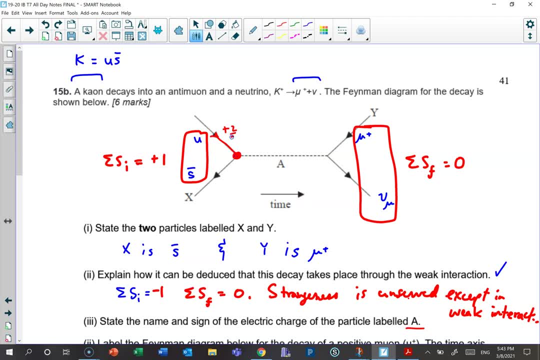 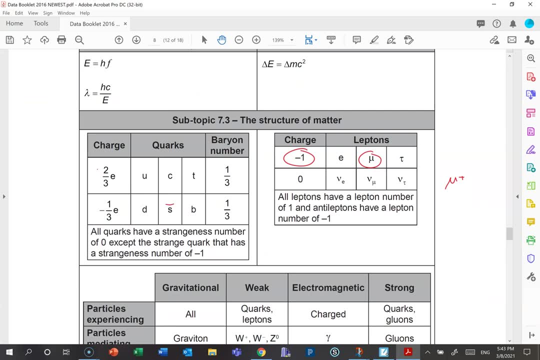 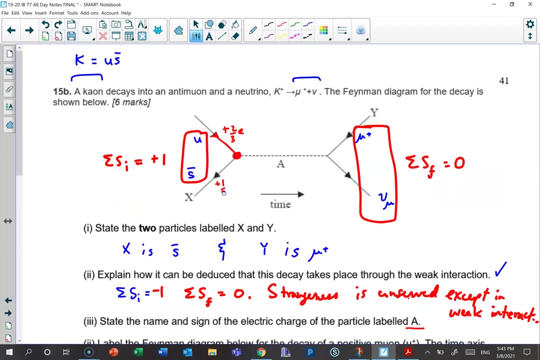 two thirds. and if you don't believe me, go check your data booklet. strange is negative one third. so anti-strange would be positive one third. I shouldn't write in my data booklet and then, if you add the total charge entering that vertex, that particle and that particle. 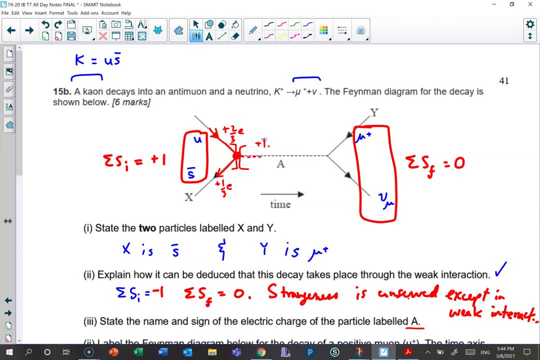 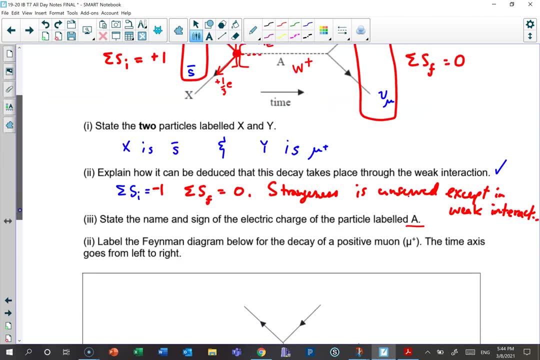 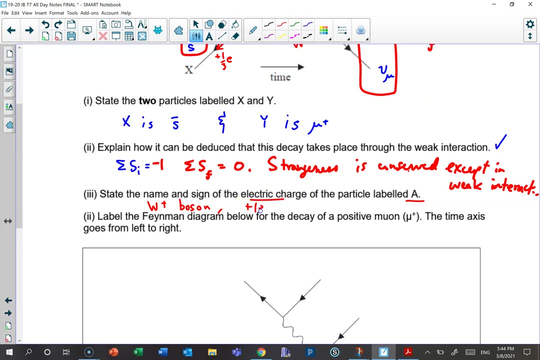 they add to positive one. so what's the total charge exiting the vertex? positive one. this has to be a positive a W plus boson, it's the electric charge, E, don't forget the E. another way to put that would be positive one point six times ten to the minus nineteen. 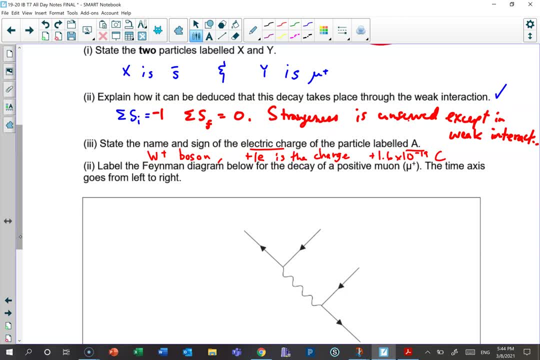 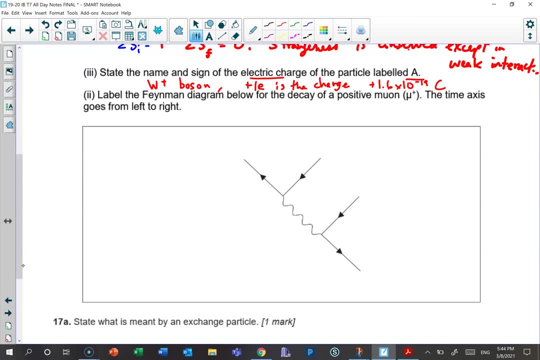 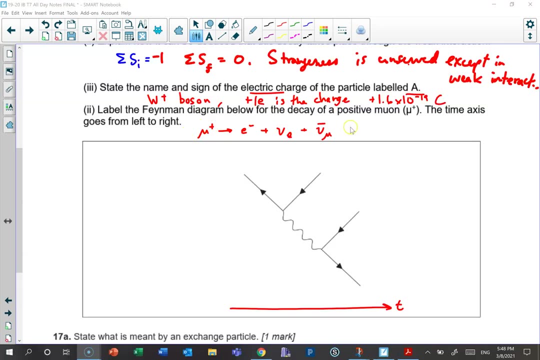 we're always dealing with the elementary charge here for these problems. ok, label the Feynman diagram for the decay of a positive muon. the time axis goes from left to right and this equation was missing so I've had to add it here. you should be given that equation. 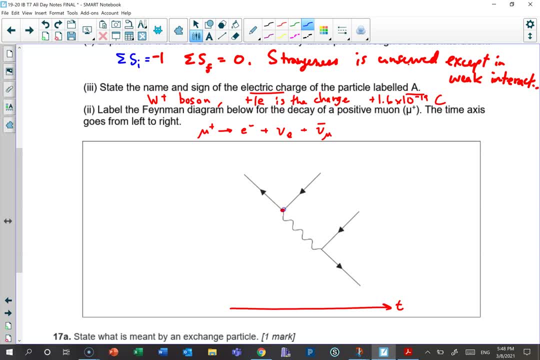 so, left to right, the very first particle is this one. it goes against time, so it's anti-matter. what is that particle? that's what we start with: the anti-muon, and so now we have to create right here. the anti-muon emits this exchange particle. 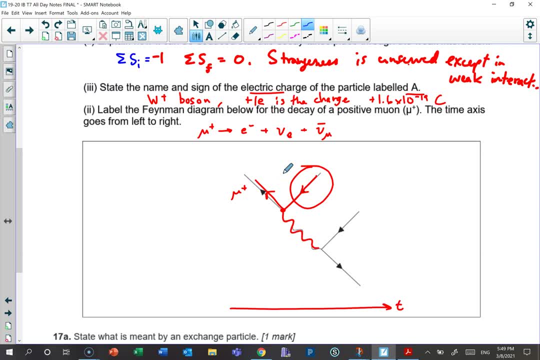 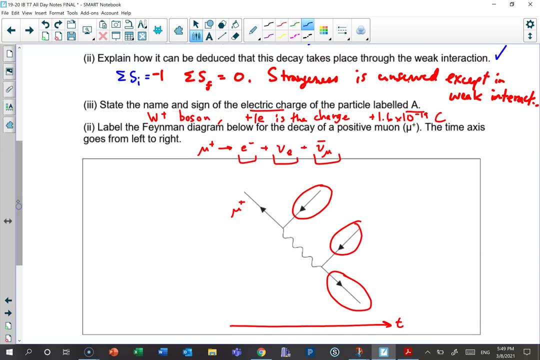 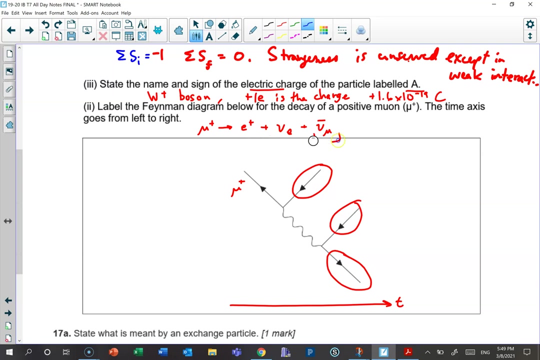 and it turns into something new. now notice the final this and this. these are the three final products, and when I wrote this- this is incorrect, that's what it should say- I miswrote down. I recorded that by looking it up online and I wrote down the wrong thing. 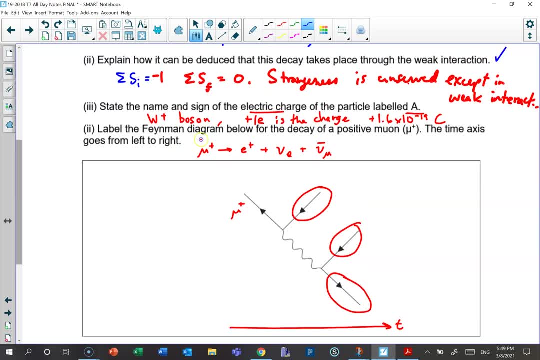 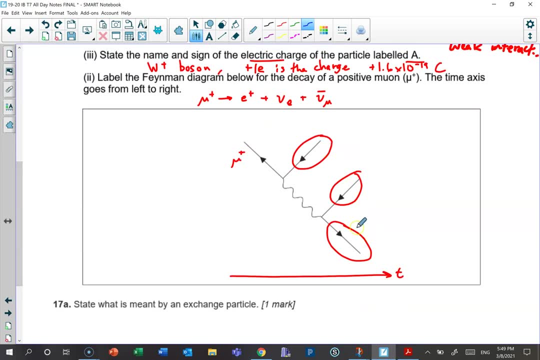 but I've corrected it now. so this again at the start of the problem. ok, so here are the three final products. notice only one points with time, so only one is matter. which one is this? look at the three. it's got to be the electron neutrino. that's the only matter. 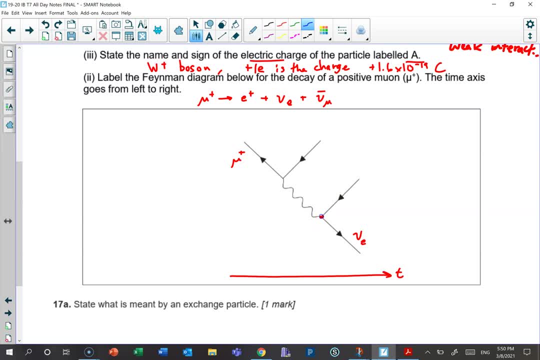 particle at the end, if you think about, ok, the electron. so this right here is either the anti-muon or it's the anti-electron, and if you're deciding between the two, you should be reminded of the fact that these guys are often produced together, not always. 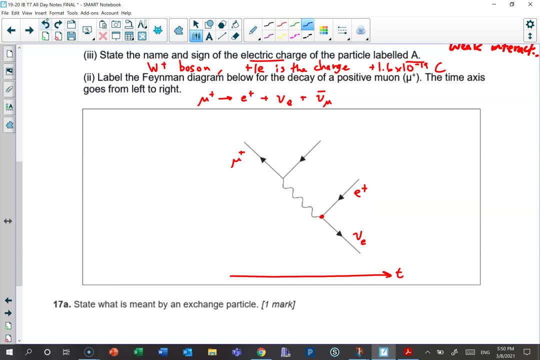 but often so. the reason for that is if you look at the total lepton number going into the vertex, it's zero. and remember, when you count leptons you have to stay within one of the families. so stay within the electron family or the muon family or whatever. 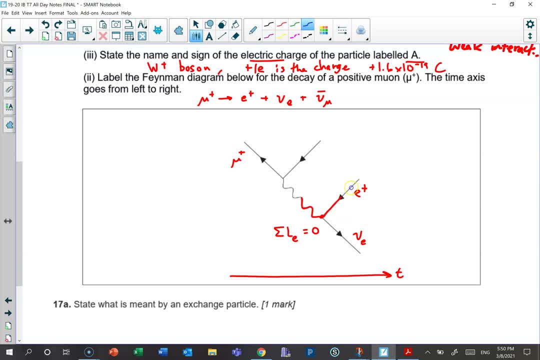 so that's the total lepton number going in. if you count how many electron style leptons there are at the end, this counts for positive one because it's a lepton. it's matter. this anti-electron is an anti-lepton, so it adds to zero. 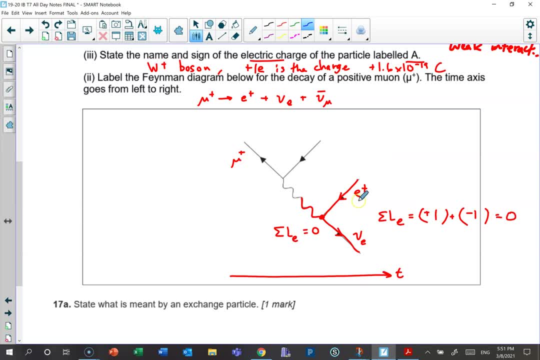 so you need the positron right there. if you had put the other one, the anti-muon, if you had put this there instead, it does not count as part of the electron family, so now you would have violation. this can't work, because zero does not equal positive one. 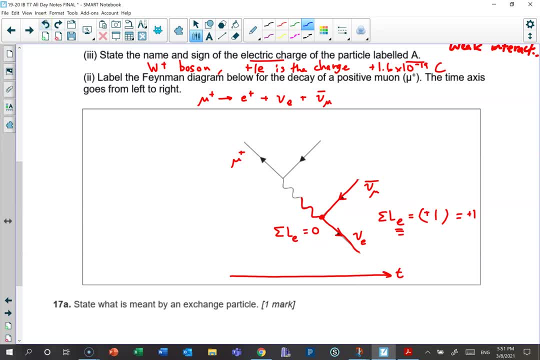 this would violate conservation of lepton number within the electron family, and so we have to have right there the anti-electron. that leaves right here the anti-muon, and if you think about, if you think about this vertex here you've got initially going into the vertex. 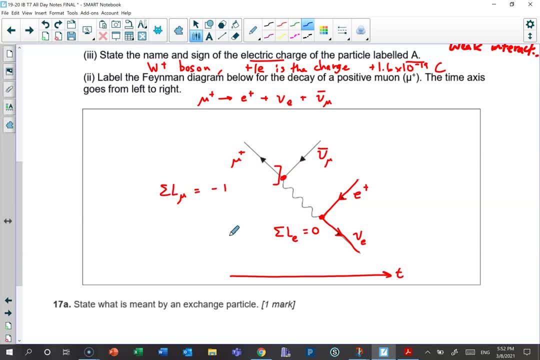 how many muon style leptons are there? there's negative one, because it's anti-matter and then leaving the vertex exiting. how many muon style leptons are there? remember, the leptons are just the neutrinos and you know, like the muon or the electron. 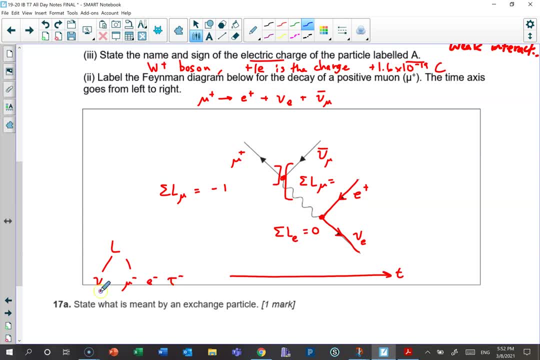 the tauon. those are the leptons, and each one has it's own neutrino. so in that case, the total at the end would be: this is a lepton. yes, it's in the muon family and it counts as negative one because it's anti-matter. 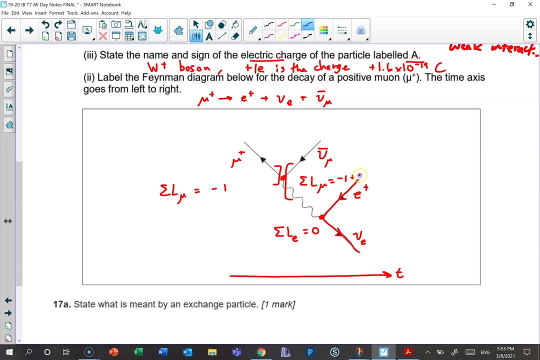 this squiggly exchange particle is not a lepton, so it's plus zero and the initial equals the final. now the final thing we need to do is label the force particle the exchange particle, and so if you look at this vertex, you know, maybe it's easy. 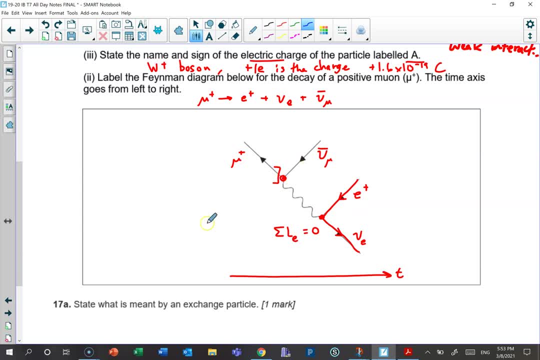 yeah, this is a fine vertex. the total charge going in is positive one, and so the total charge exiting that vertex must be equal. it must be positive one, which means this is a W positive boson, because that one right there has no electric charge, so you need your positive one. 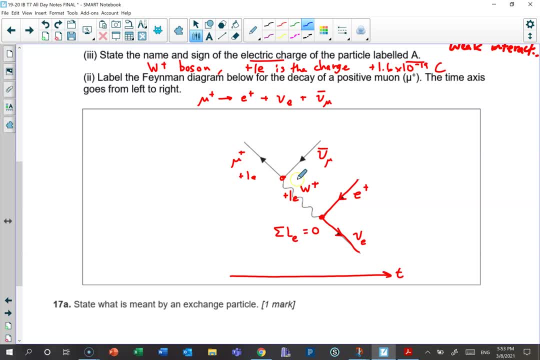 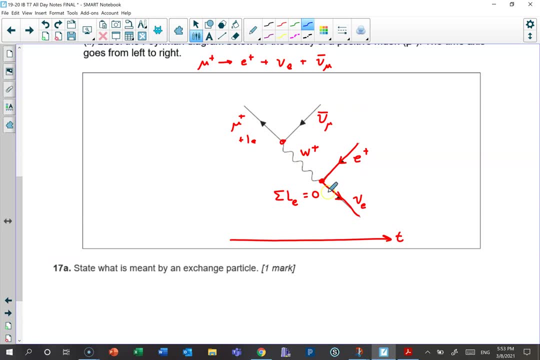 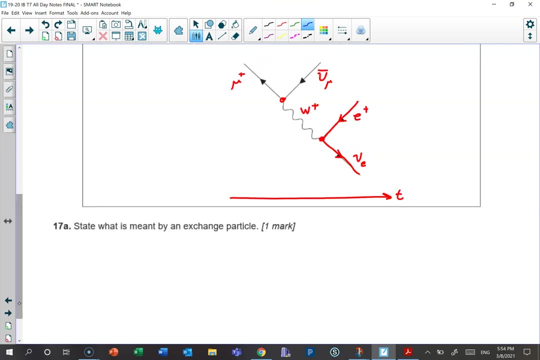 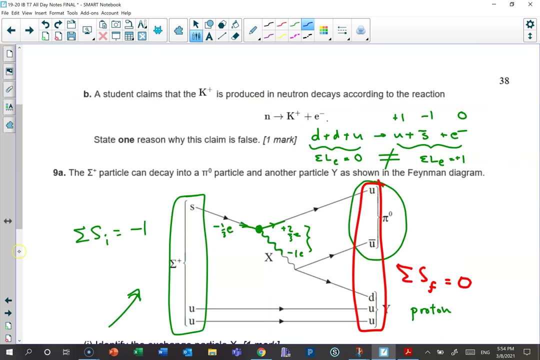 electric charge to be carried off by the boson. so that's our labeled diagram. there you go. state what's meant by an exchange particle. we've already answered that. there's a lot of things you can say. we had a really fun answer. that was like better than what I'd be. 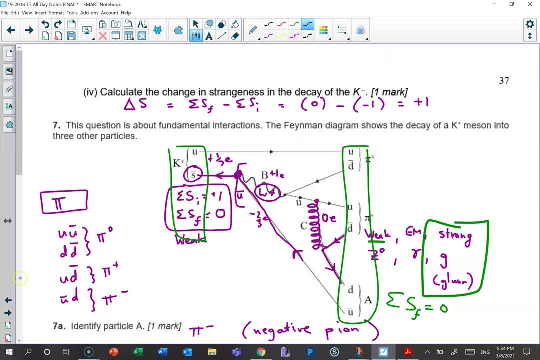 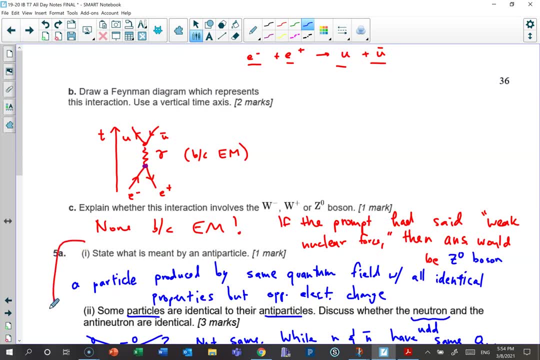 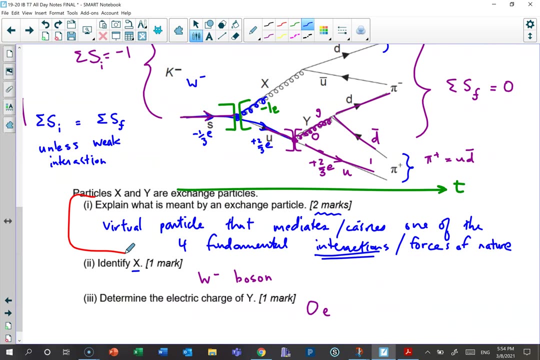 would expect. where was that fun answer? yes, no, not that. that's antiparticle. yeah, here it is, there it is um now, now, this is actually not perfect. it should say a particle that is not real but mediates or carries one of the four fundamental interactions. 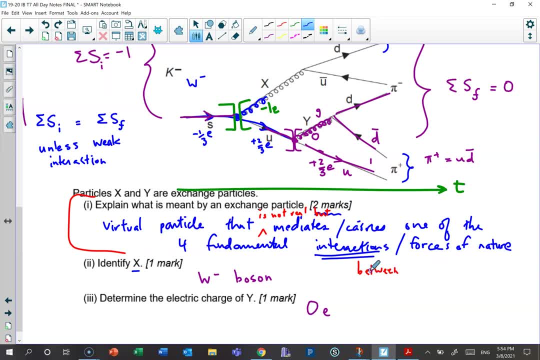 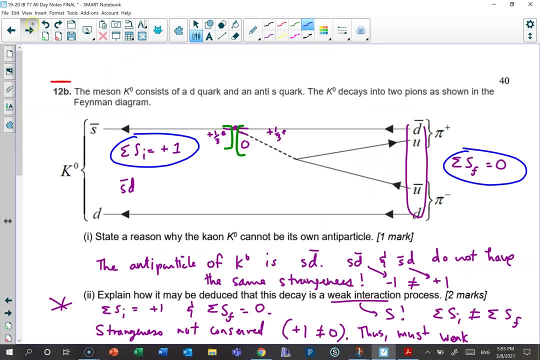 or forces of nature, between two real particles. it doesn't have to be just two, it could be more than two, but we model it typically just between two particles at a time. yep, exchange particles aren't real. that's weird. yeah, they're. they're more just mathematical tricks. 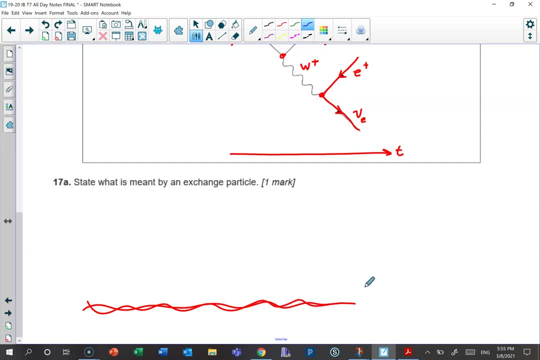 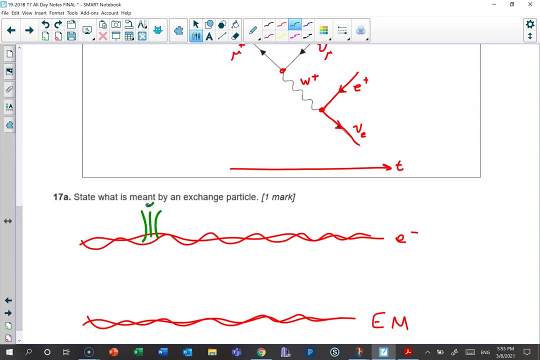 remember they're like here, like you've got, here's um the electromagnetic field, here's the electron field, literally that produces electrons and anti-electrons. and remember you've got like, okay, so here's an electron, it's an excitation or vibration in the electron quantum field. 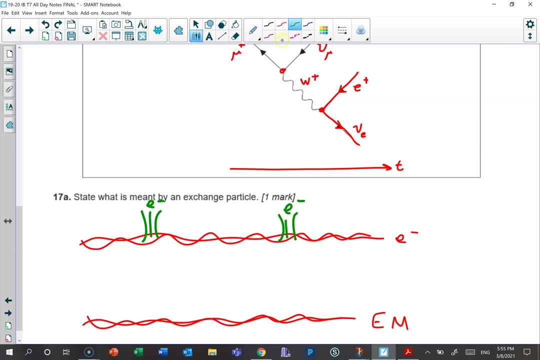 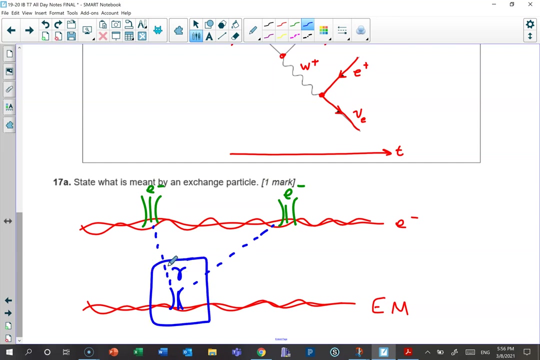 here's another electron, and the way they interact with each other is by interacting with a vibration in the electromagnetic field, which then interacts with that one. that's how we model this interaction. so exchange particles are virtual particles, they're force particles. they're not real, but they mediate the force. 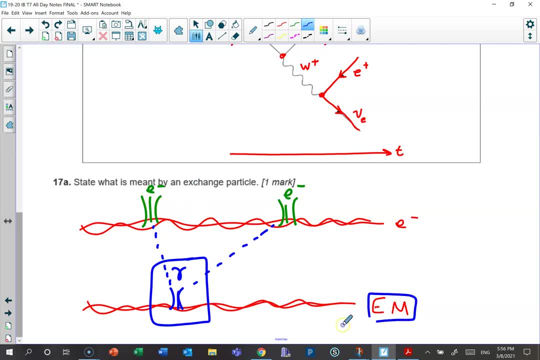 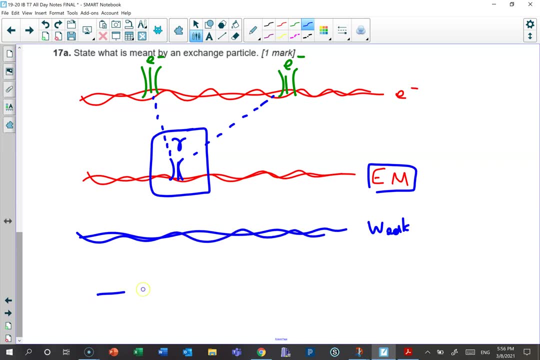 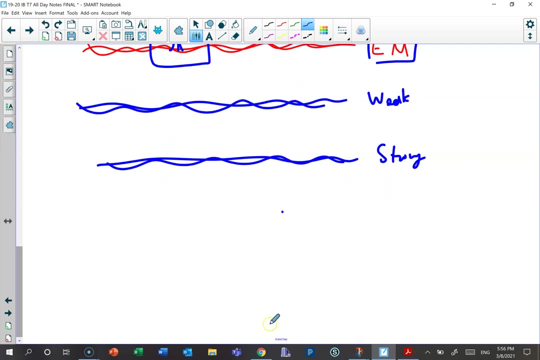 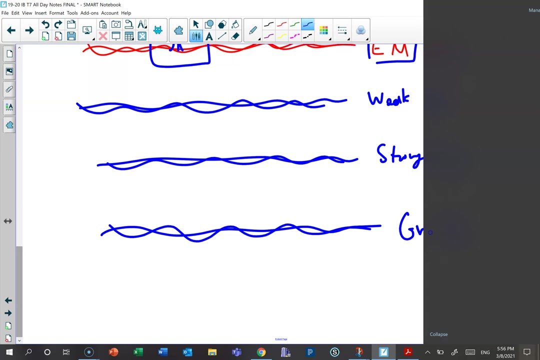 between two real particles. one of the four fundamental forces, em is one, the weak nuclear force is another- I should be using different pen colors. the strong nuclear force is another and the gravitational force is the last. of course, you remember I've said this many times: gravity does not. 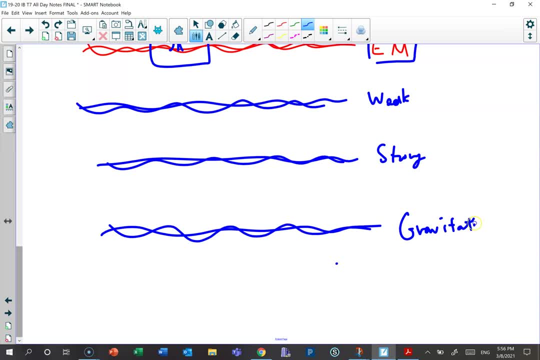 we do not actually know how that part works. whoops, we do not have a working model that is confirmed for quantum gravity, for force particles like the graviton. we've never seen that particle, ever so we don't know yet for sure what it's like, how it exists. 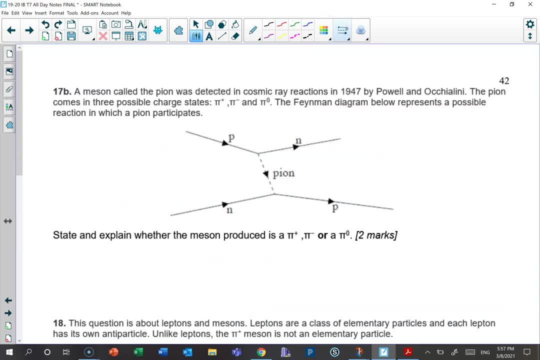 whether it exists. finally, last one: a meson called the pion was detected in cosmic rays. blah blah blah, it is cool, this is good, not blah blah blah, it's fun. the pion comes in three possible charge states. we've learned that. here is a reaction. 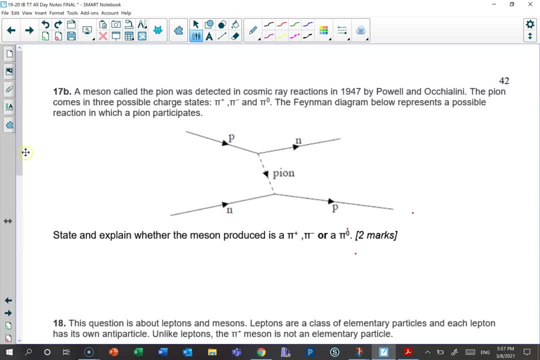 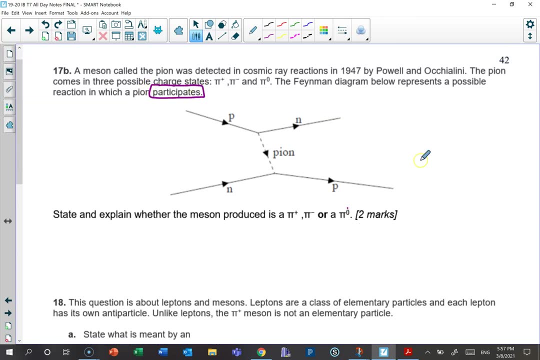 in which the pion participates. what a fun way to talk about these interactions. it participates in this interaction. kind of fun. so, yes, this is good. remember how we said: every fundamental force is really just a field, a force field. think about particles popping out vibrations in those fields. 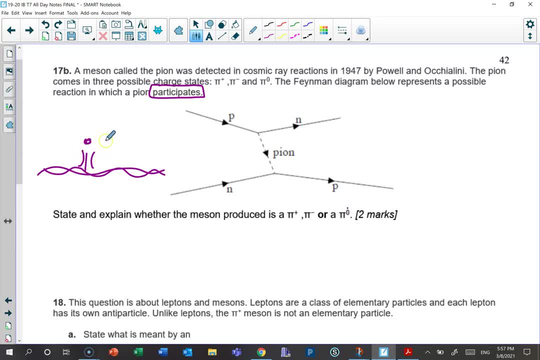 those force fields are particles and those particles particle-ish. that's what mediates the force. so well, hang on if particles mediate forces. when I push on my car to try and get it moving because it's out of gas or whatever, I'm not going to be very successful. 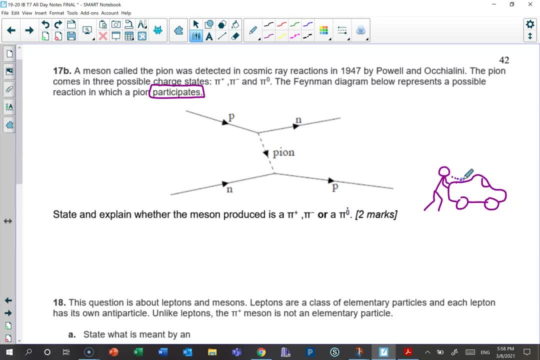 can I pretend that I'm exchanging particles with the car back and forth and that's what creates my applied force? does that work? no, there is a limit on how far this is going to go and how long will it be useful. there's going to be a limit. 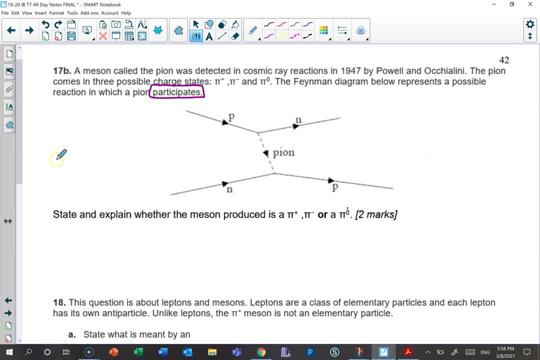 on how useful it is. but that limit does not stop with individual quarks. yes, when two quarks interact, they exchange force particles. but remember what the proton and electron are. here's a proton. it's proton bruh. here's the nu. not did I say electron. 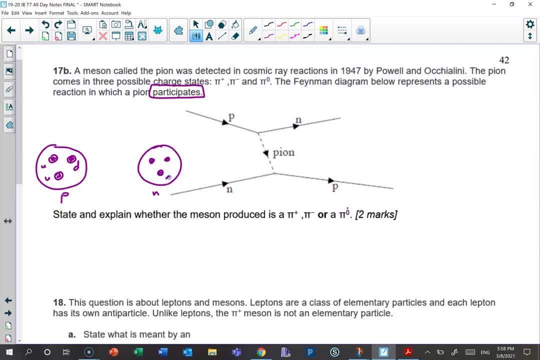 proton and neutron is what I meant to say. the neutron is two downs and an up and no, I can't pretend that my force on the car is happening via exchange particles. but these two baryons, these two composite particles, you can pretend they are exchanging mesons. 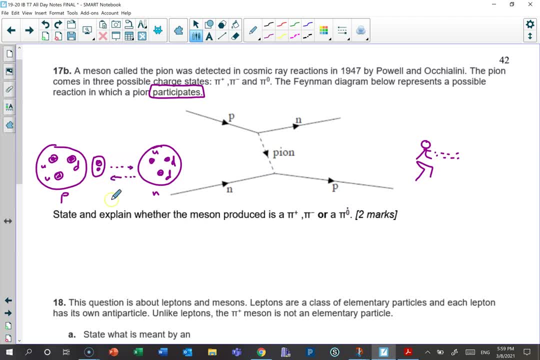 back and forth. in particular, they exchange pi mesons and that's one of the ways to model this long range force. longer, well, it's still short range. I shouldn't say long range, but this is the nuclear force. it's the only one we knew about. we didn't know. 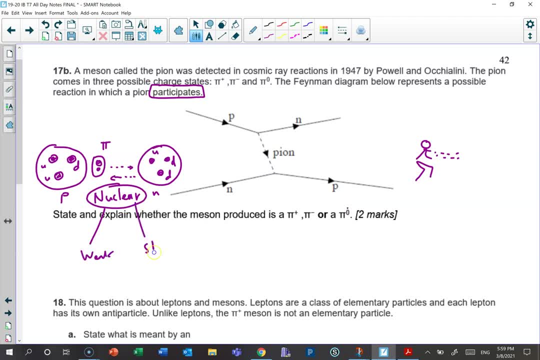 that there was actually a weak nuclear force and a strong nuclear force. that didn't come until later. we only realized. initially we thought there was just one force in the nucleus, the nuclear force, and so that nuclear force is really kind of outdated. it's really more of like: 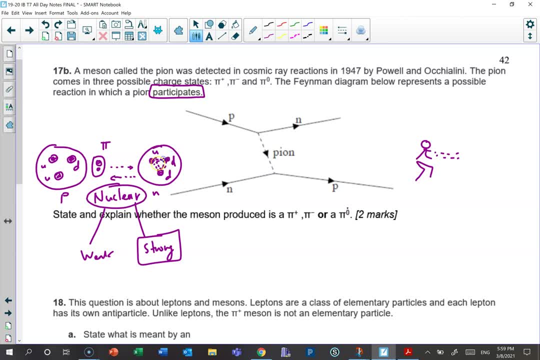 it's the strong force. these things are exchanging via the strong force, and they're exchanging gluons like mad. there's so much interaction and a little bit of interaction leaks out from one proton to its neighboring neutron. that's the idea, and vice versa. so that's what they're trying to tell you here. 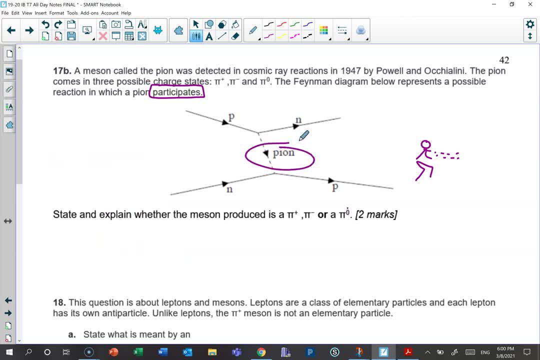 if it looks weird to you that a pion, if it's weird that a composite particle could mediate a force, that is weird. it's mediating the nuclear force, which is kind of a relic. the nuclear force really is just the residual strong force which leaks out. 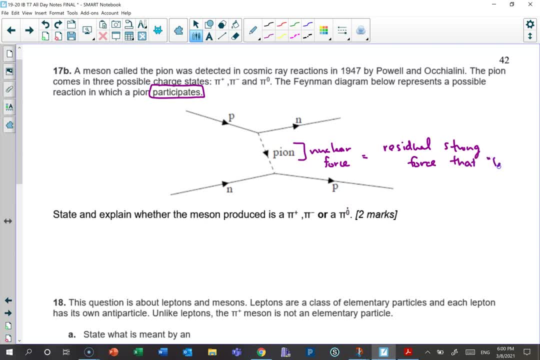 that's a technical term, not really- that leaks out of a baryon like a proton or a neutron. most of the strong force happens completely inside of the proton or completely inside of the neutron and it leaks out, allowing those two to interact with their neighbors. would this be a positive, negative or neutral meson? 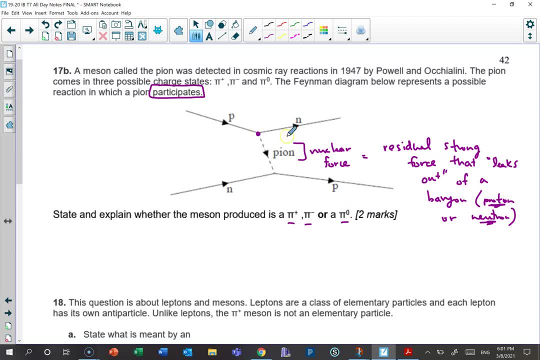 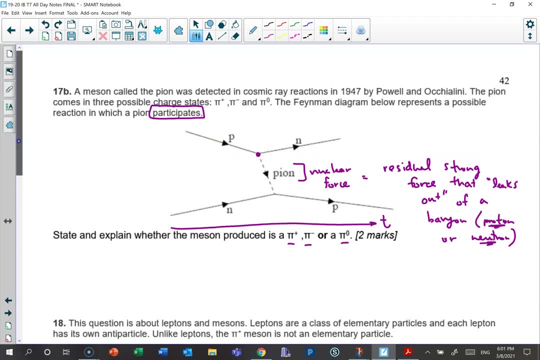 well, that's not too hard. proton, that's a matter particle. so time must be headed this way, and so you've got entering this vertex: positive one. the proton has a positive charge. the neutron has zero charge, so this must be positive one. which is it the positive pion? 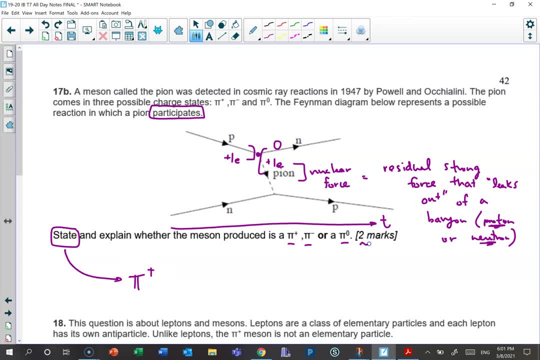 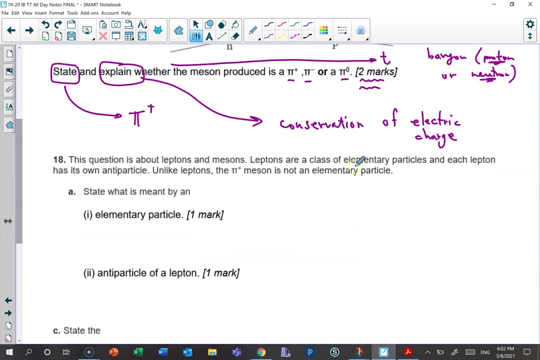 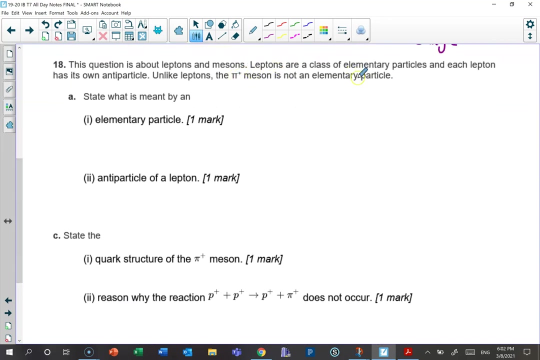 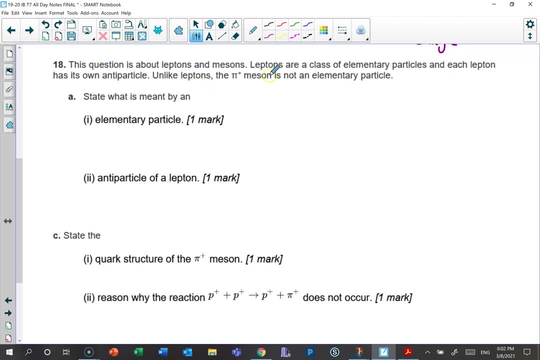 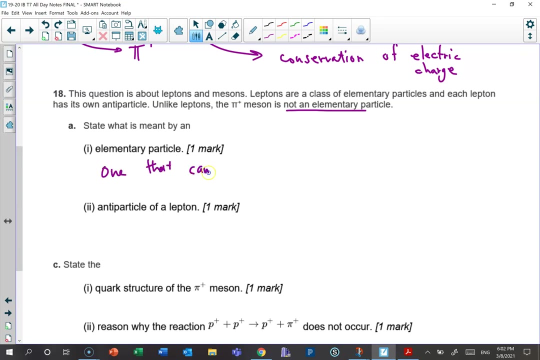 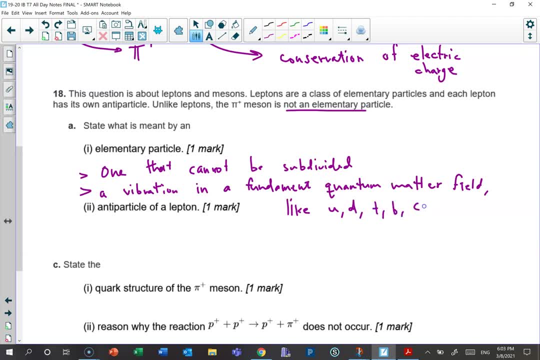 That feels a little bit excessive. I mean, you know you're not going to get it wrong if you list every single fundamental particle right. You might still get it wrong. You never know with IB. That's all of them, But I like this definition. 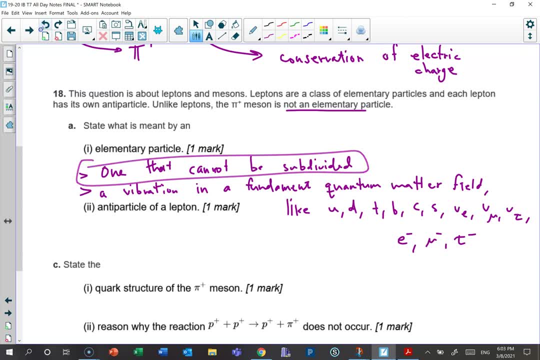 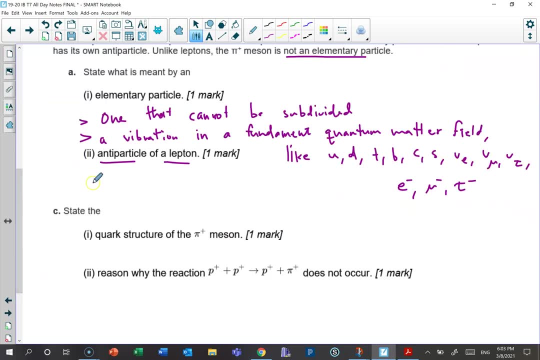 But probably they're looking for that answer. Okay, State what's meant by an antiparticle of a leptine. We talked about this already. It has all the same properties. If you want to get fancy, you can say: and comes from the same underlying quantum matter field. 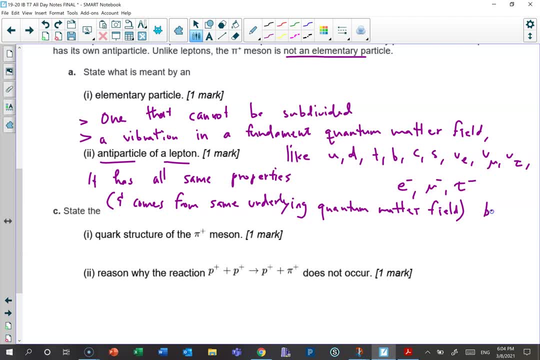 But has opposite electric charge. Okay, State the quark structure of the pi positive meson. This is something you're expected to have memorized. I've got it memorized, but if you don't, you can just write down all of the possibilities, right? 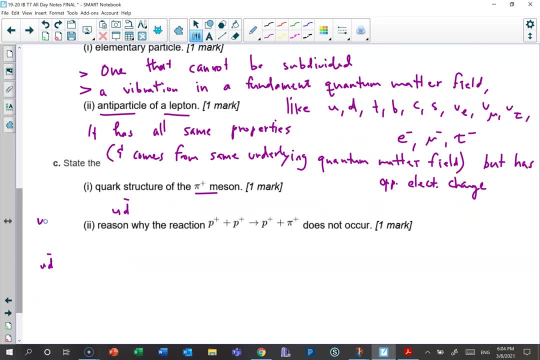 Mesons have quarks, Quarks and anti-quarks, one of each. Pi mesons use only up and down. So these are the options to figure out which is right. You figure out which of those four gives you positive total charge. 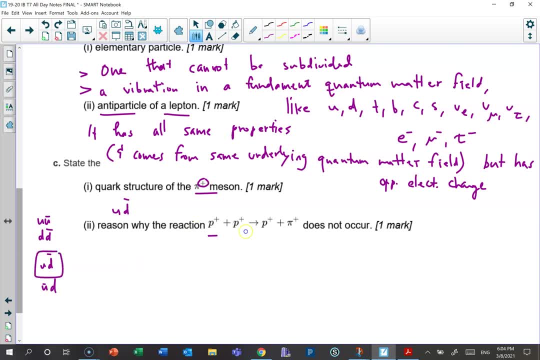 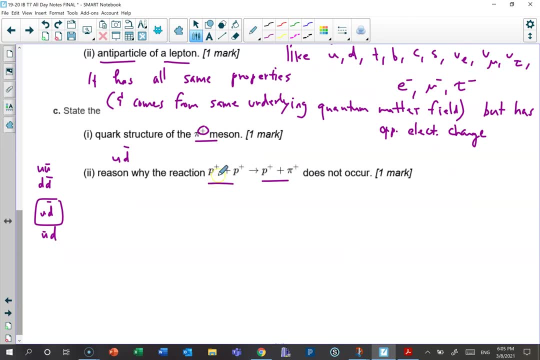 And it's that one. Okay, Why does this not occur? I've got an idea. This is a baryon, So three quarks. That's a baryon. Three quarks- This is still obviously the same baryon. 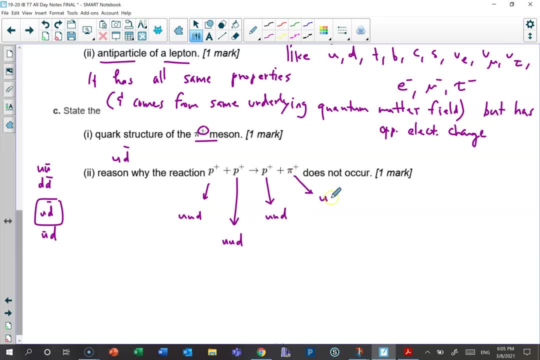 but this is a meson Like that. perhaps The total initial quark number- Do you see where I'm going? It would be six. The total final quark number would be three, Because that's positive one and that's negative one. 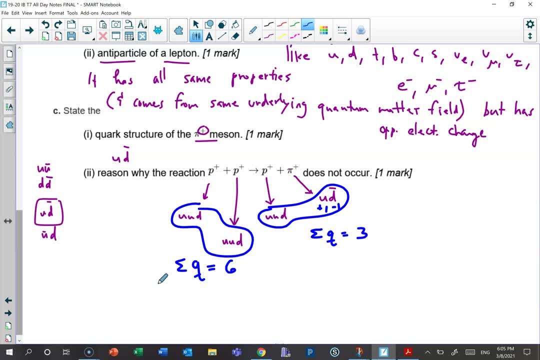 And you cannot. this is also called baryon number. Some people write it as b And they say there are two baryons on the left and just one baryon on the right. You see both, So you can do it either way. 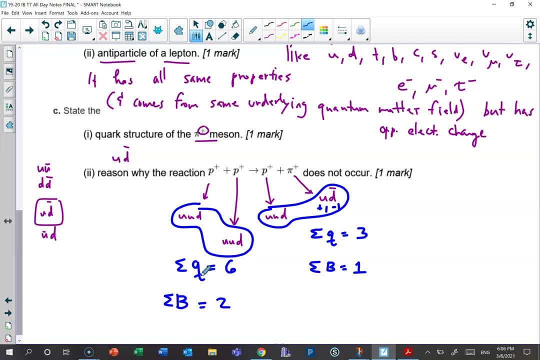 The quark number or the baryon number is not conserved, Which makes this impossible, this reaction, And we're done Great job.